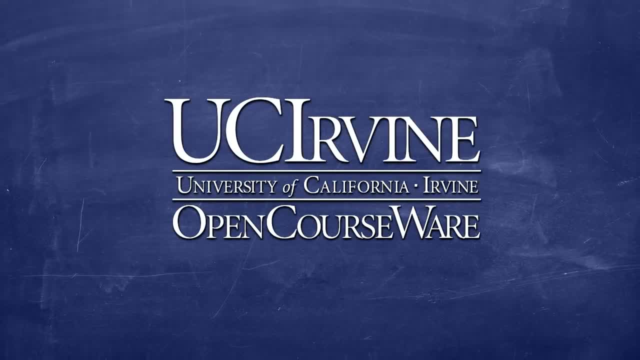 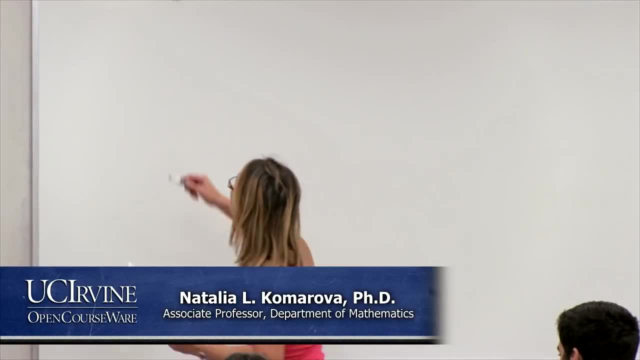 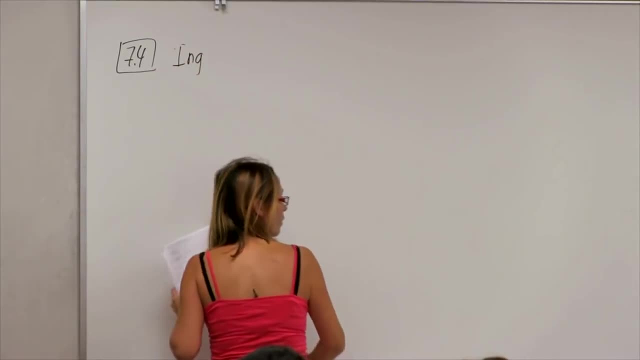 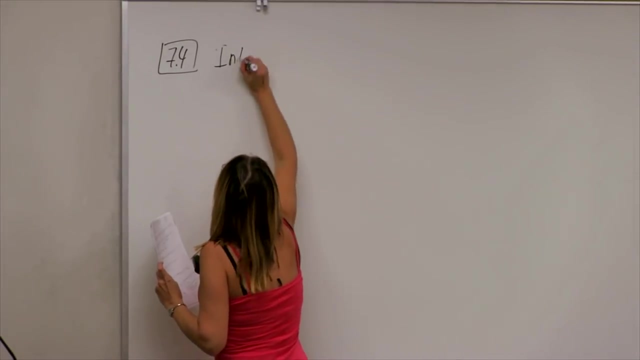 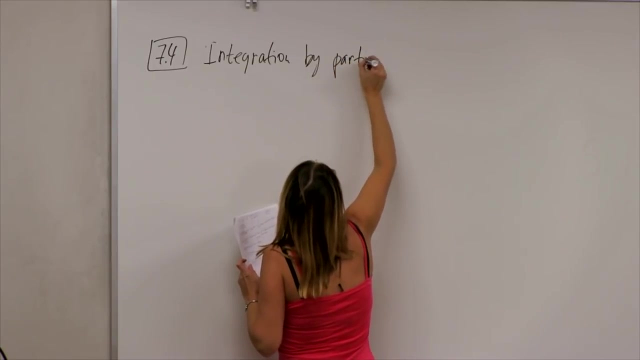 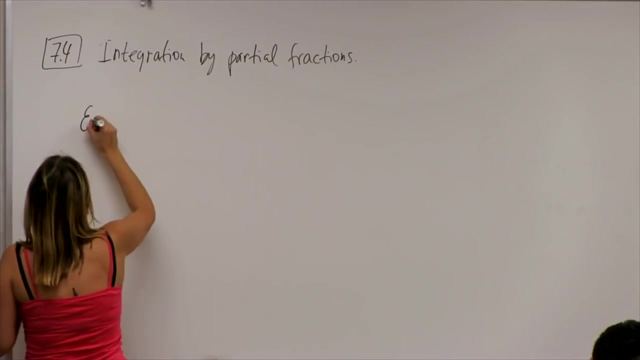 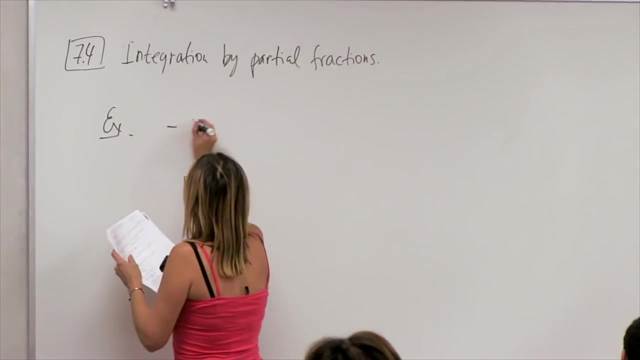 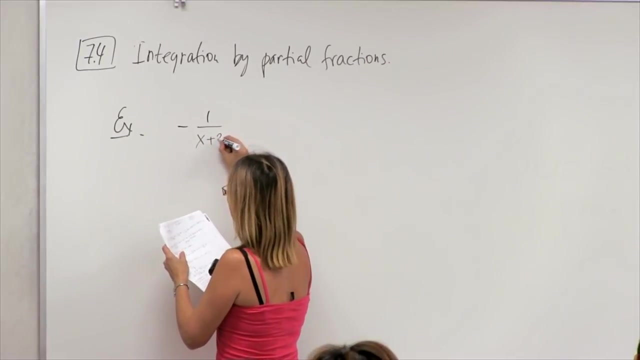 Okay so today we cover section 7.4, Integration by Partial Fractions. So to motivate, I start with an example. Okay, let's suppose that on the left we have negative 1 minus 1 over x plus 3 plus 2 x minus 4.. Okay So, 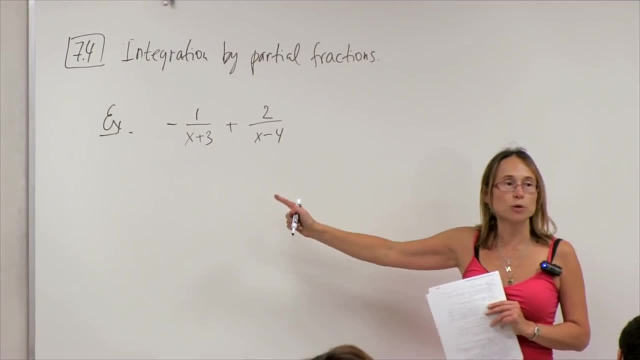 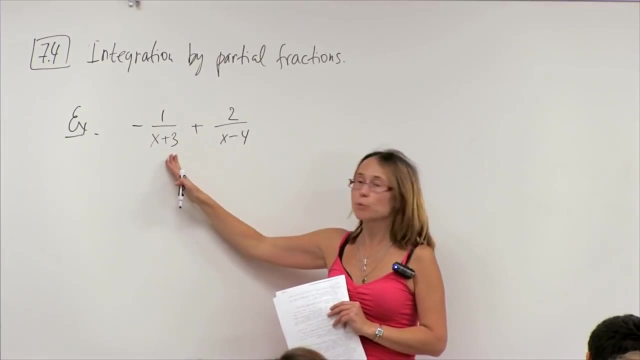 tell me, is this a function that is easy to integrate or not? If I were to integrate this, is it easy or not? So you can see that it's the sum of two terms. Let's look at the first term. What's the integral of this? Something like it's a log, right, It's a log of x plus. 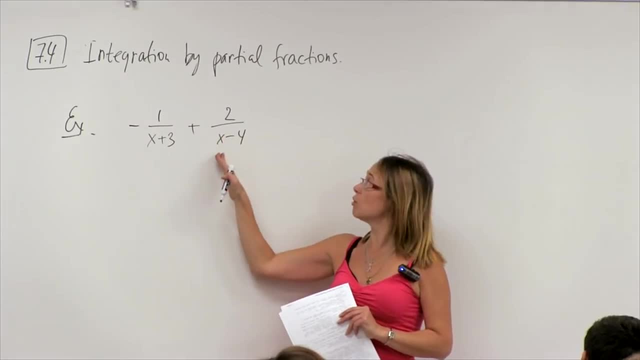 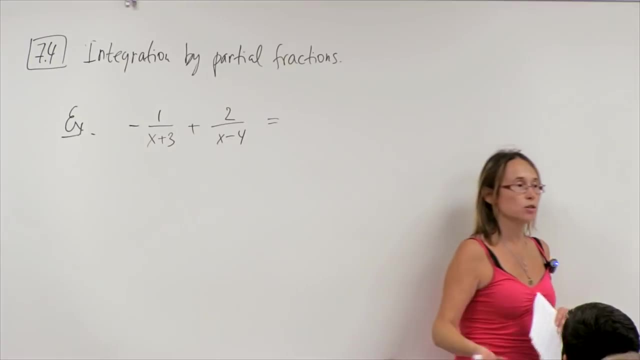 3.. What's the integral of this? It's the log 2 over log of x minus 3.. So it's very easy to integrate. Now I'm going to multiply through and get it to a common denominator, Okay. 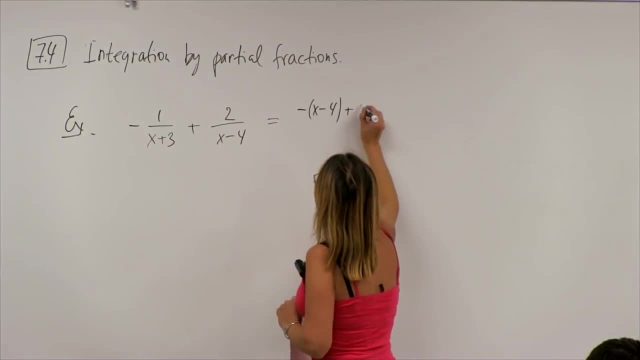 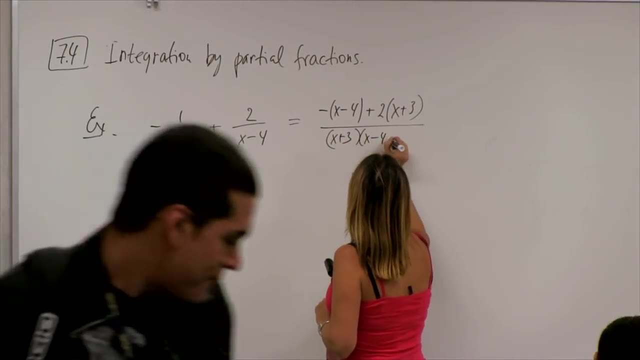 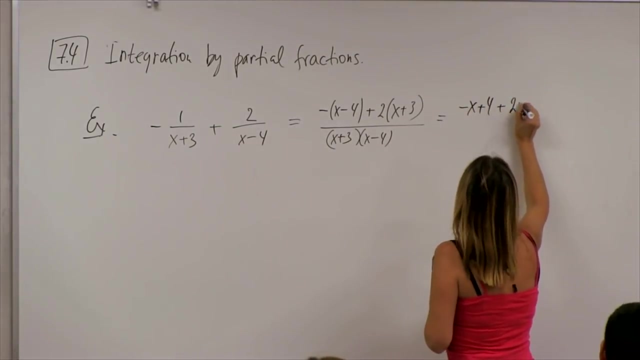 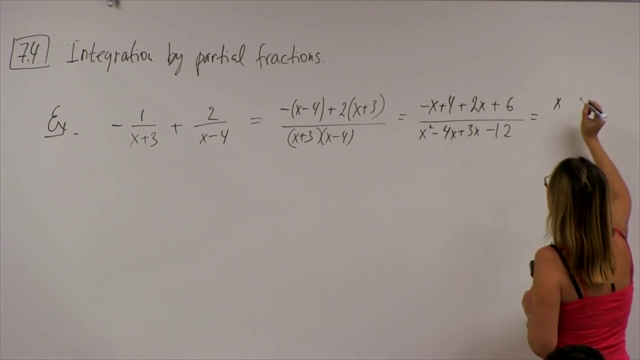 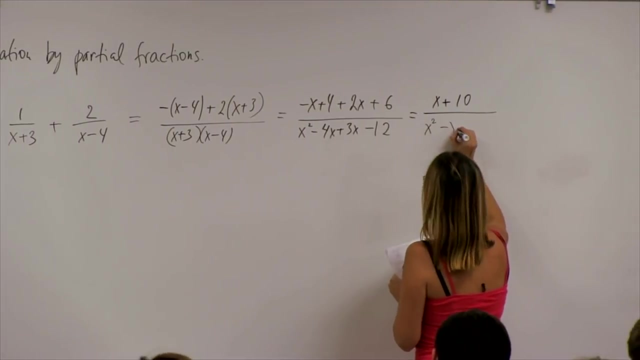 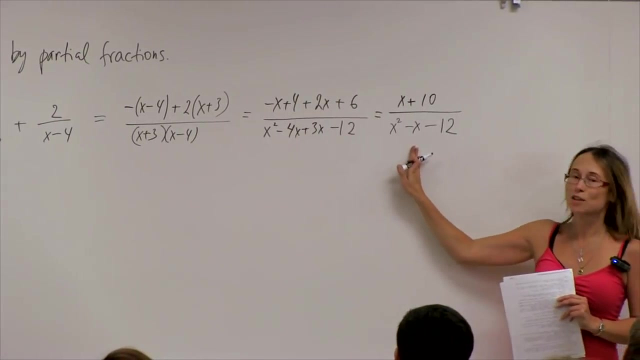 What do I get? Minus x minus 4, plus 2 x plus 3 x plus 3 x minus 4.. And I open the brackets, Okay, And I simplify Okay, Okay, so this obviously is equal to this. Now look at this function. Is this easy to? 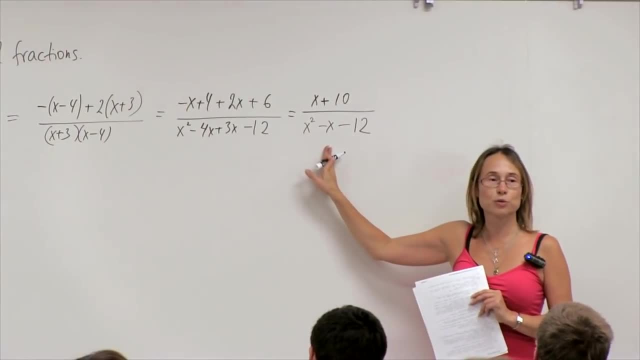 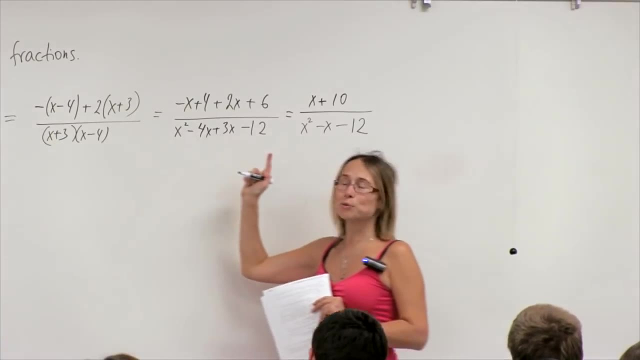 integrate. Would you know immediately how to integrate this? No right, You would have to stop and think: What do I do next? So on the left, we have something that is very easy to integrate. On the right, we have something that we don't know how to integrate, and they're. 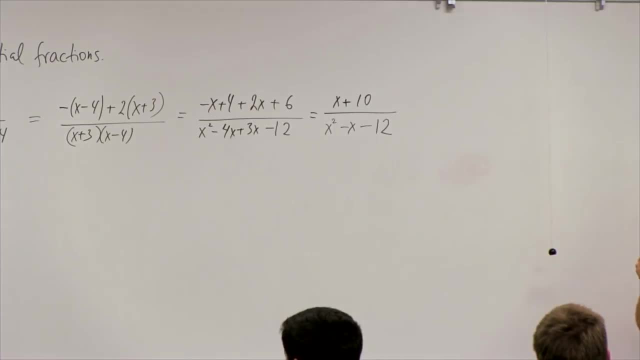 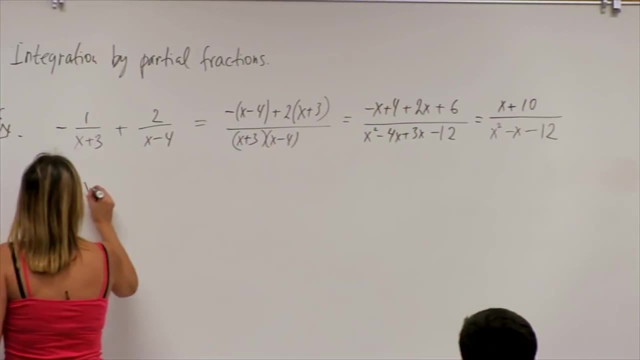 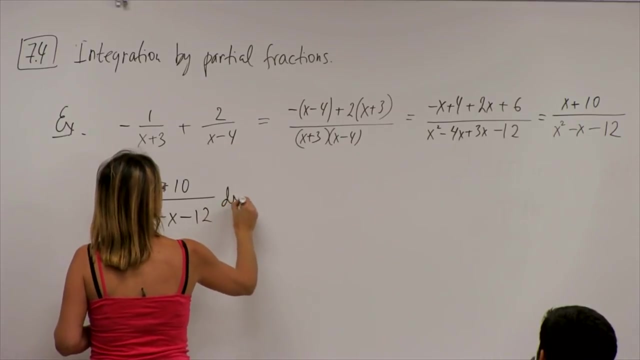 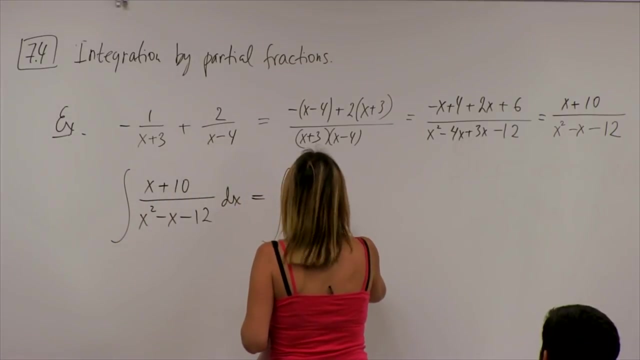 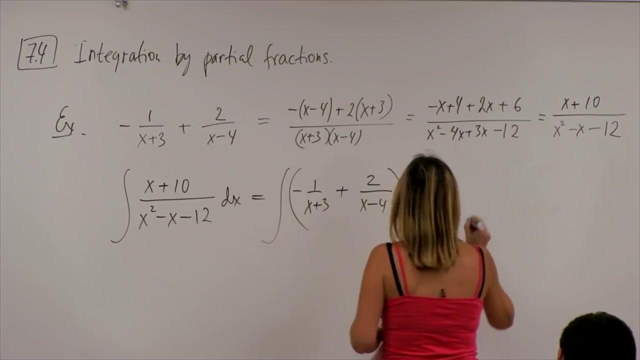 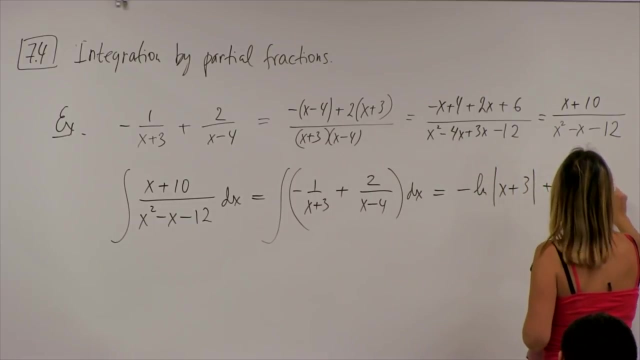 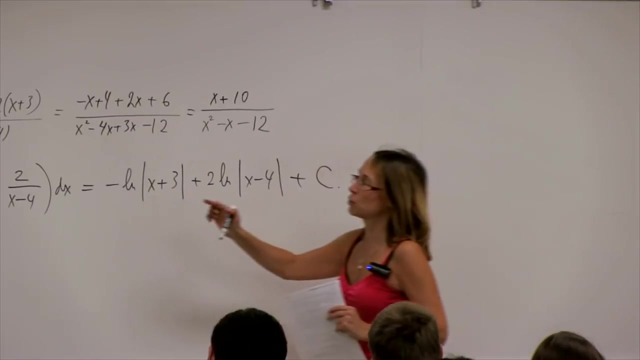 and they're the same. okay, so that, working backward, that gives me a very good method to integrate something like this. so let's write it down right away: the integral of the right hand side is equal to the integral of the left hand side, which is very easy, and I'm done right. only if I knew to begin with how. 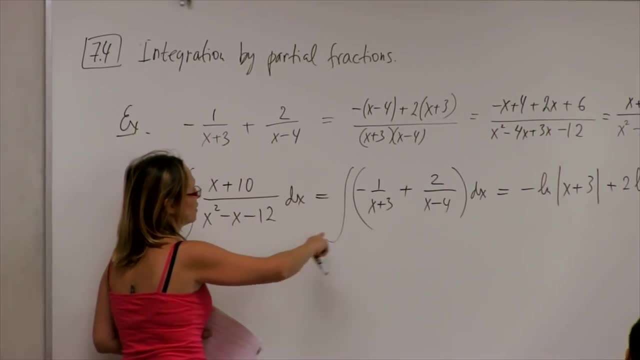 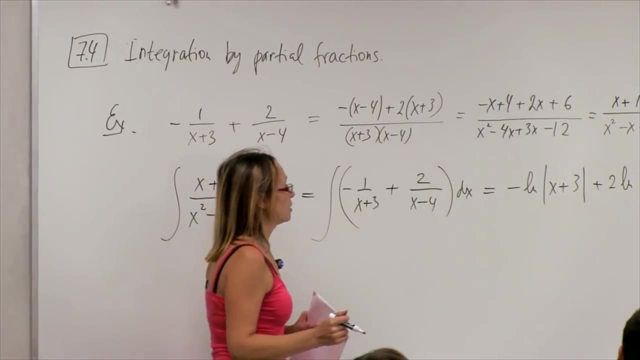 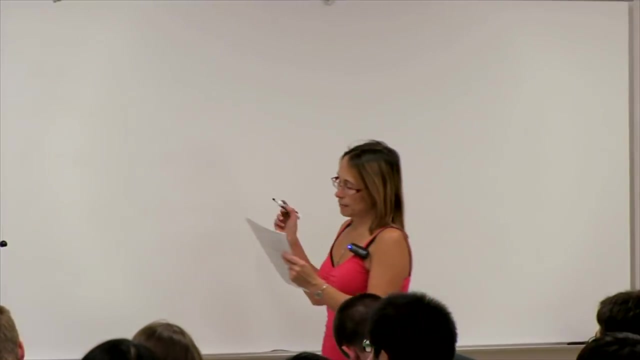 to represent this fraction as something like this: okay, so let's stay on the left hand side. okay so let's see. did I hear that like this? I would be able to integrate all such examples, and this is where we have the method of partial fractions that we are going to cover today. so we 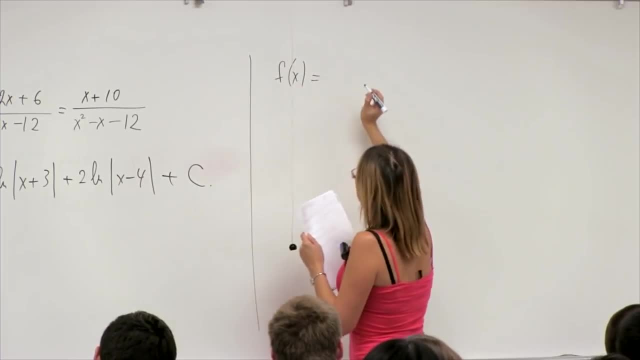 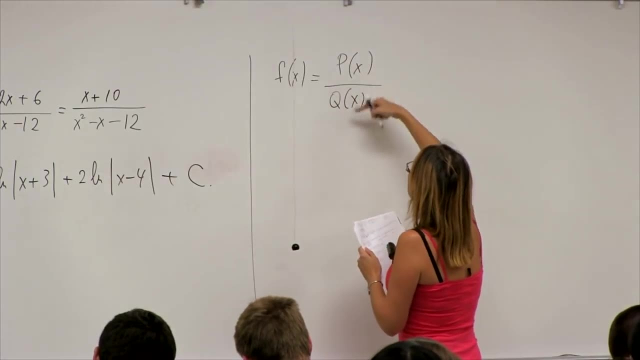 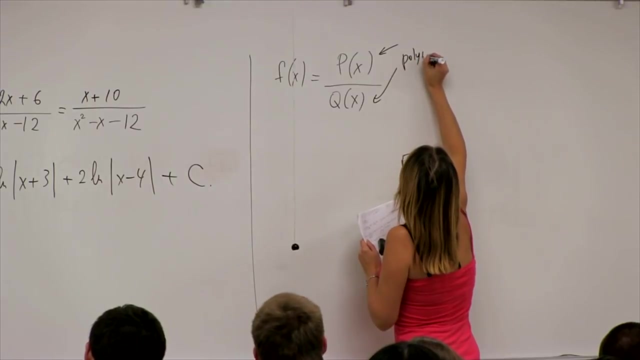 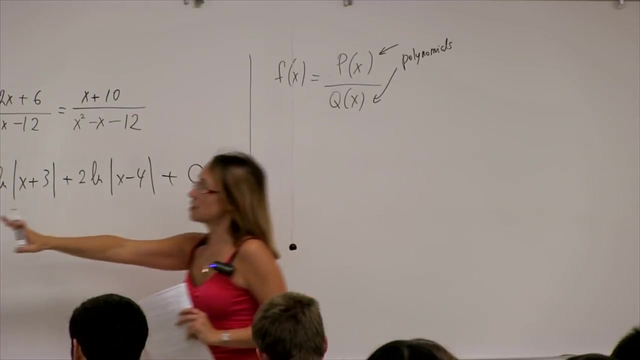 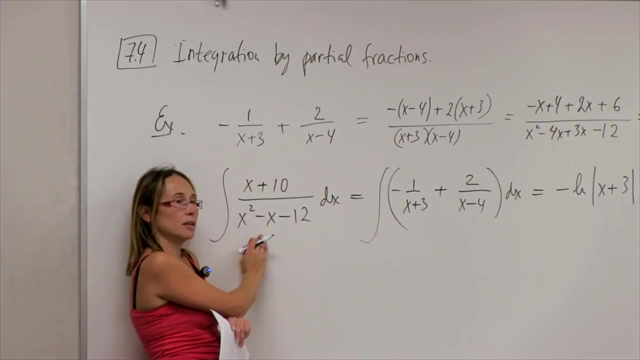 will consider functions that look like this: P of X over Q of X. P and Q are polynomials- okay, polynomials, and, as you can see, this is an example of such a function. we have a polynomial of the first degree on top and the polynomial of the second degree at the bottom, so we're going to need the notion of a. 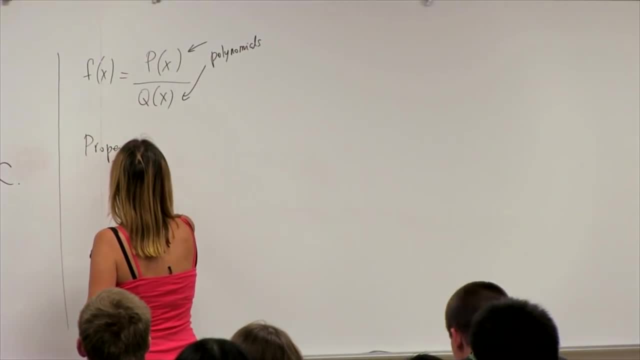 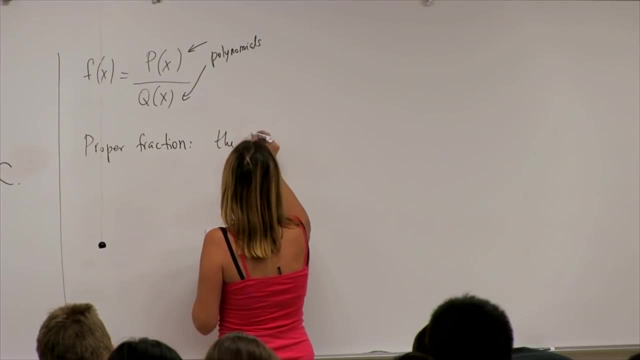 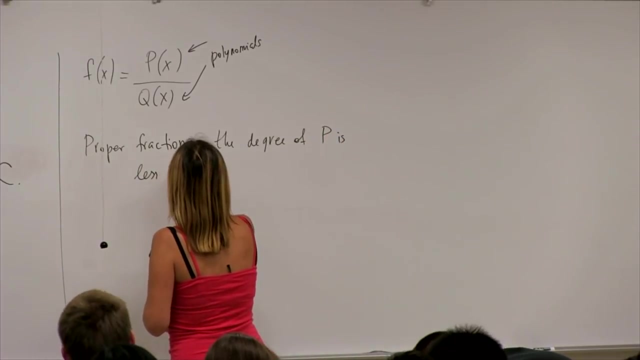 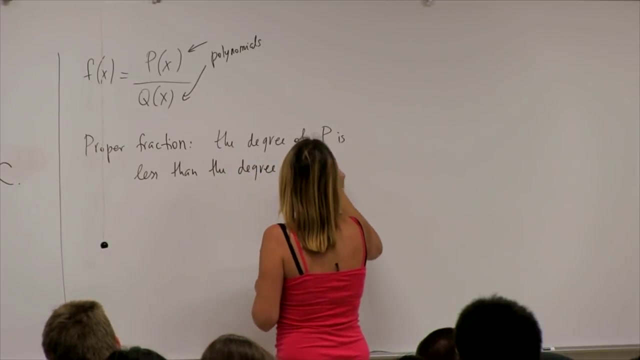 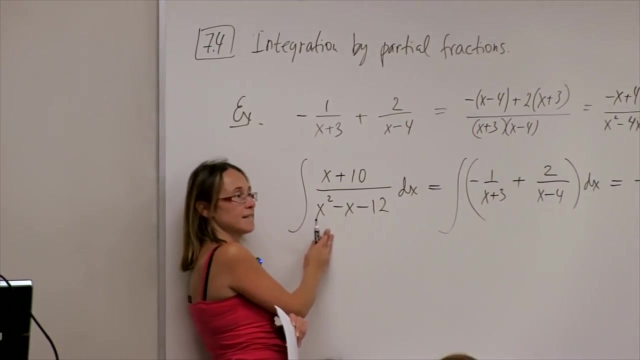 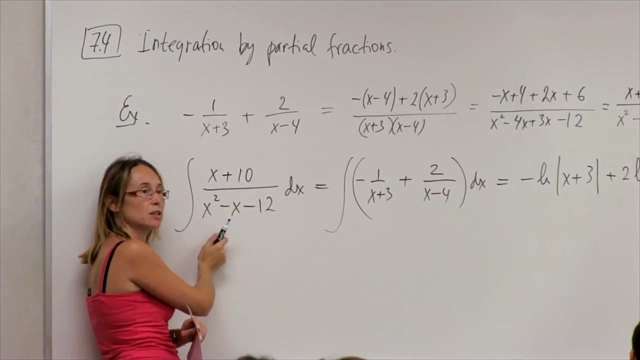 proper fraction means that the degree of P is less than the degree of Q. okay, so is this a proper fraction? is this a proper fraction? the degree of a, a, a, P is 1. the degree of Q is 2, so it is a proper fraction. now, if we are given an 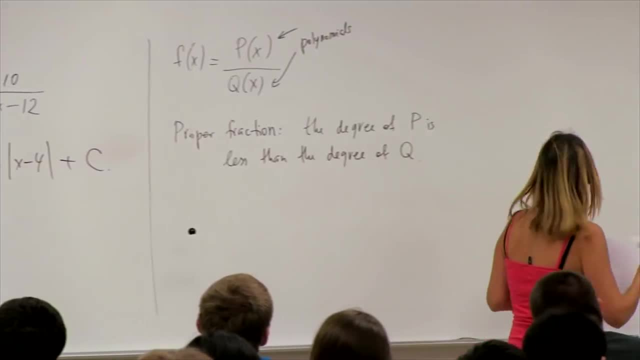 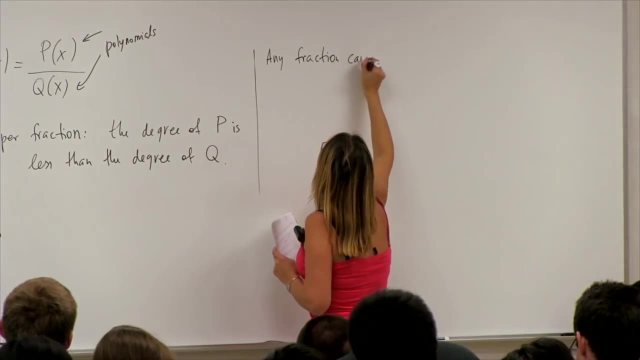 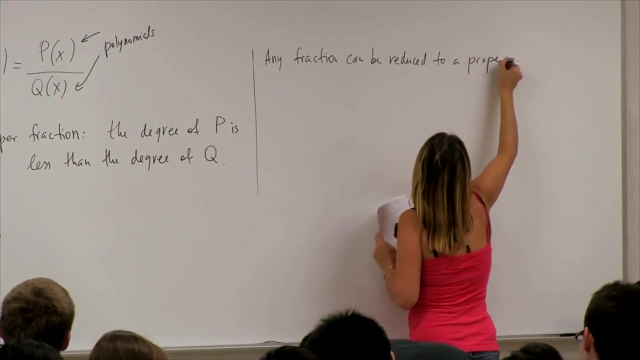 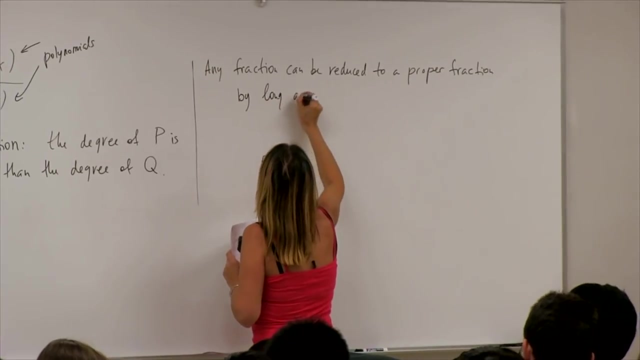 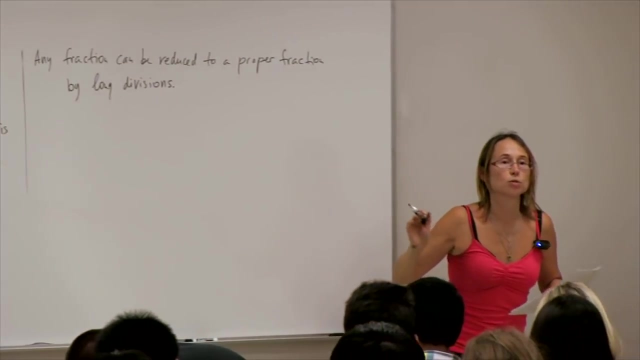 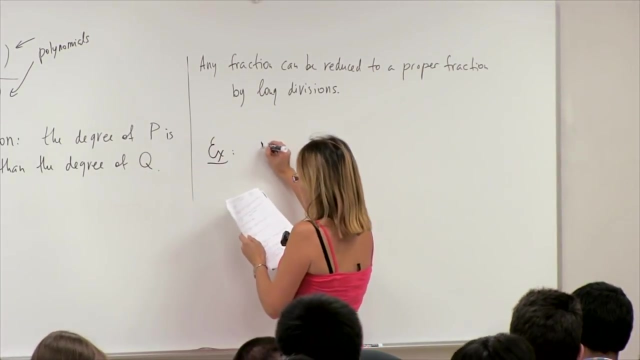 improper fraction, we can always reduce it to a proper fraction. any fraction can be reduced to the proper fraction by long, by long divisions. so this is something that you should be able to do: to divide one polynomial by another. so for conceptal, let's consider X cubed, last to. 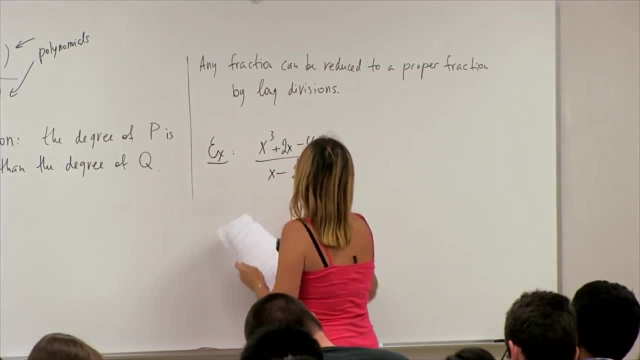 X till minus form, X minus 2. so you can't hear. this is not a proper, because here the degree of P is three剑3ég وهmetph говорит: в soror komunя вungen. full square is 3. 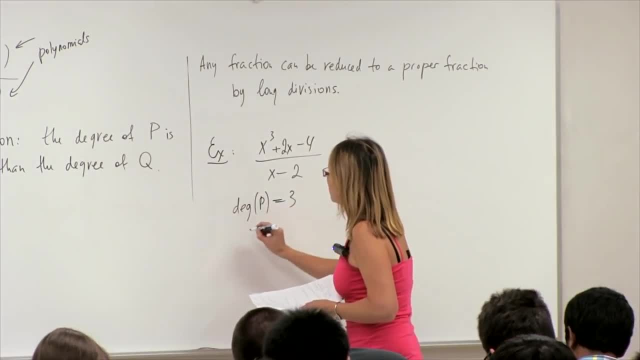 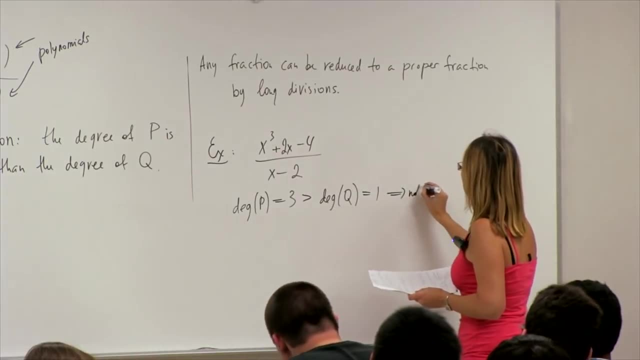 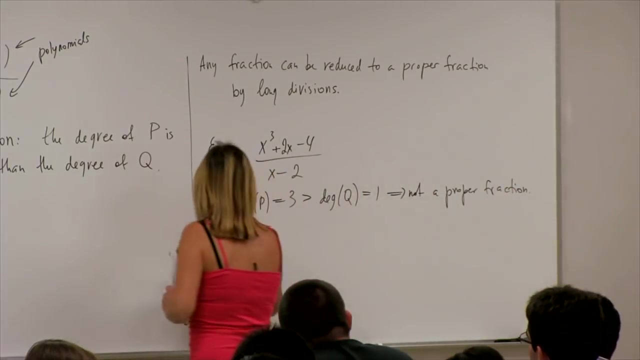 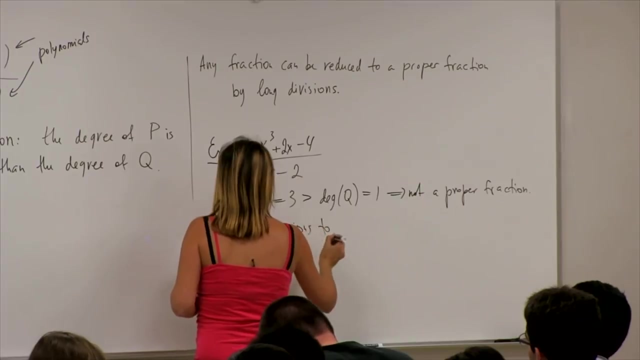 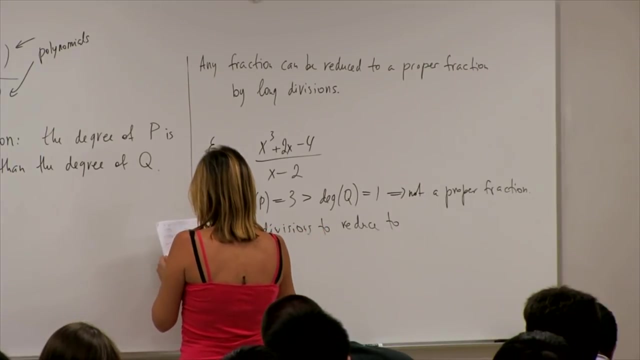 so you can see this is not a proper fraction, because here the degree of P is 3, 3 and it's greater than the degree of Q, which is 1, not a proper fraction. so we can use long divisions to reduce to x squared plus. 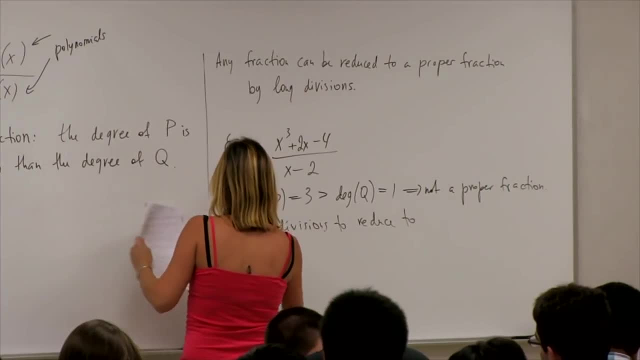 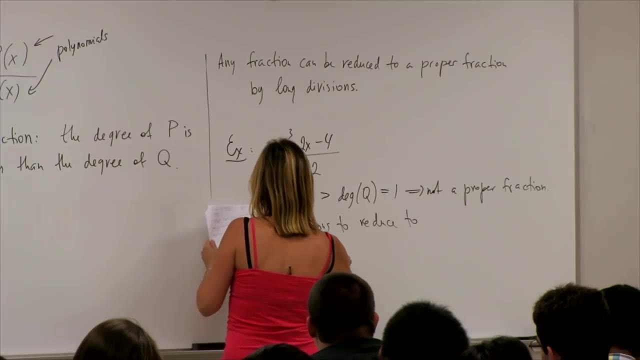 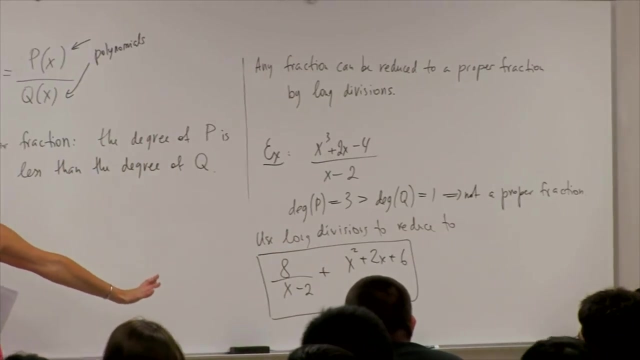 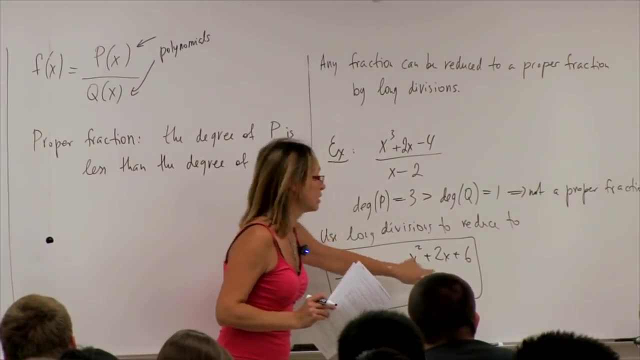 8 plus over x minus 2 plus x squared plus 2x plus 6. so you'll be practicing to do this at the discussions, okay, and you can see that there is something. there's a polynomial which is very easy to integrate, plus a proper fraction, which is also easy to integrate. 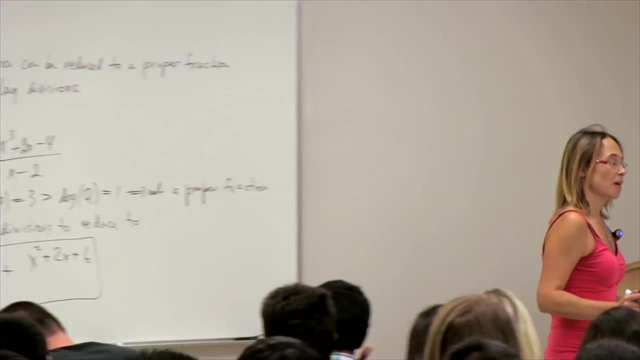 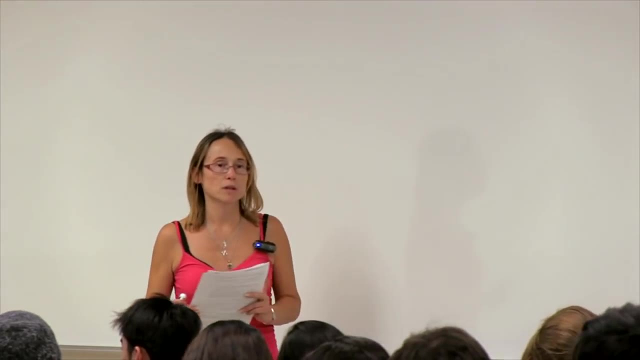 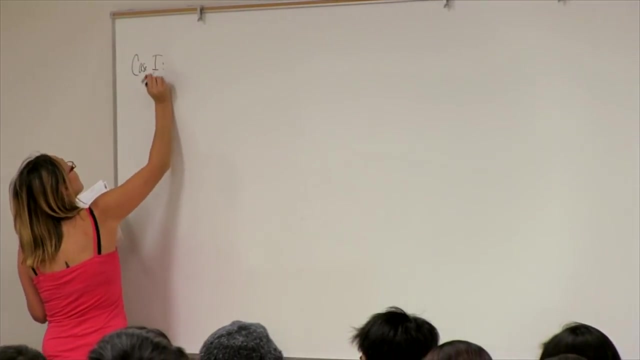 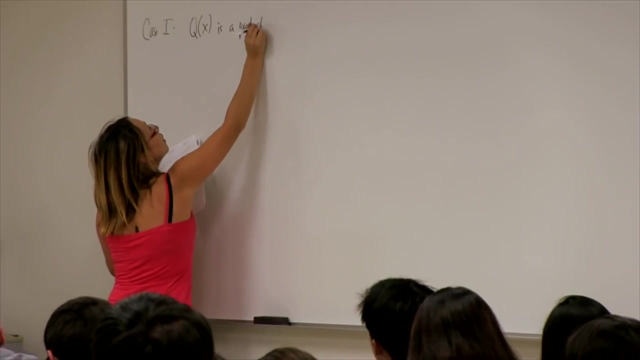 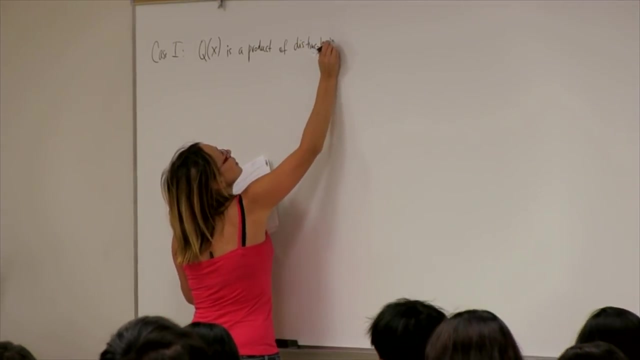 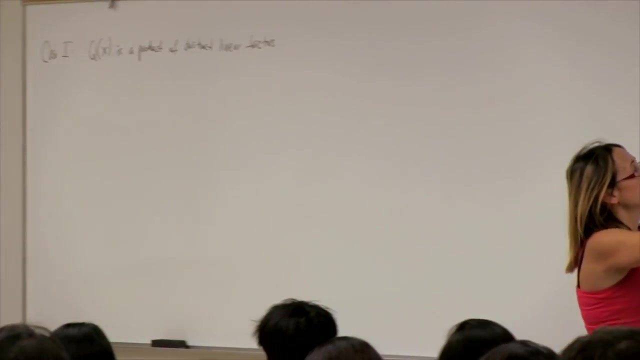 and the methodology will be worked out at discussions. so now today we'll go through four cases of partial fractions, and they go from easy to hard. so case one is when Q of x is a product of distinct linear factors. so let me keep track of them here. 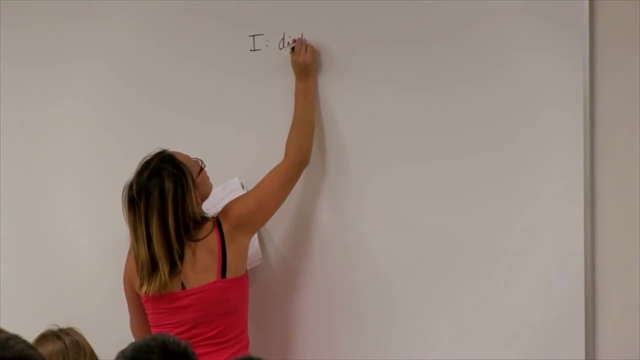 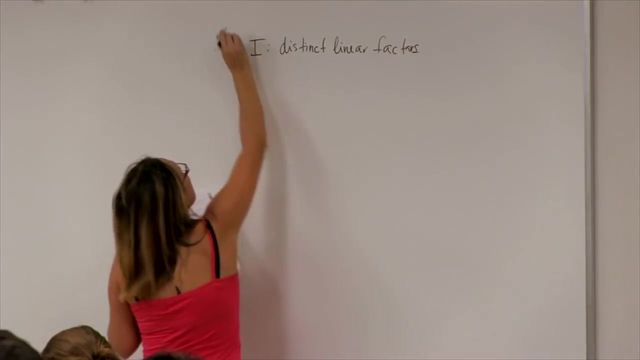 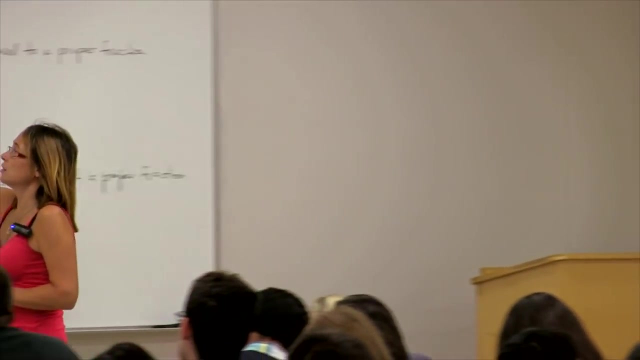 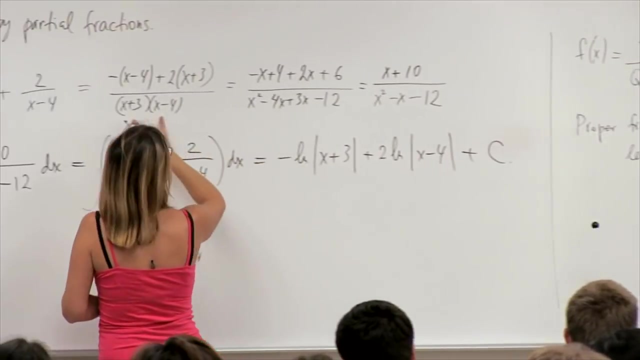 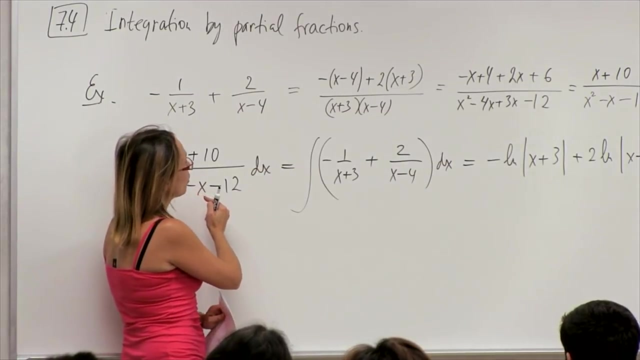 one is distinct linear factors. so an example. so to classify all these things, we always look at the denominator of a proper fraction and we'll try to factor it into linear multipliers. so, for instance, here we have a degree two, polynomial, and somehow we were able to factor it. 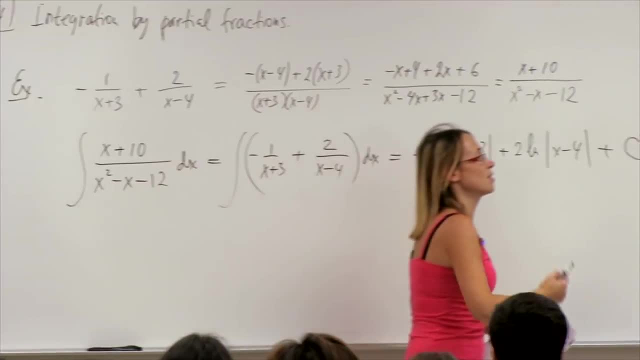 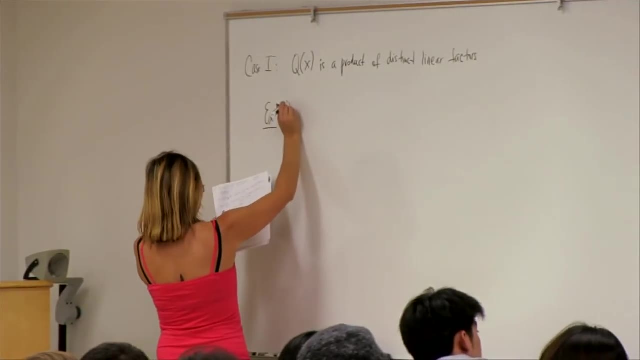 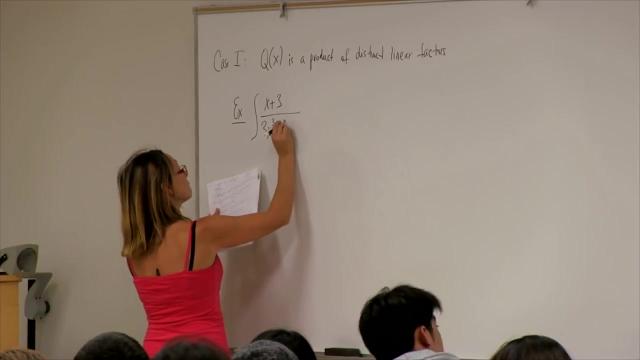 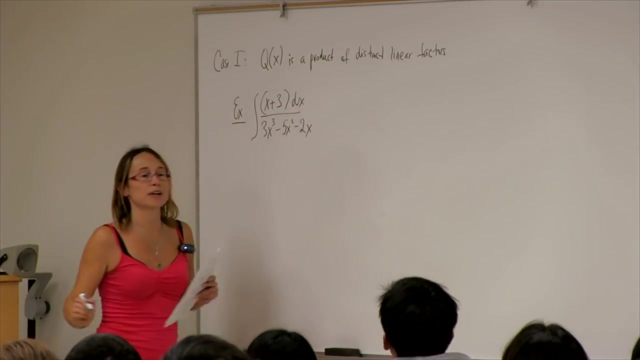 into these two, and so this comprises the main idea of the method. so let's look at an example to make this all very clear. so let's suppose we are given the following fraction: is this proper or incorrect? so the degree of p is one, the degree of q is three. 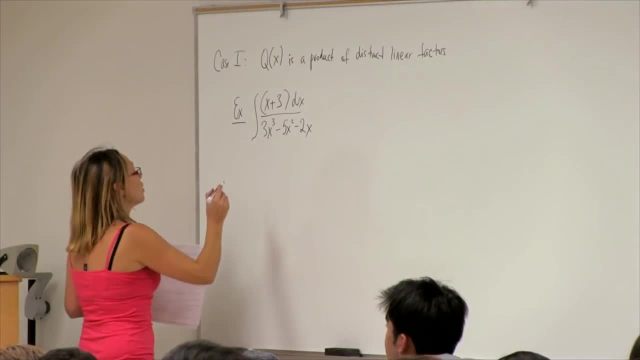 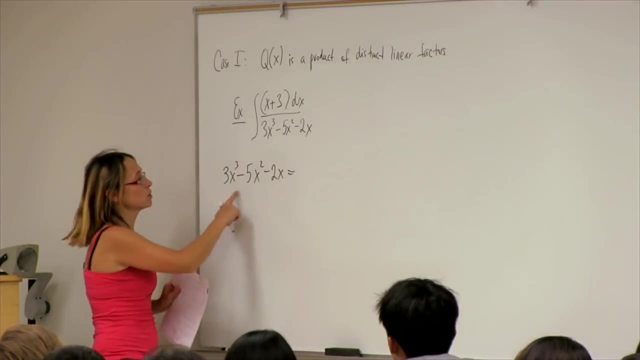 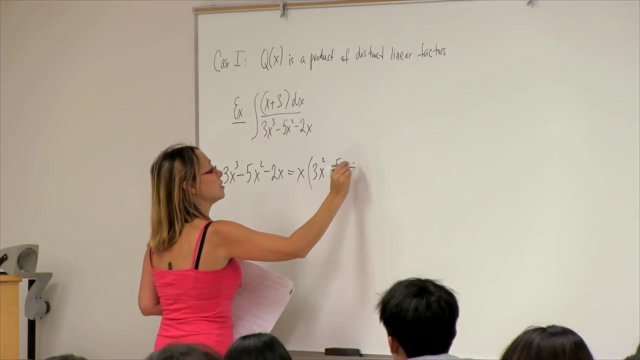 so it's a proper fraction, so we don't have to do anything. now let's consider the denominator and try to factor it out so you can see that x multiplies everything. so I put x here and I have three x squared minus five x minus two. 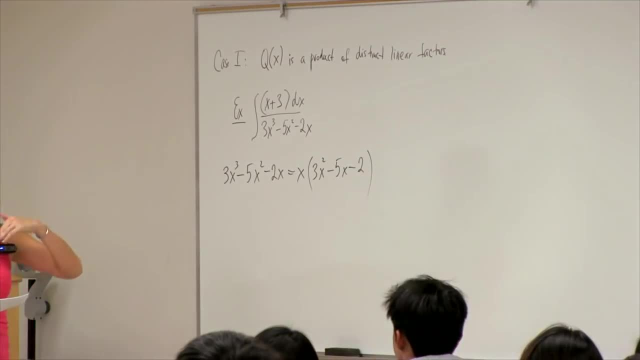 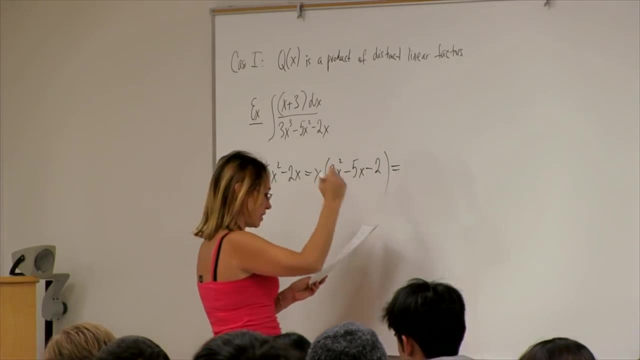 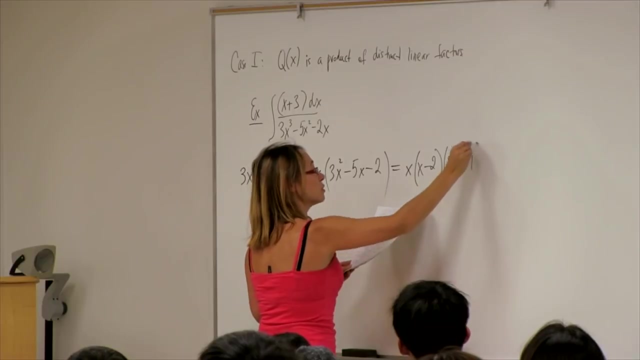 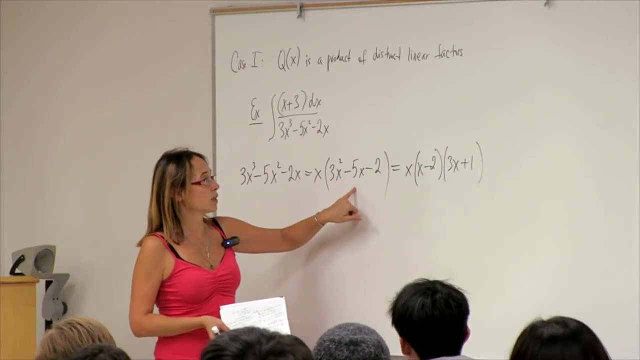 now it's a quadratic polynomial and everybody knows how to you know decompose this into factors. we just have to find the roots. so I'll skip one step here and write down the decomposition of this quadratic polynomial. if I find the roots of this, I'll get one third. 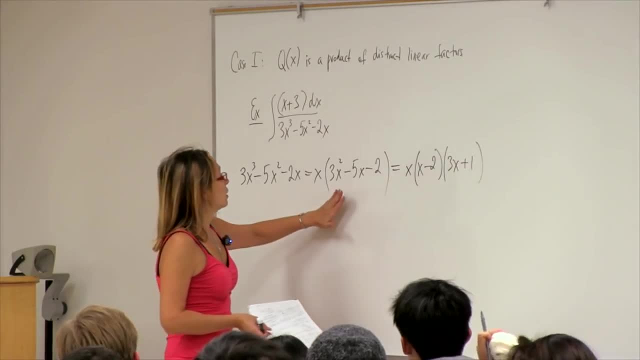 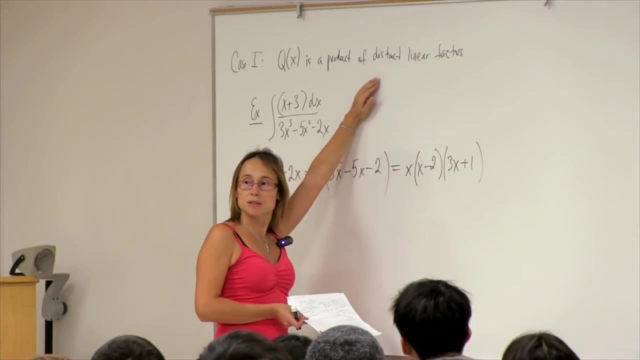 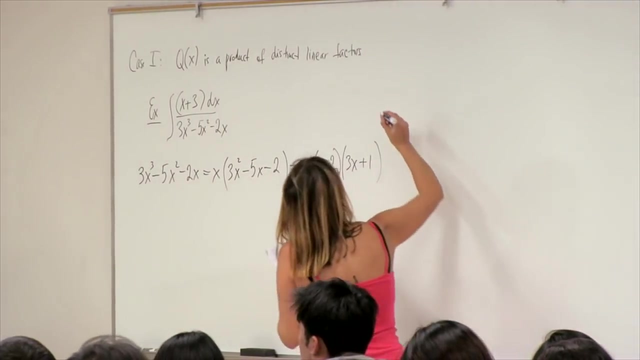 minus one third and two. so you can see that this is a product of three distinct linear factors, and that's what classifies it as the simplest of cases, and we'll have other cases a little bit later. so the next step is to write it in the following way: 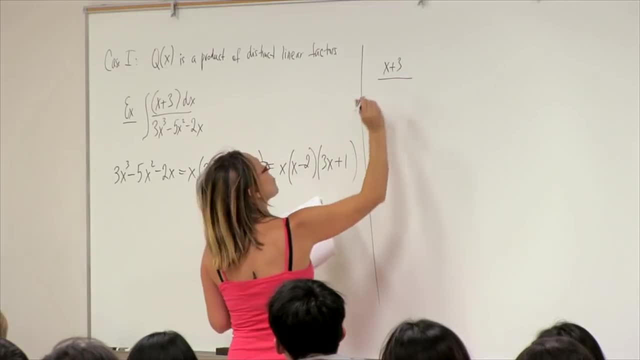 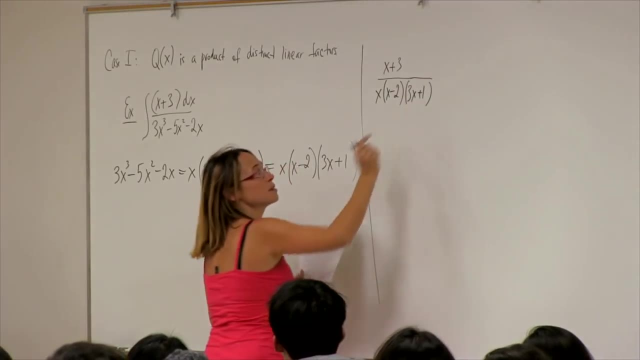 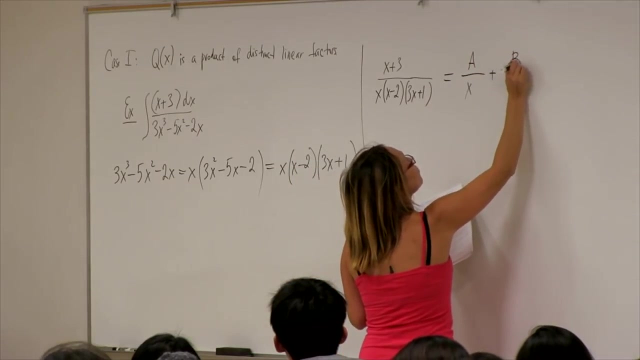 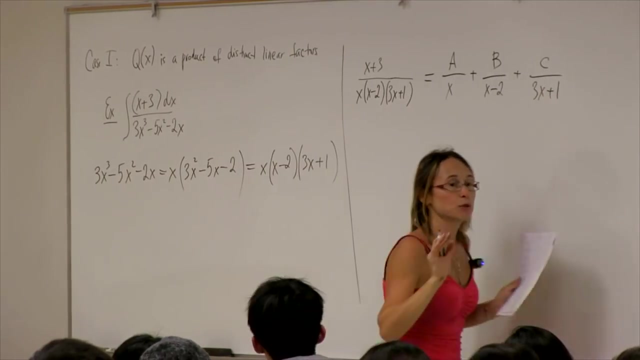 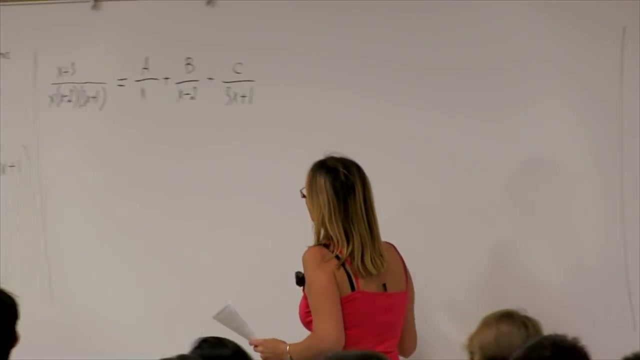 so our given function. now I'm always going to write it like this: to make explicit the three linear factors, I represent it as the following decomposition: and it can be shown that you can always find constants a, b and c to make this an identity. so our task is exactly this. 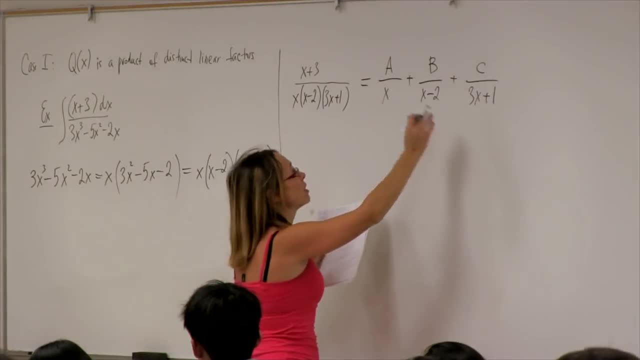 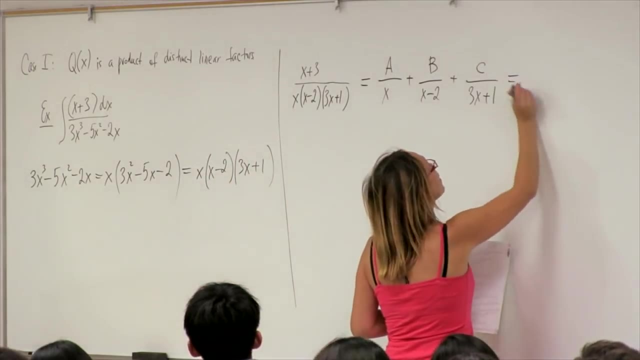 to find a, b and c. the next step is obvious. this has to be equal to this. the right has to be equal to the left. so I bring the right hand side to a common denominator. so in the denominator I'm going to have the product of the three factors. 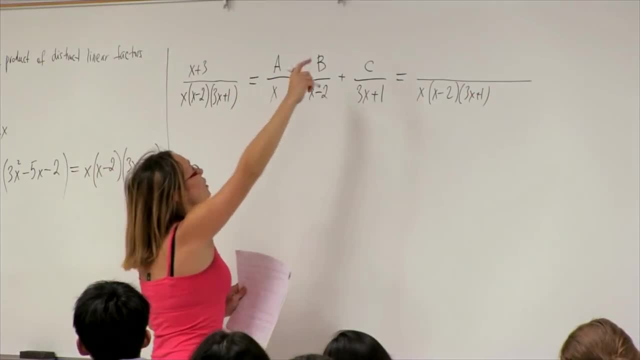 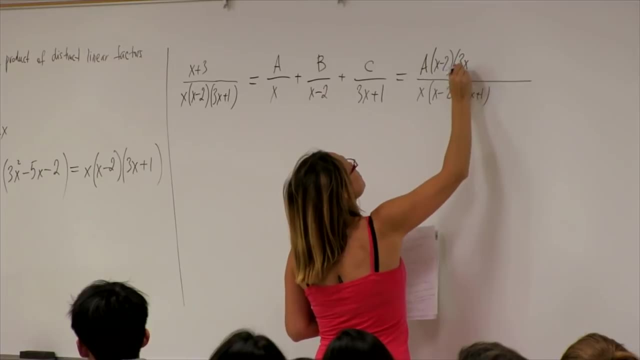 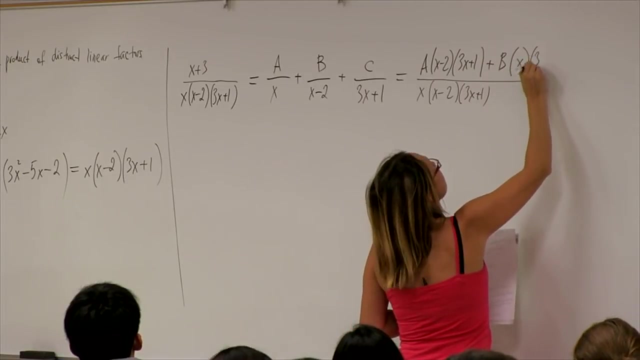 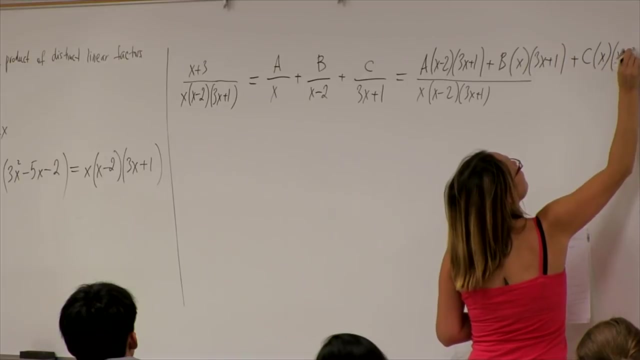 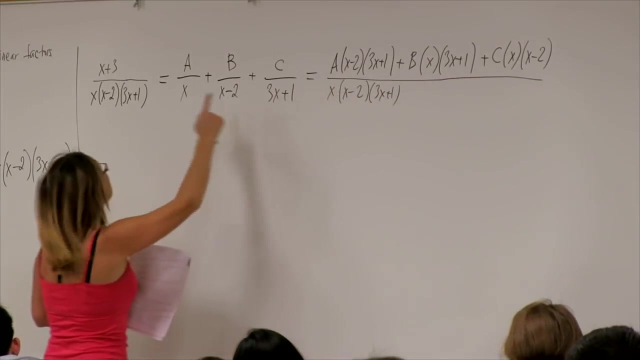 just like on the left and in the numerator I'm going to have the following combinations of coefficients. so I have to find numbers a, b and c to make the right hand side equal to the left hand side. the denominator is already the same by construction. 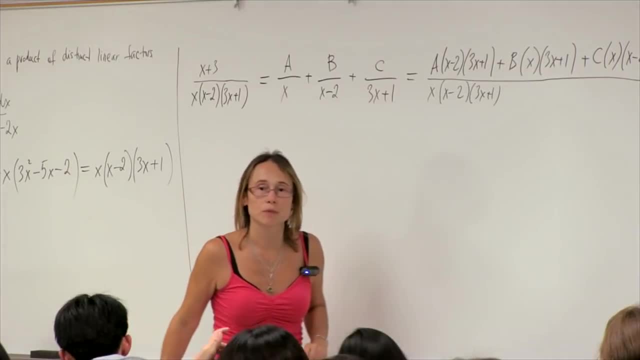 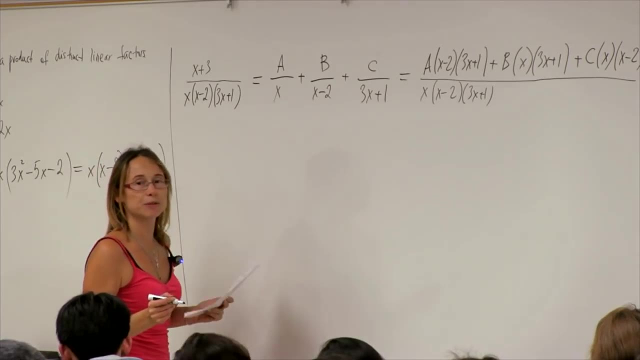 they're going to be the same: linear factors in the denominator. the numerator is the problem, alright, so how do we make them the same? there are two methods of doing it, so I'll start with the simpler method. so the simpler method doesn't always work. the more complex method always works. 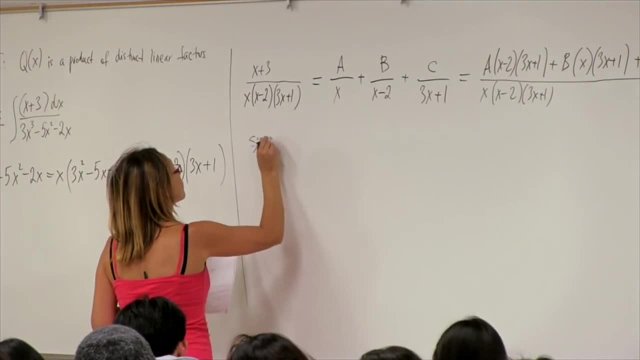 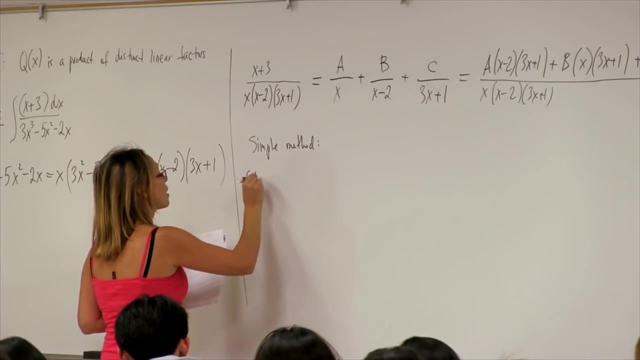 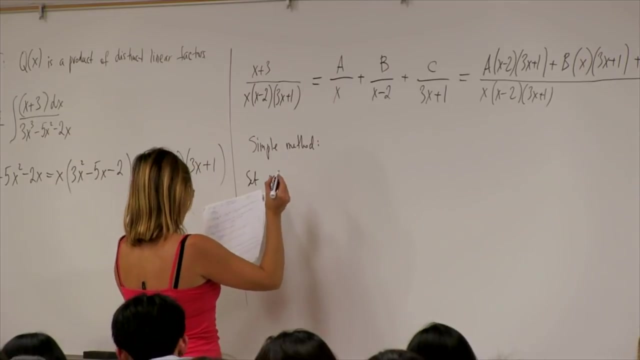 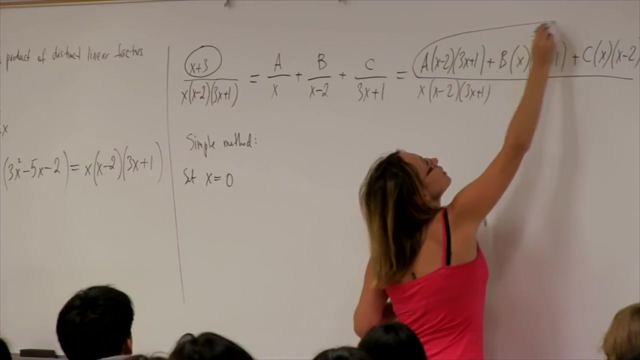 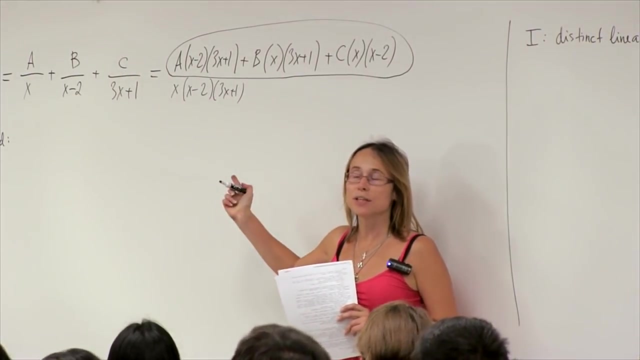 but it's a little bit more involved. so simple method. I'm going to set x equals 2, for instance, x equals 0, so this numerator has to be equal to this numerator for all values of x. the two functions have to be the same, so the equality has to hold. 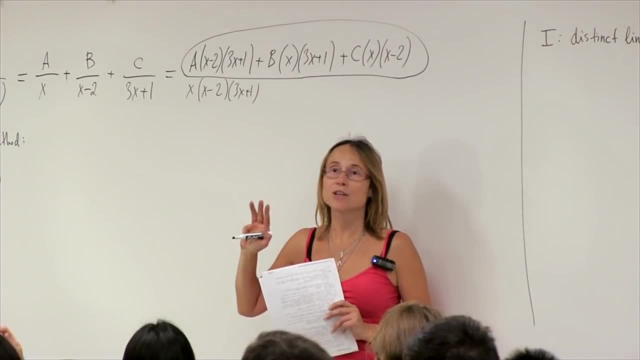 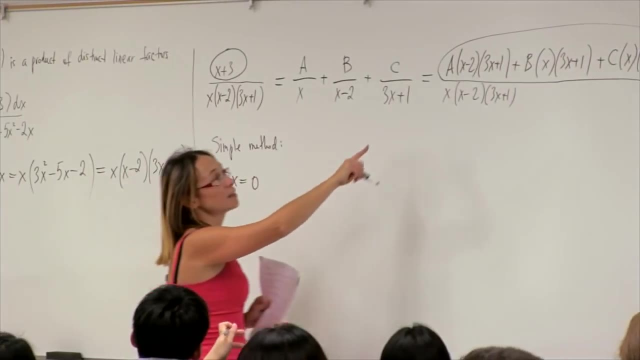 for all values of x. I'm going to pick three values of x that make this equation really easy. so the first value is: x equals 0. and why is it easy? see the first factor, let's not talk about it for now. this one is 0. 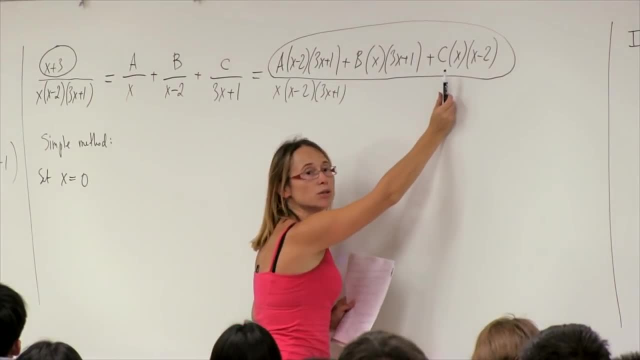 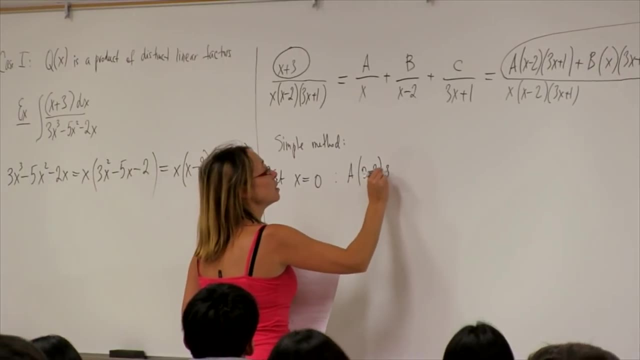 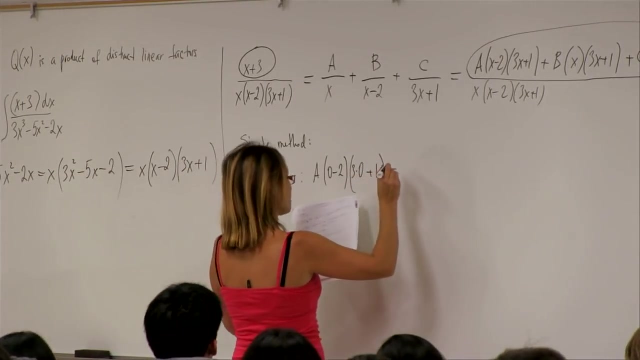 because x equals 0 and this is 0. so on the right I just have a 0 minus 2, 3 times 0 plus 1, or I can say that this is minus 2x minus 2a and that's supposed to be equal to the left hand side. 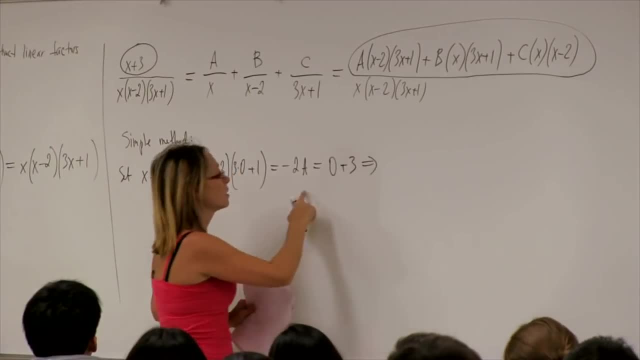 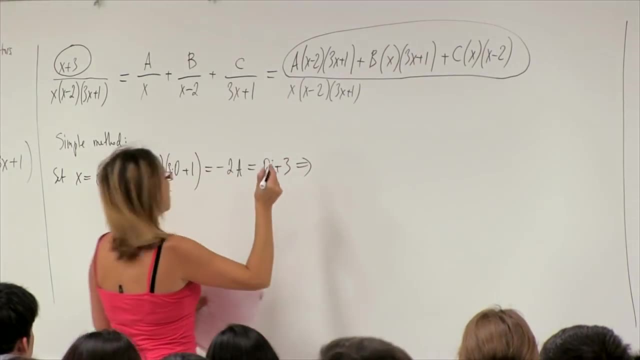 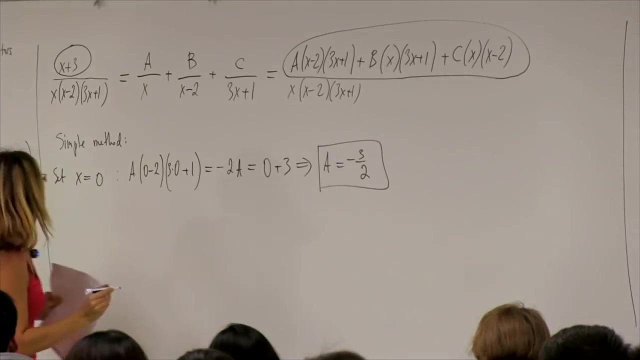 which is 0 plus 3. so this is a very easy equation for a, because many things cancel. these two whole terms cancel. so that gives me a equals minus 3 halves. then what are other good choices of x to take to make this really simple? 2: 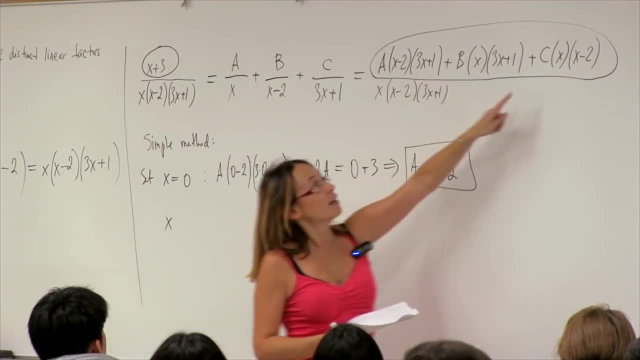 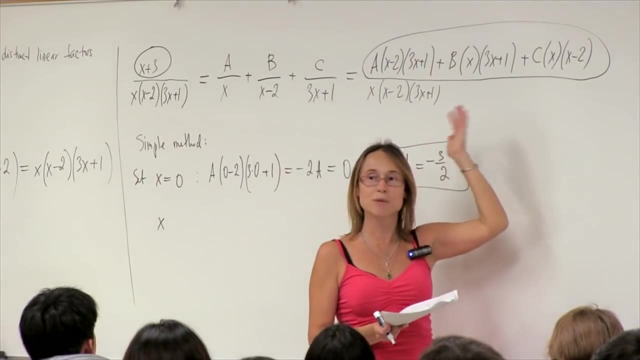 because if x equals 2, this one is killed, and this one is killed. the only remaining factor is this one. it's 0. we choose x in such a way as to kill as many of these as possible. so x equals 2, so I have 0. 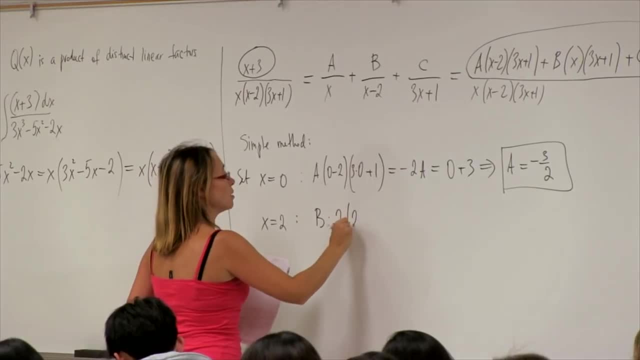 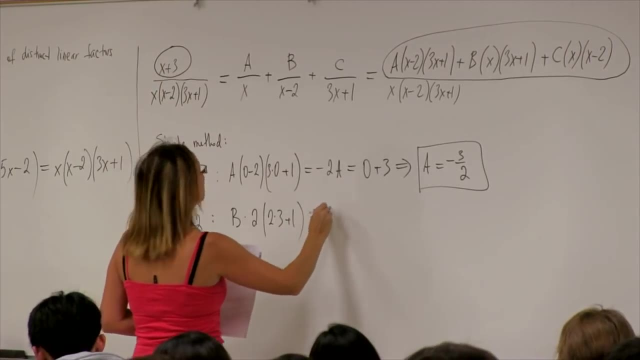 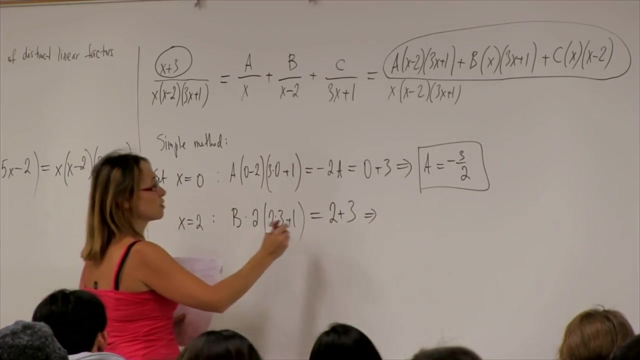 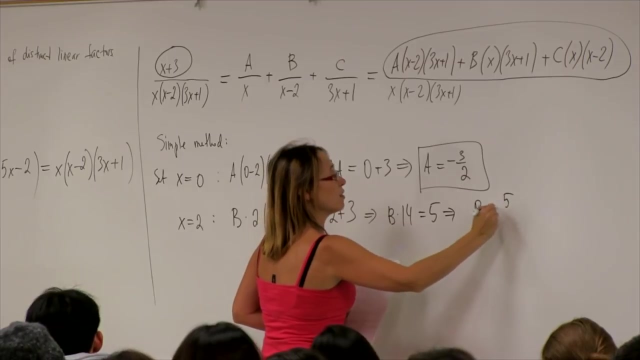 plus b times 2 times 2 times 3 plus 1 plus 0 equals- left hand side is 2 plus 3. so let's rewrite this equation. this is b times 14 is equal to 5. therefore, b is 5 over 14. 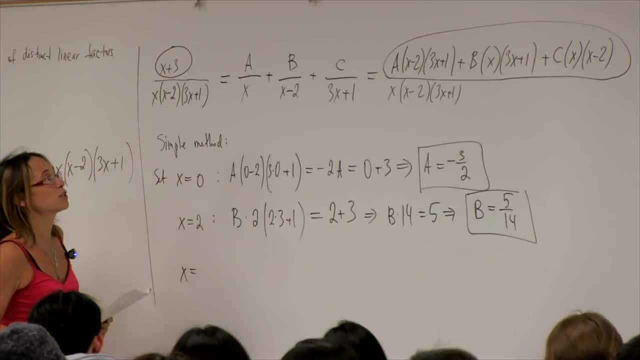 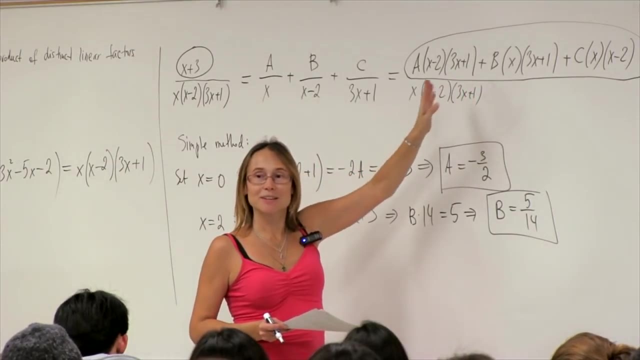 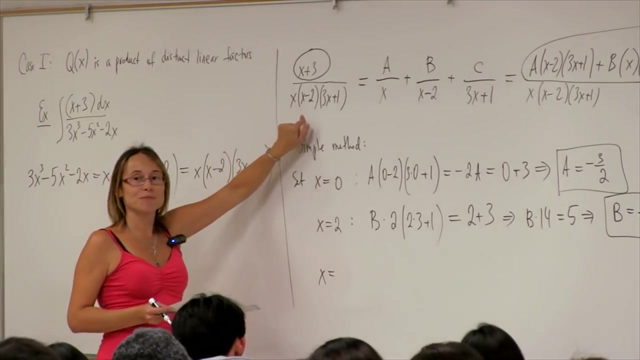 so I solved for b. the last one was the last good choice for x minus 1. third. by the way, you can always determine these easy values by looking at the roots of the original denominator. what are the roots here? 0, 2 and minus 1. third. 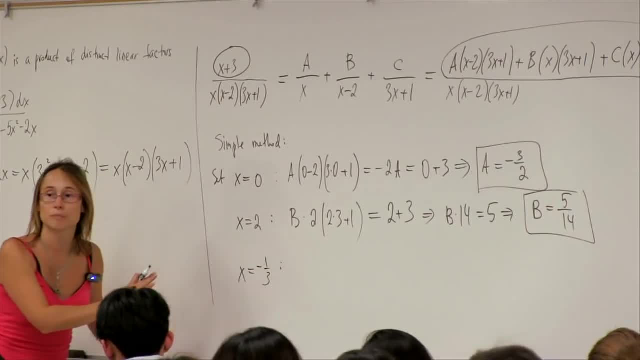 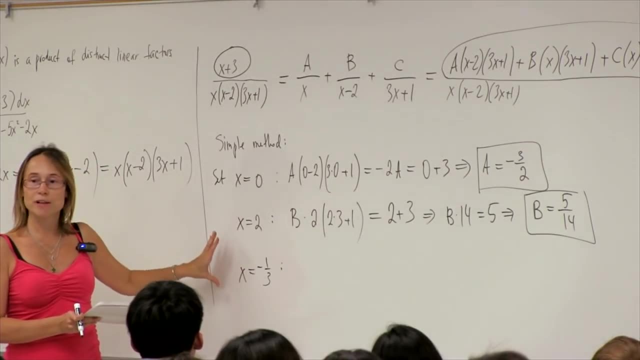 0, 2 and minus 1 third. these are the ones that work. any other choice would also work, but make the math a lot harder. so this is a clever choice of the values of x that make the calculations the easiest, so when x is minus 1 third, 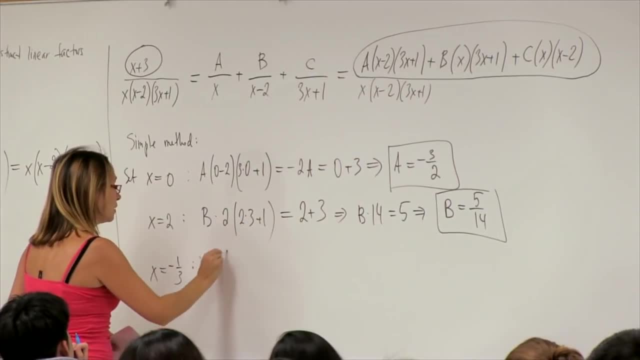 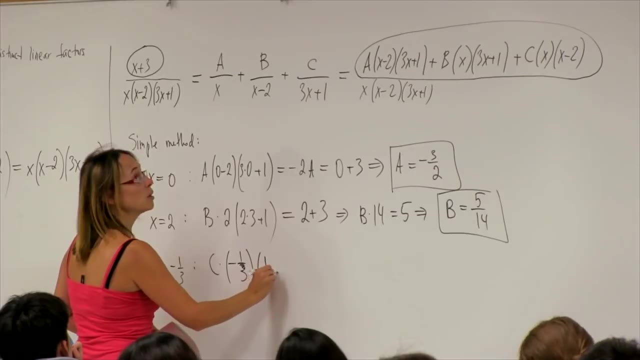 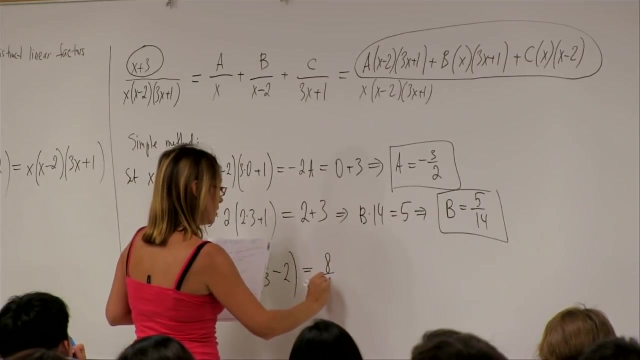 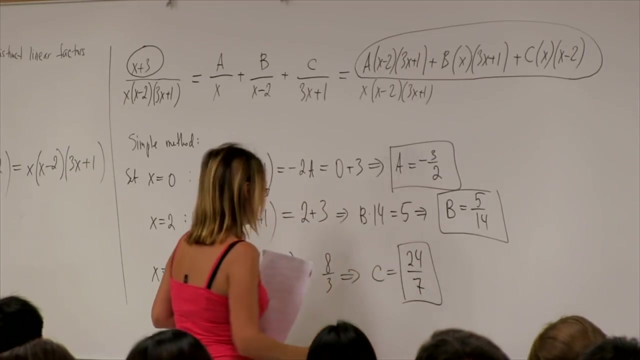 the first and the second terms are 0 and I have c times minus 1, third times 1 minus 1. third minus 2 is equal to 8 thirds, so c is 24 over 7 if I solve for this. so what is the result? 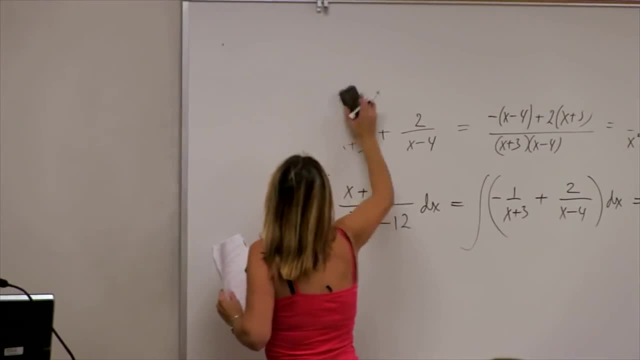 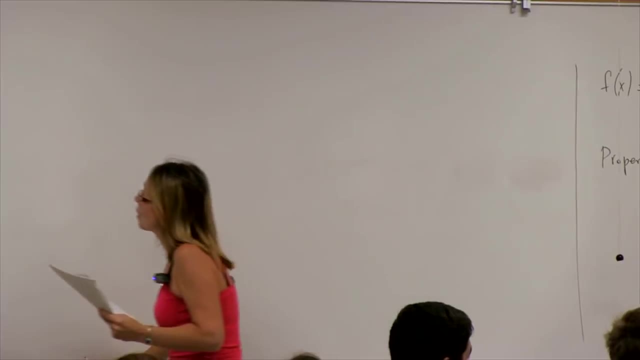 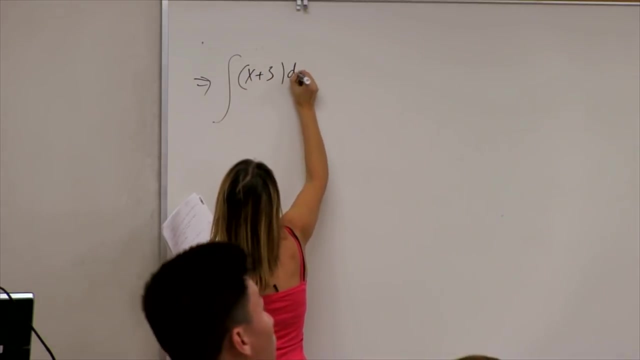 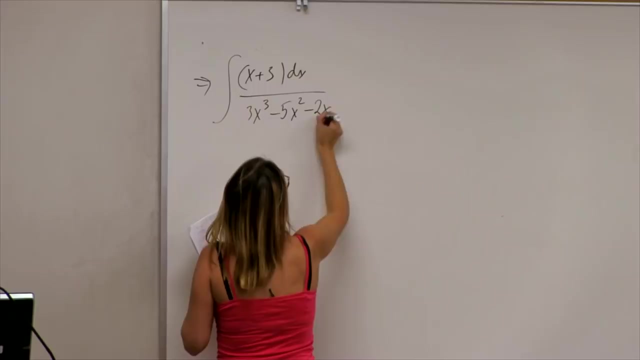 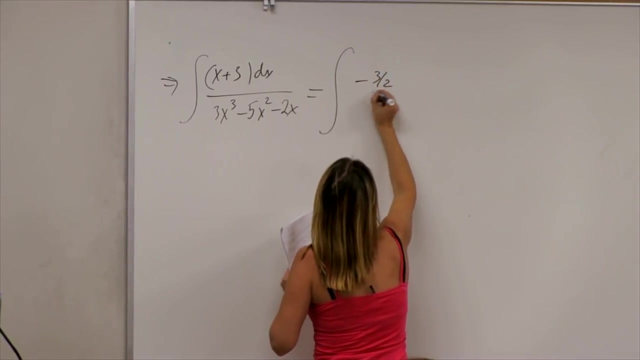 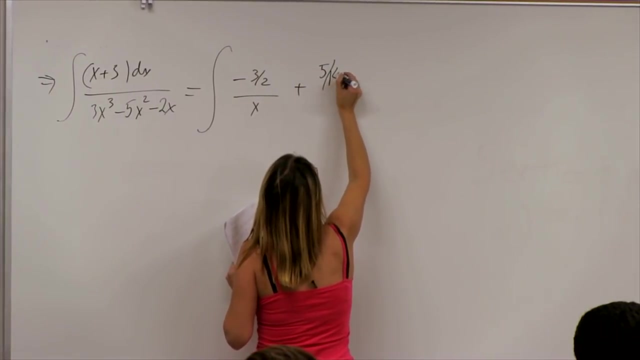 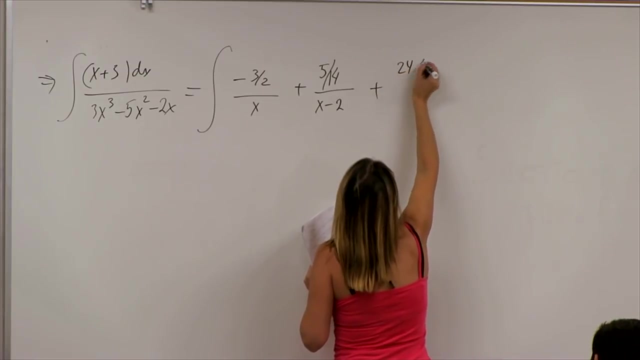 of this calculation, the given integral x plus 3 dx 3x cubed equals the integral of the partial fraction. so I substitute minus 3. halves over x plus 5, fourteenth over x minus 2 plus 24, seventh over 3x plus 1. 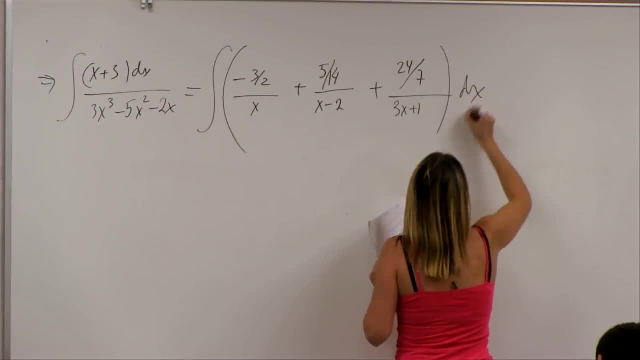 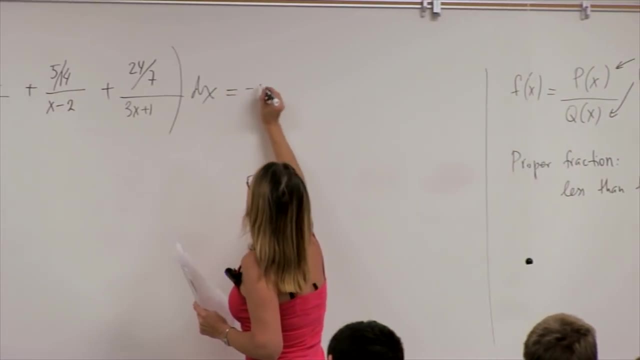 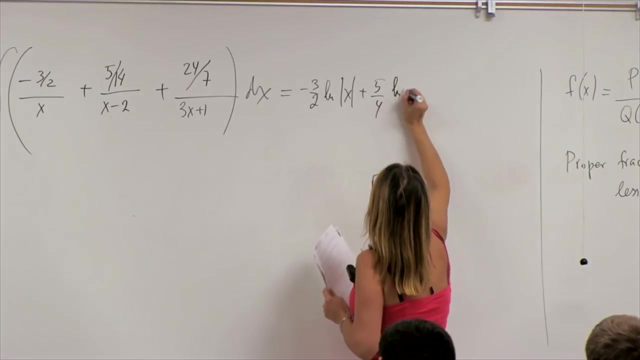 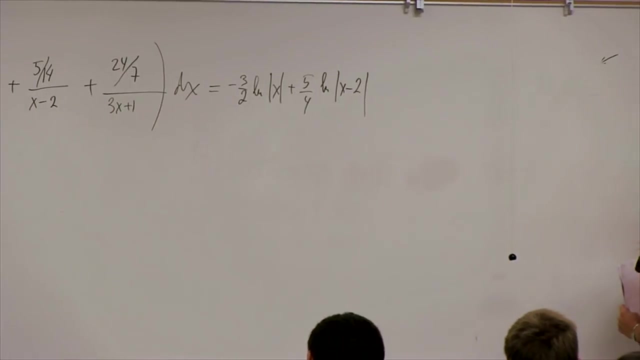 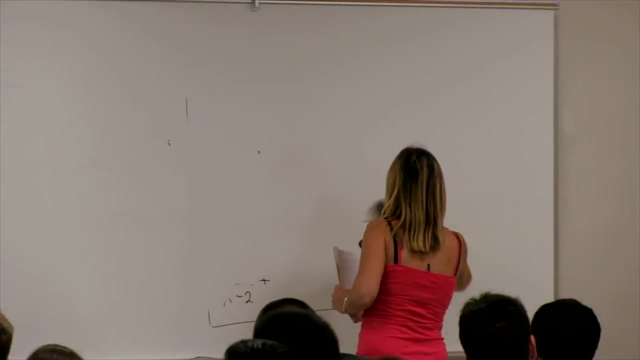 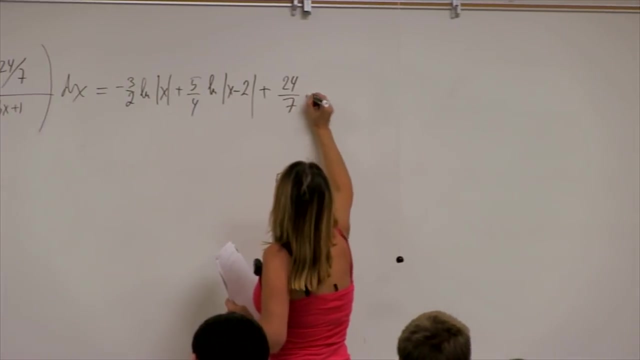 dx and you can see that this is easy. it's just the sum of 3 logarithms minus 3. halves: log x plus 5. fourth log x minus 2. log x minus 2 plus 24. over 7: log 3x plus 1. 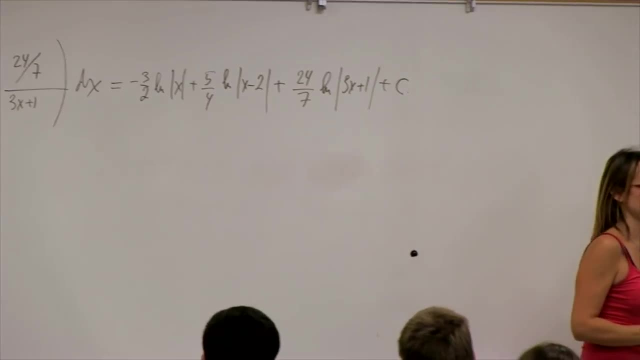 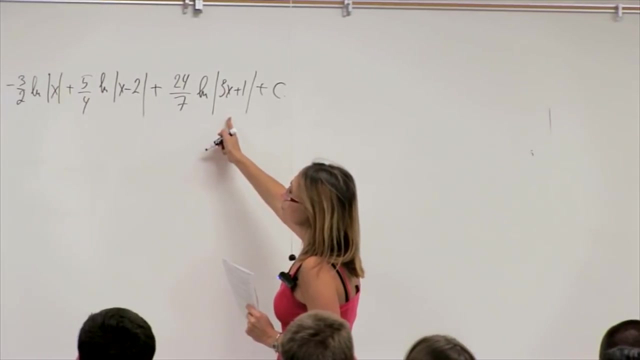 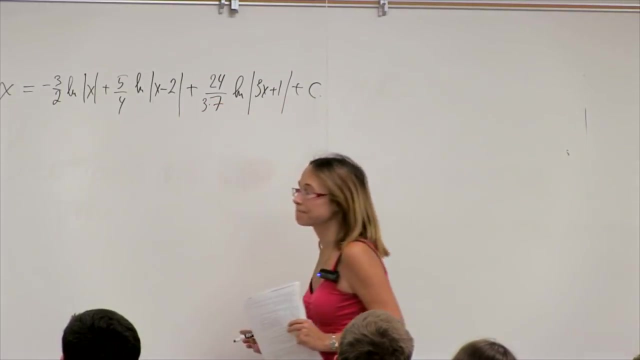 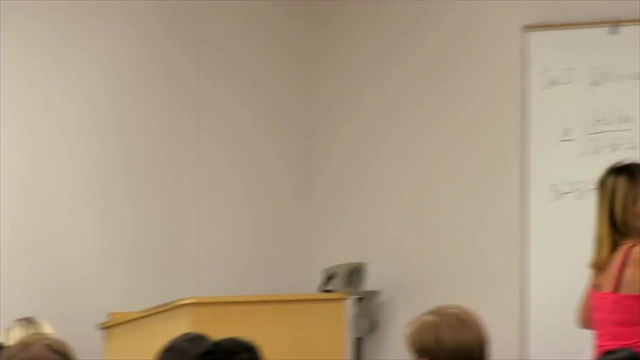 plus c questions: 3x plus 1 over 3, 3x plus 1 over 3. you're right, thank you. so what's that other method that I didn't mention here? so the first method: I just look for convenient values of x and write down three equations. 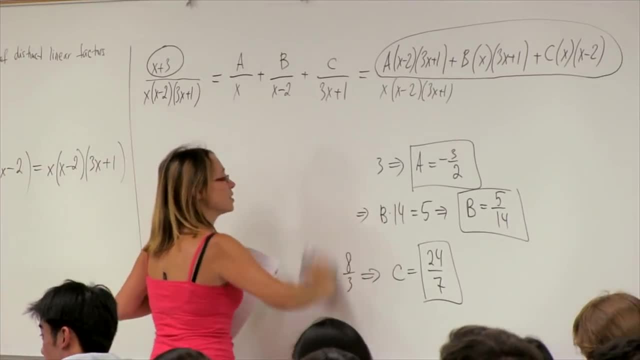 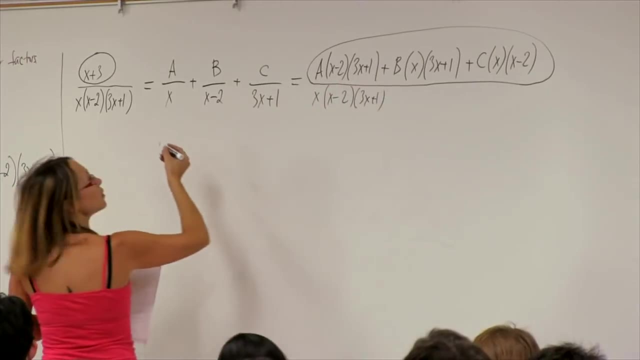 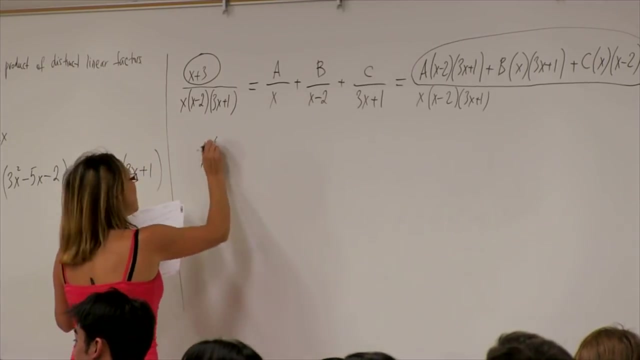 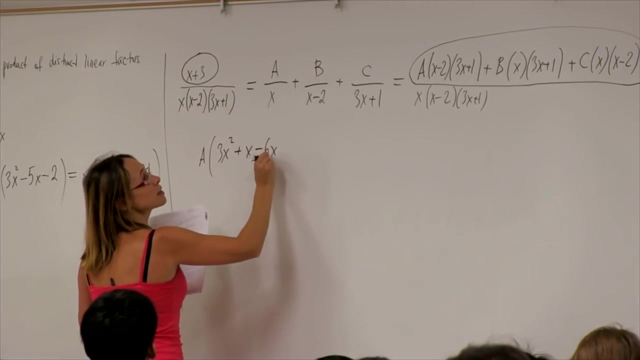 so the more general method is as follows. I look at the right hand side, ok, and I rewrite it by multiplying everything through. so I'm going to have a quadratic equation for x here. so 3x squared plus x minus 6x, minus 2 plus b. 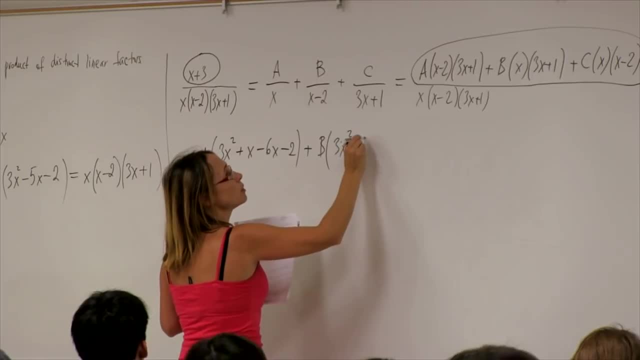 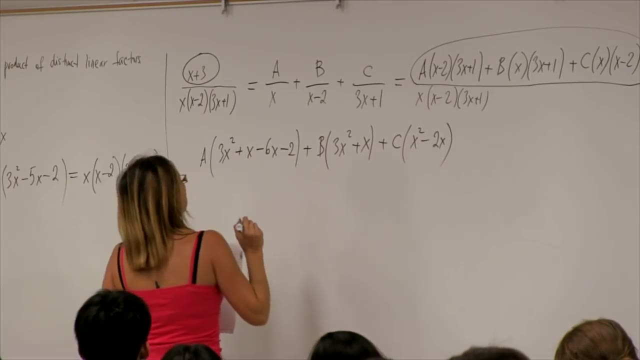 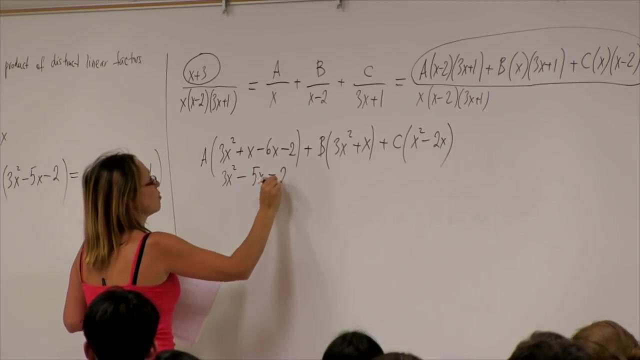 I multiply all the x's right: 3x squared plus x plus c, x squared minus 2 minus 2x. now I simplify a little bit. so this is 3x squared minus 5x minus 2, nothing else to simplify. and now I want to collect. 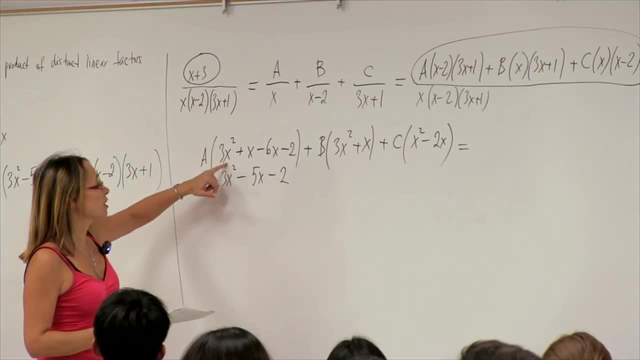 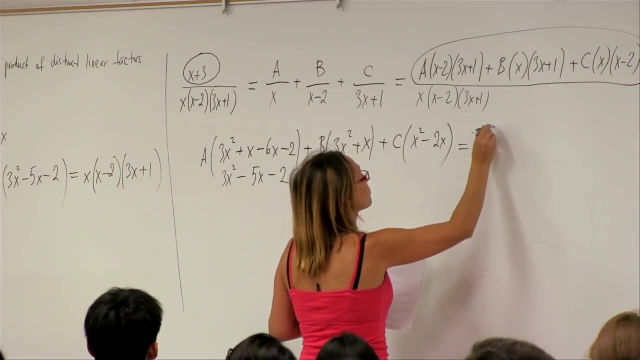 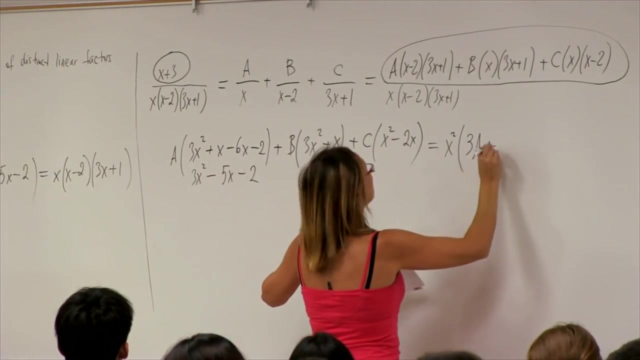 the coefficients in front of each power of x. so I have a second power of x, I have a first power of x and I have a zero power of x. so in front of x squared, what do I have? 3a? here I have plus 3b. 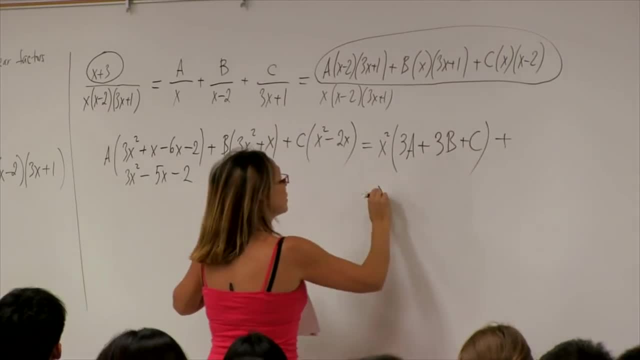 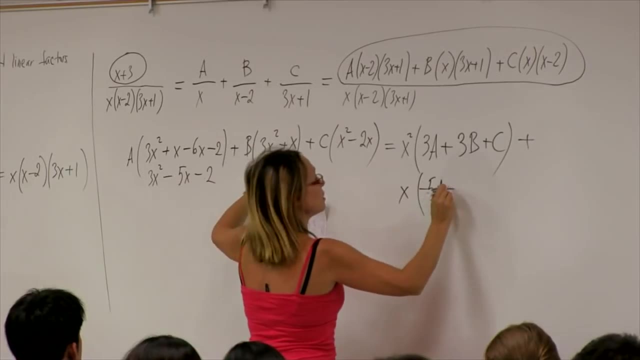 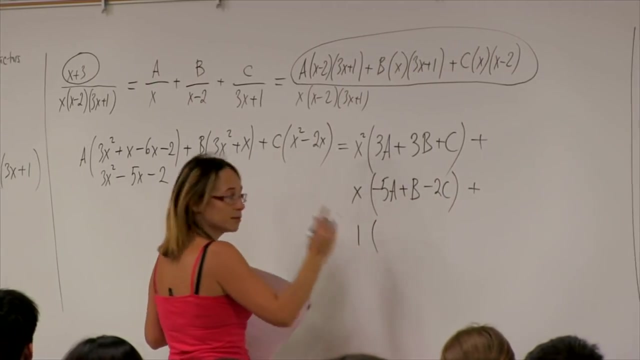 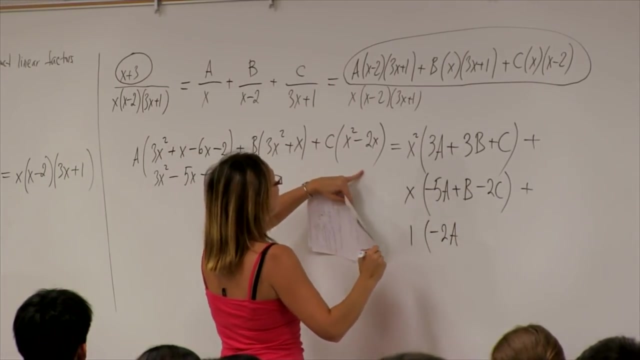 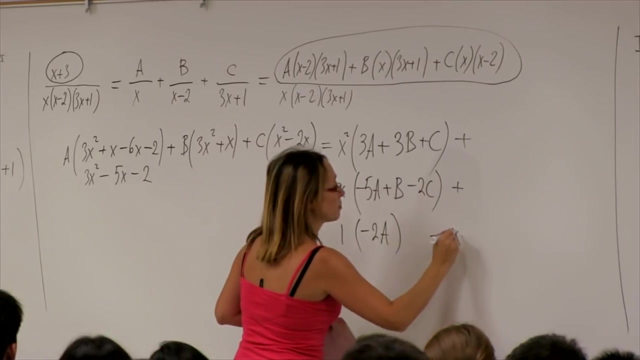 plus c. ok, in front of x, I have minus 5a, plus b, minus 2c, and in front of 1- basically terms that don't contain x- I have minus 2a. nothing here and nothing here. this has to be equal to x plus 3. 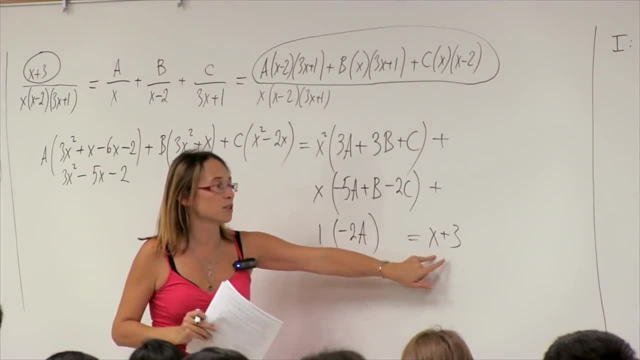 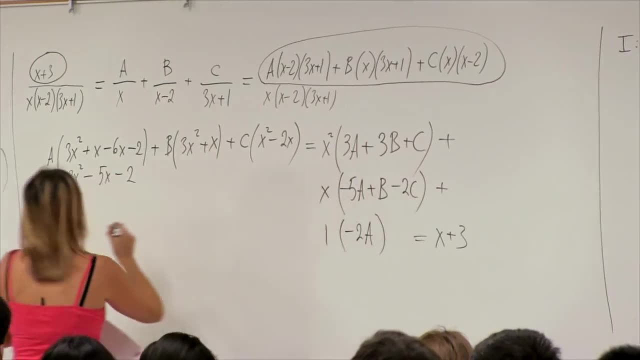 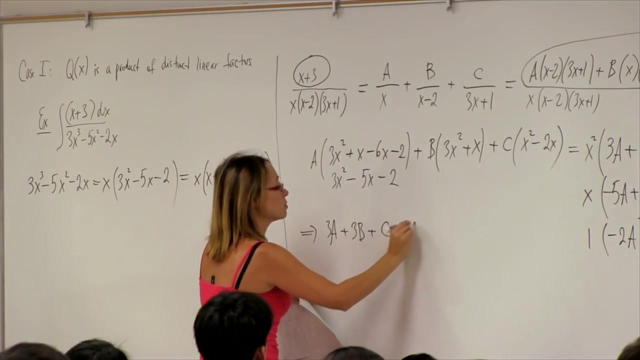 so now I compare the powers of x. what is the coefficient in front of x squared here? obviously it's zero, right? so the coefficient in front of x squared has to be zero. so my first equation becomes: 3a plus 3b plus c must be equal to zero. 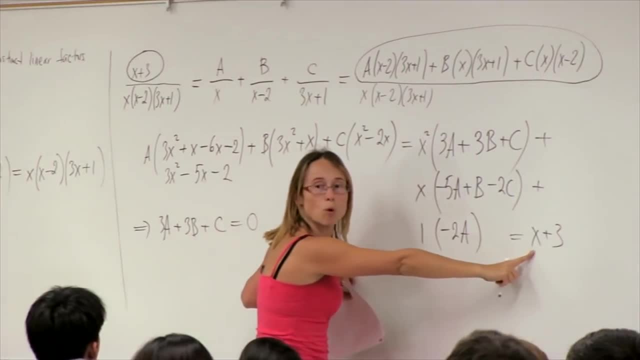 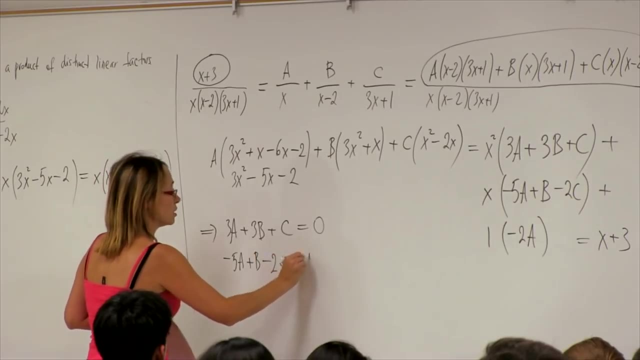 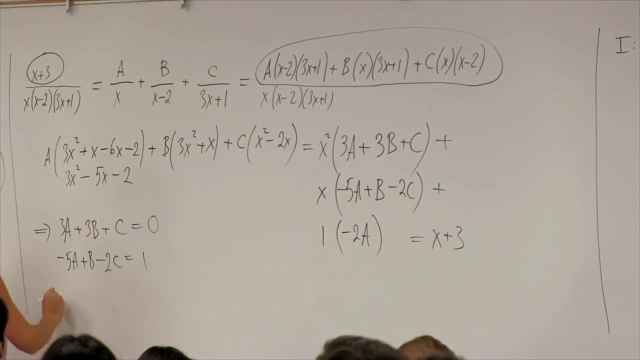 the coefficient in front of x has to be 1. so my second equation is: minus 5a, plus b, minus 2c is 1. the coefficient in front of the term that doesn't contain x must be equal to 3, so minus 2a. 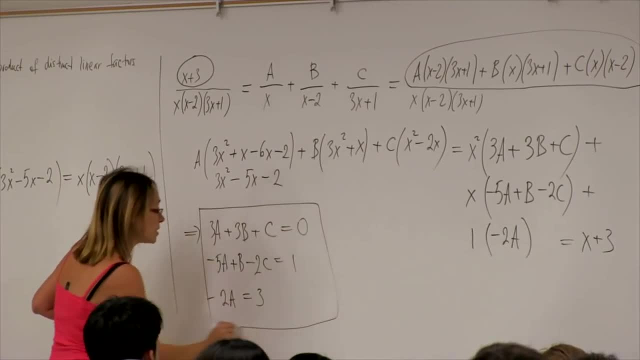 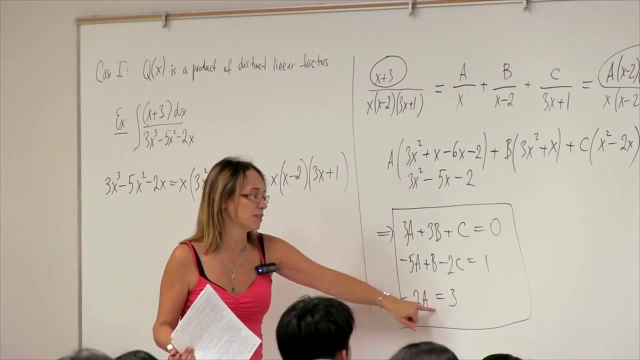 is equal to 3, so this is a system of 3 linear equations. ok, that I can resolve. for instance, the last equation actually gives you minus 3 halves, which is the same as the first equation, which is the same as I obtained by the simple method. 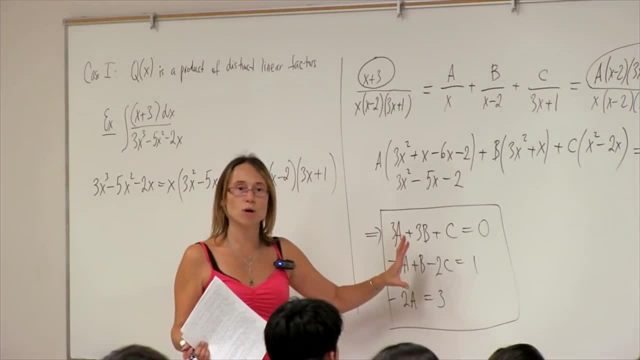 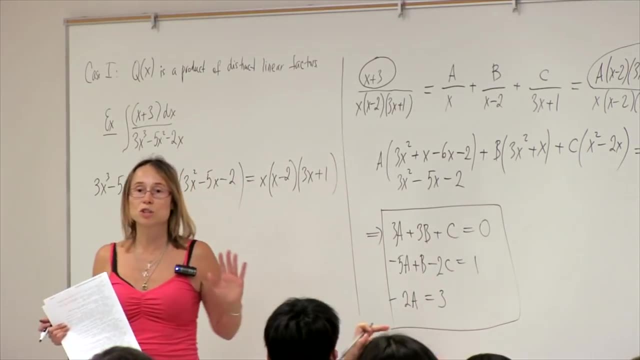 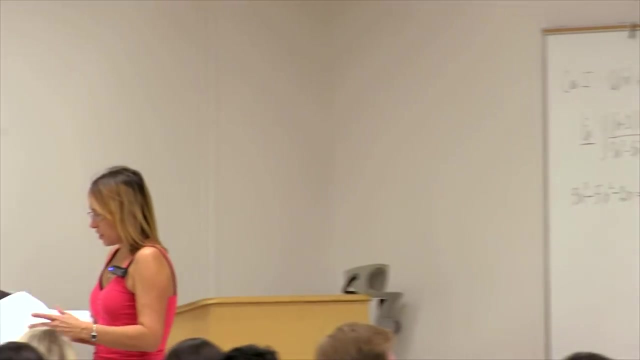 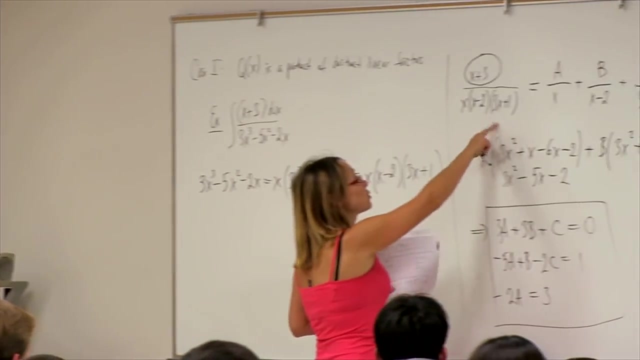 from knowing a, I can solve these two. it's a little bit more involved, but it always works ok. so it's your choice which method to choose. students usually prefer the simpler method. fine, so this shows you an example of a fraction whose denominator consists of distinct linear factors. 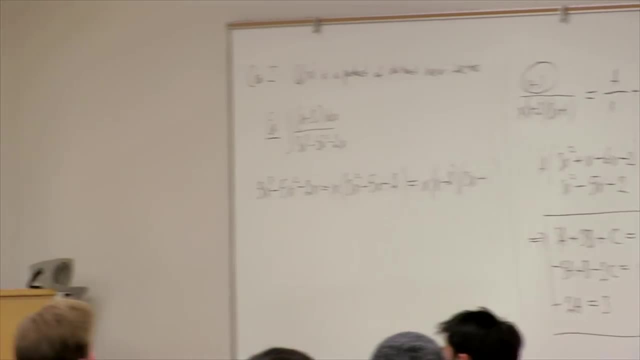 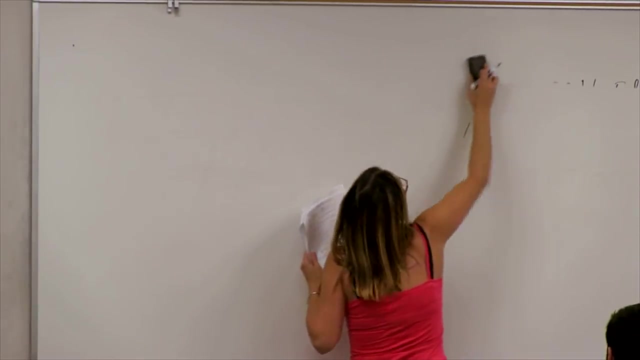 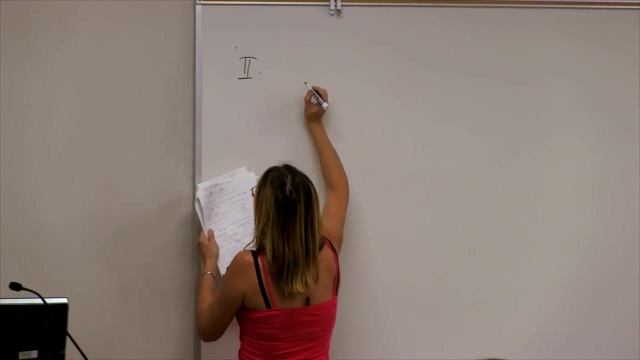 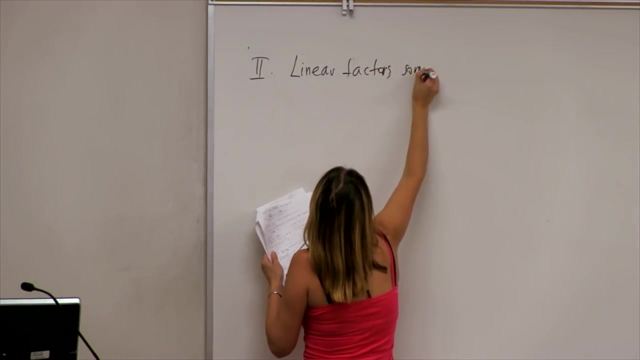 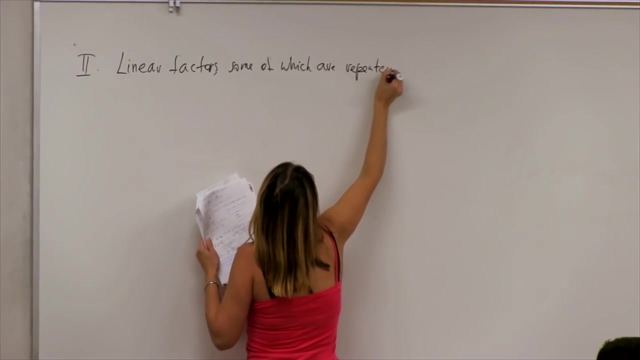 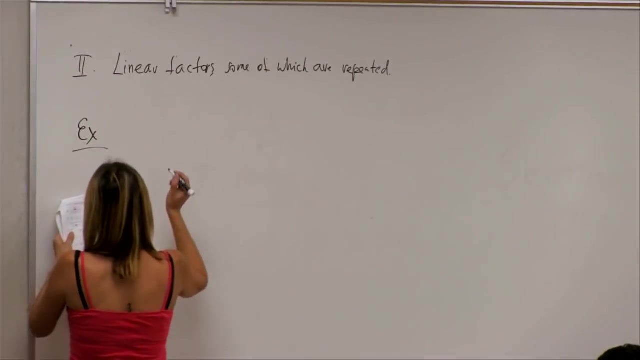 so what else can we have? in the second case, so case number 2, we can have linear factors, some of which are repeated. ok, so here's an example. first of all, we establish that this is a proper fraction question. yeah, I'm just a little curious. 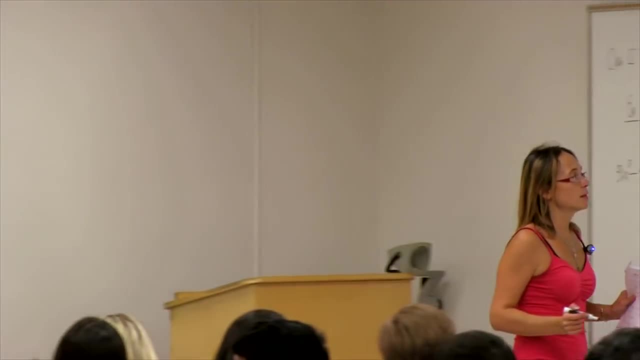 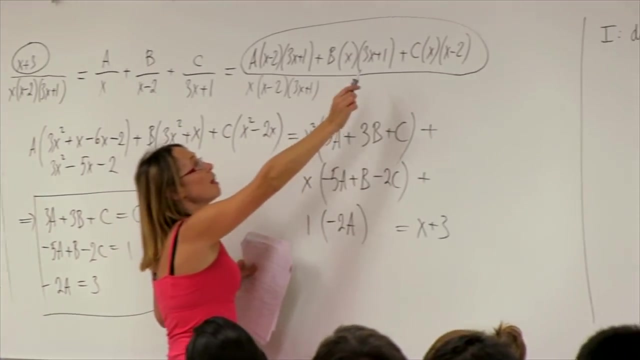 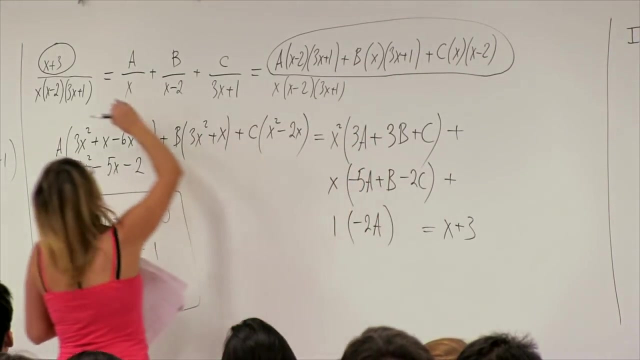 the three equations that ended up defining what the values were. how did you come up with those? ok, so first I multiplied this whole through and collected the powers in front of x, squared x and 1. ok, and this is supposed to again be equal to the left hand side. 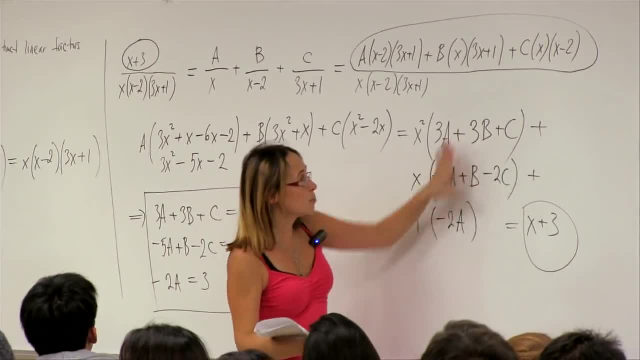 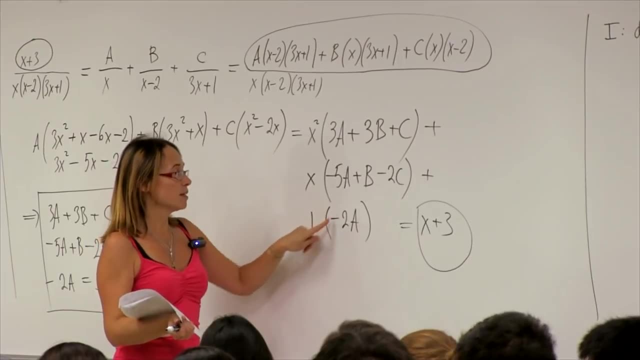 x plus 3. so this is a polynomial in x that contains. so this is the coefficient in front of x squared. this is the coefficient in front of x. this is the remaining coefficient. it's supposed to be equal to this on the right: the coefficient in front of x squared. 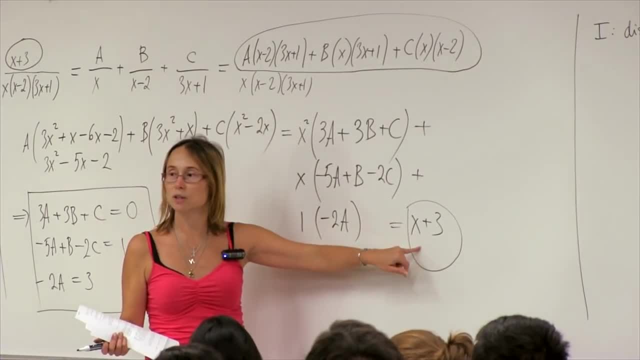 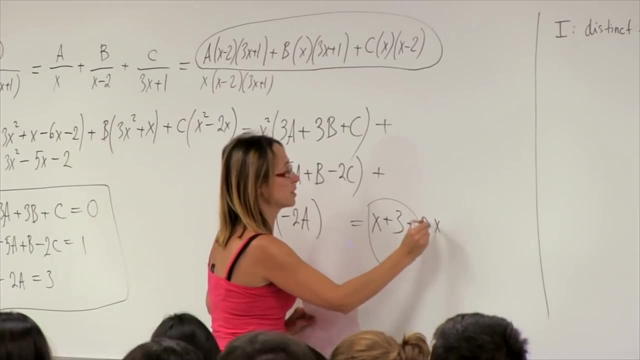 is 0, right? it doesn't have x squared. x plus 3 does not have x squared. so formally speaking, we can say that it's 0 times x squared. so this coefficient in front of x squared has to be equal to this coefficient in front of x squared. 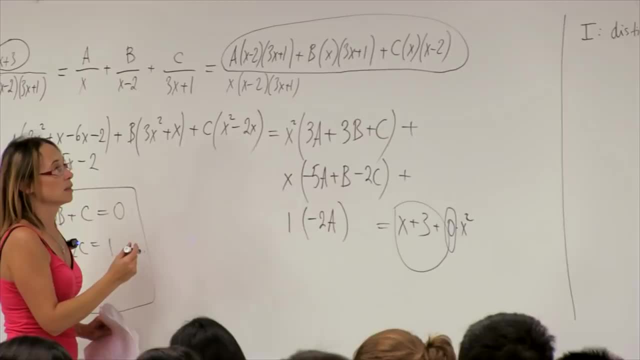 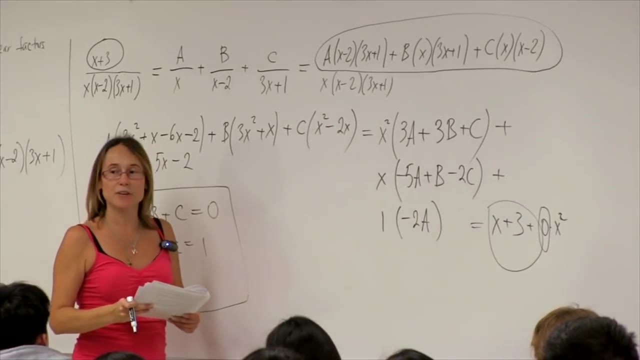 for the two functions to be exactly the same, so each individual one has to be equal to that part. so we view the right hand side and the left hand side as polynomials in terms of x and we equate the coefficients in front of equal powers of x. 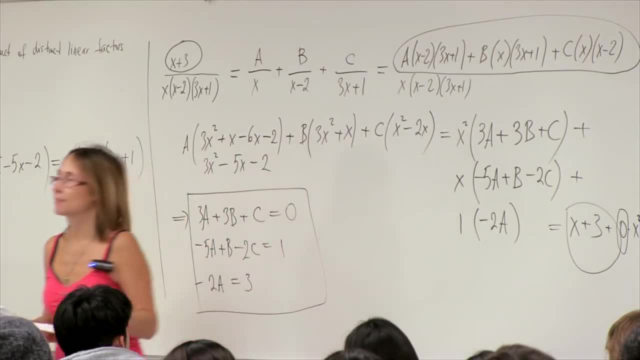 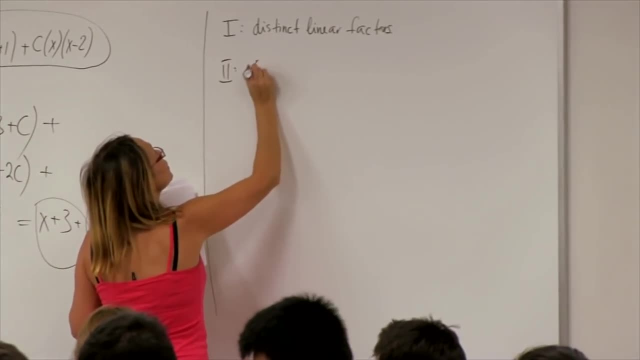 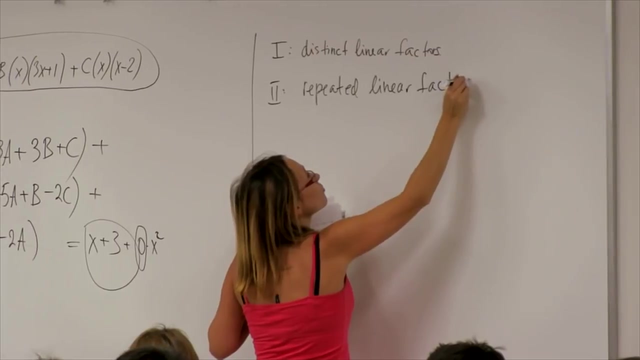 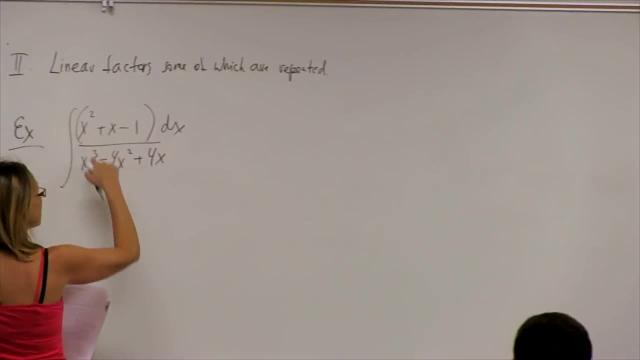 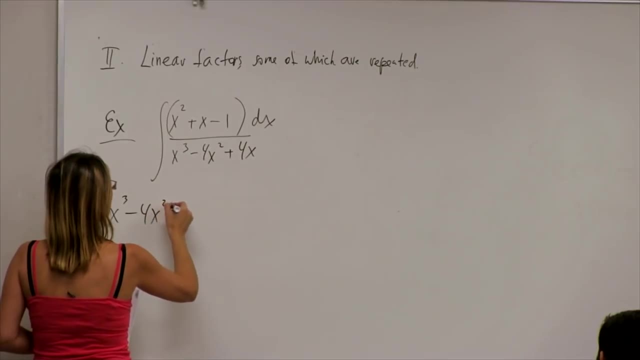 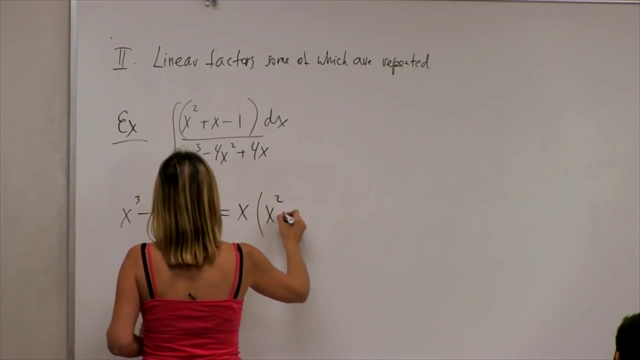 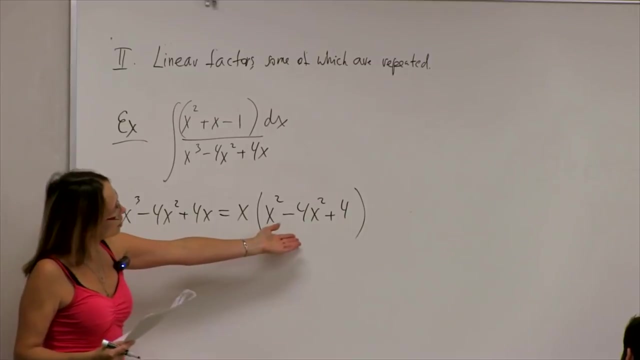 it's easy to see that this is a proper fraction: second power divided by third power. so we're good here and let's write down the denominator and try to factor it out. so, again, x comes out and what's left is this polynomial. so there are two ways. 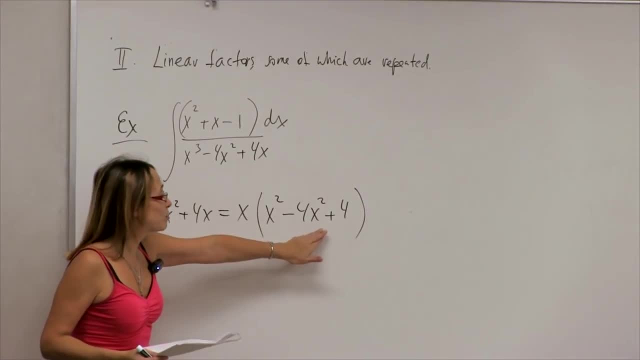 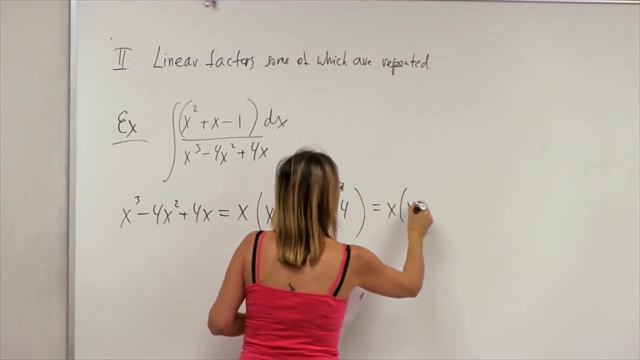 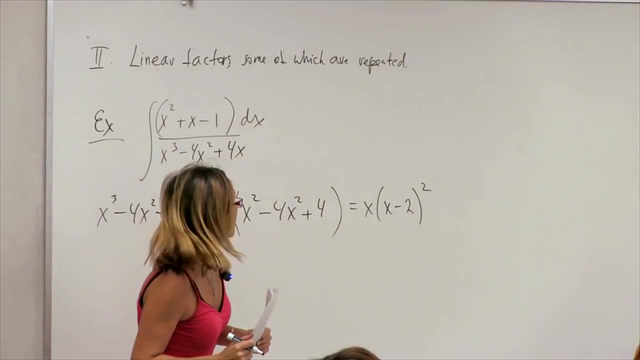 to deal with this. you can either take the roots of this or you can simply recognize this as a full square. so it's x times x minus two squared. if we were to look for the roots, we would have two roots that are the same question. yes, oh, thank you. 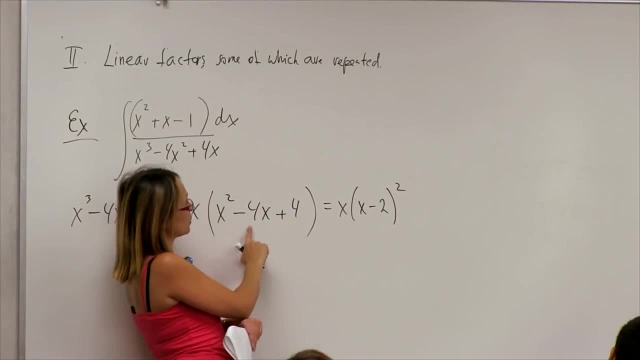 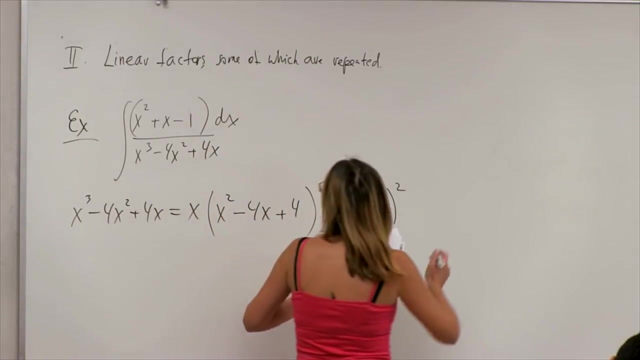 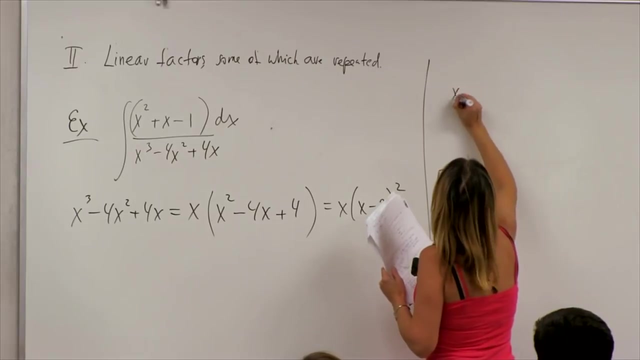 thank you very much. thank you. so there are going to be two repeated roots, which are two in this combination. so we have a factor of x and two identical factors, x minus two. so if I blindly use the previous method, what would I do? I would have to say that. 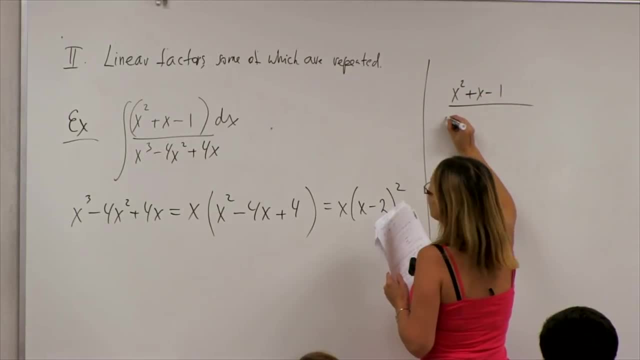 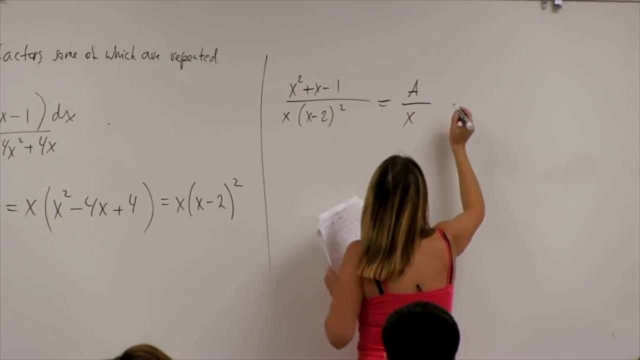 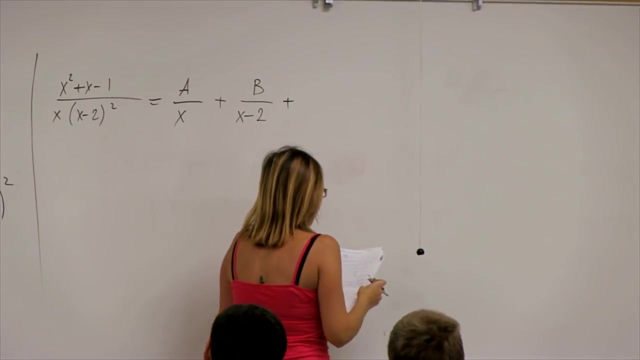 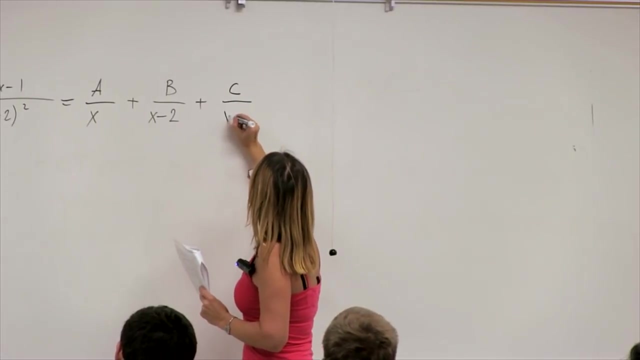 x squared plus x minus one. x x minus two squared. let's represent it as partial fractions. so the first one is a over x minus two. but what else do I put there? okay, if I blindly use the previous method, I would have c over x minus two. 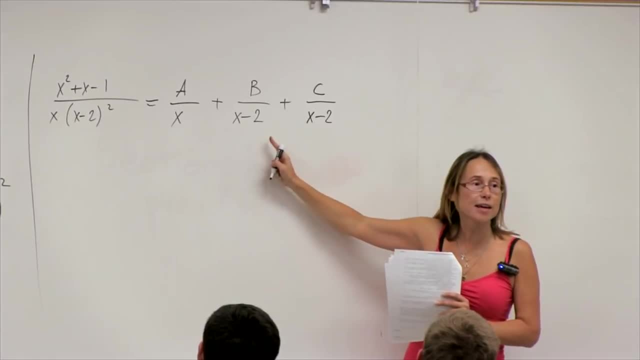 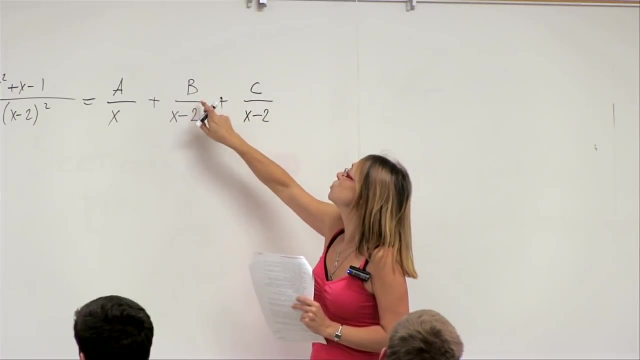 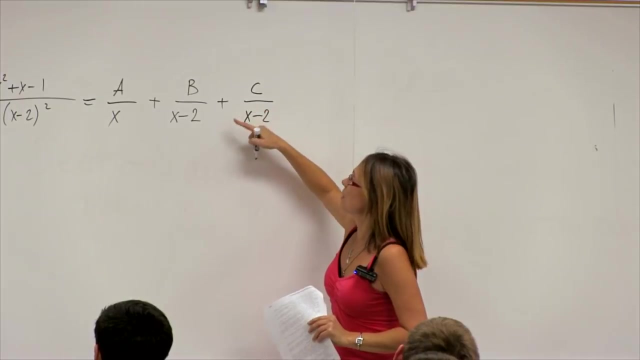 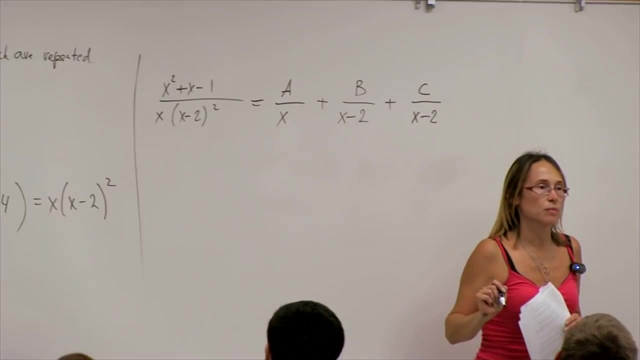 because these are two factors and, as you can see, these are the same. so by redefining a new b to be equal to b plus c, I would just have this combination and then when I make, when I bring it to a common denominator, I would be. 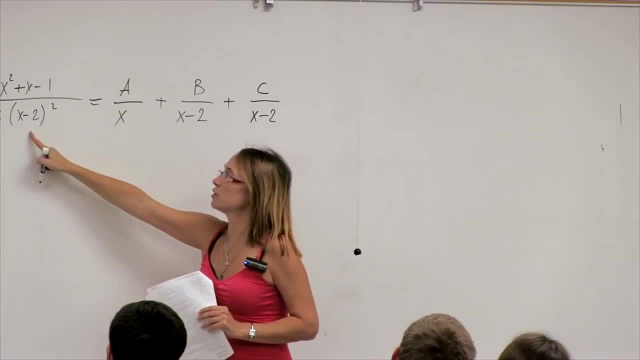 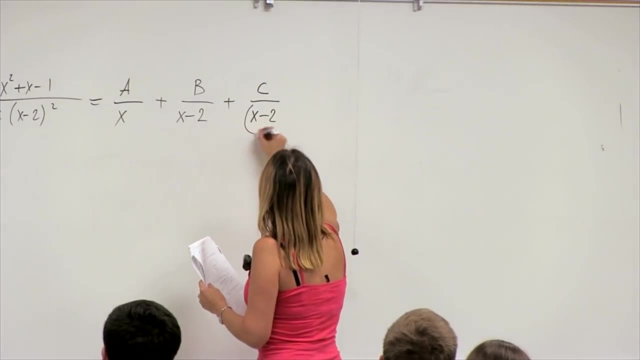 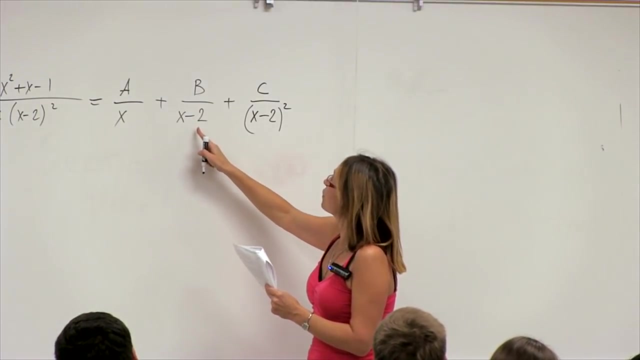 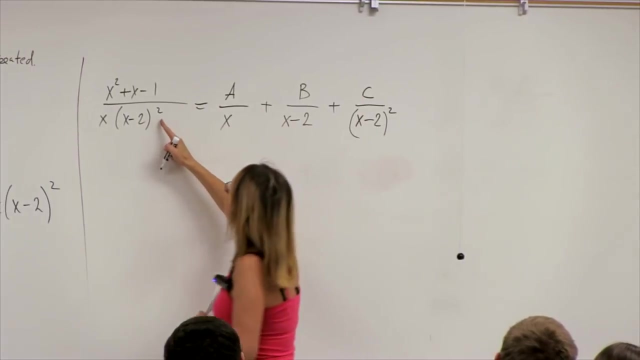 missing one power of x. okay, so it simply doesn't work. I don't have enough different denominators to use the old approach, so instead of this, we do the following: okay, this is the method we have. there are factors x minus two. for instance, if we had 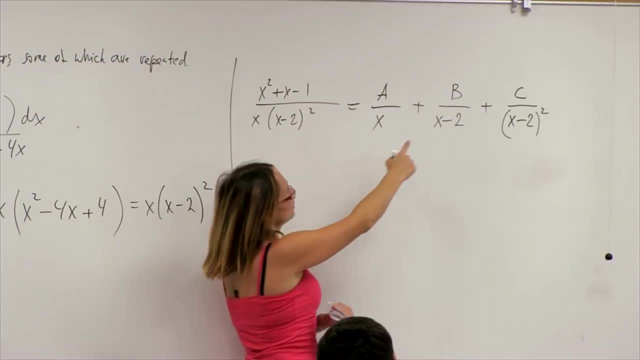 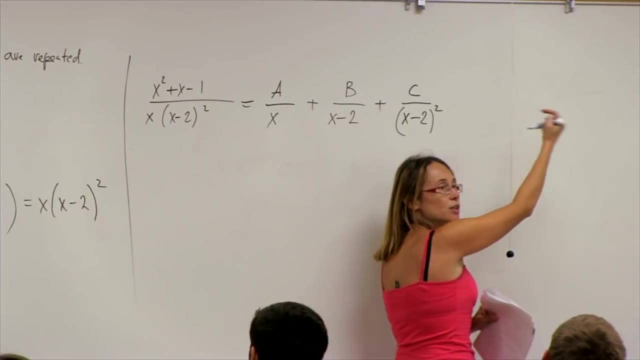 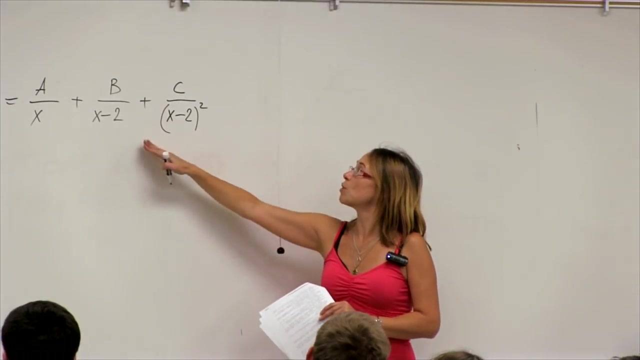 x minus two to the power seven. what would we put here? b over x minus two plus c over x minus two, squared plus d of the same thing, cubed, and so on, up to the power seven. so we would have seven terms all containing different powers of x minus. 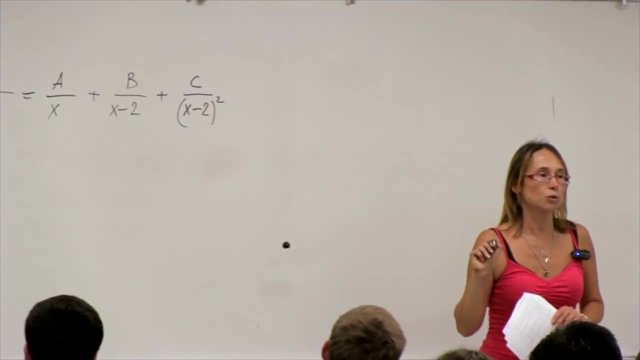 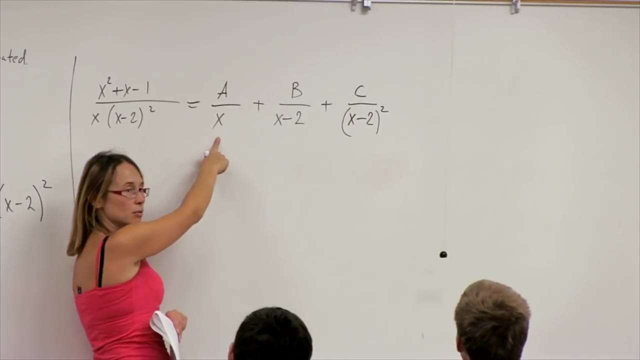 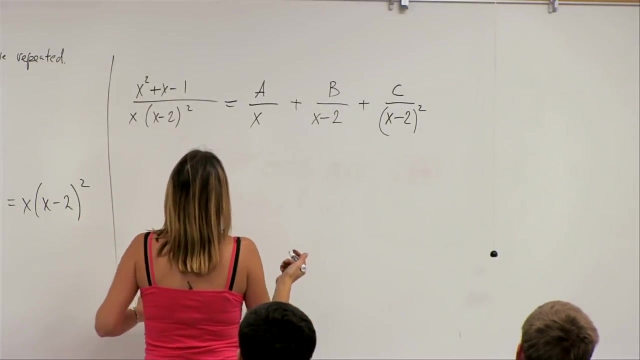 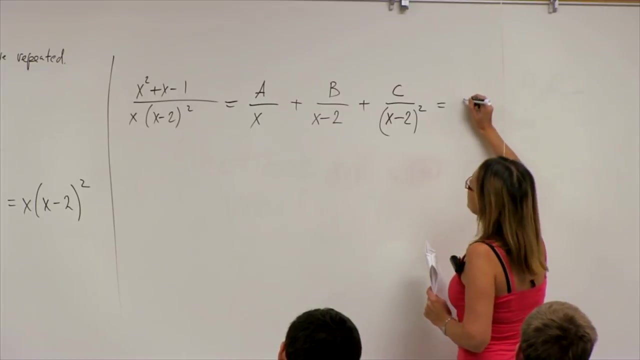 two up to the highest coefficient. okay, so this is a modification of the method. when we have a repeated factor, the non-repeated factor comes, just as before, separately with its own coefficient. okay, so now let's go through the calculations. we are going to bring this to a common 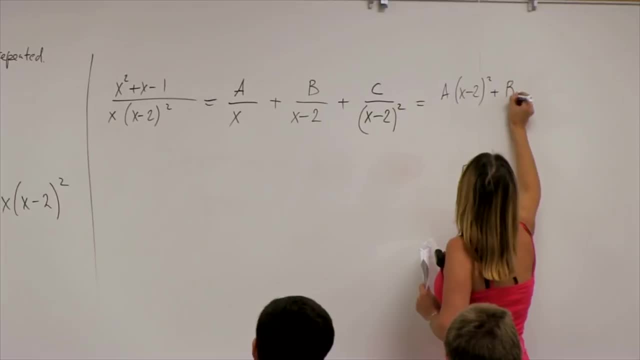 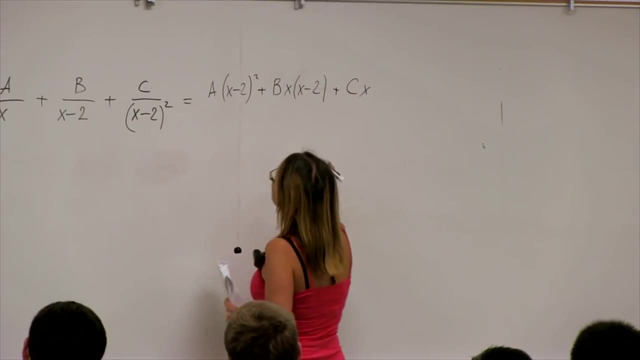 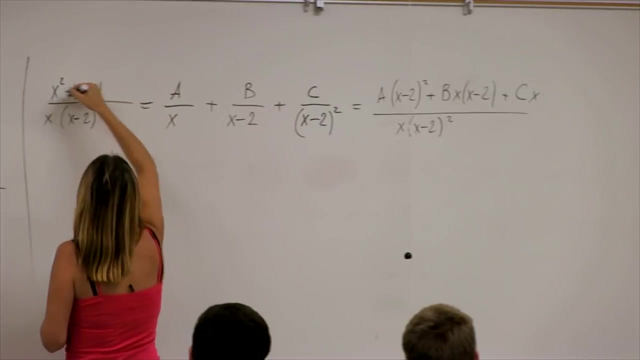 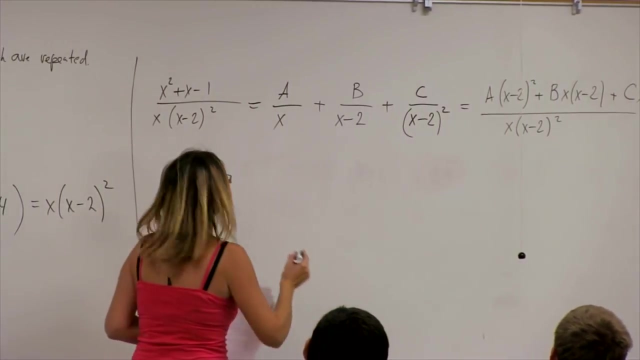 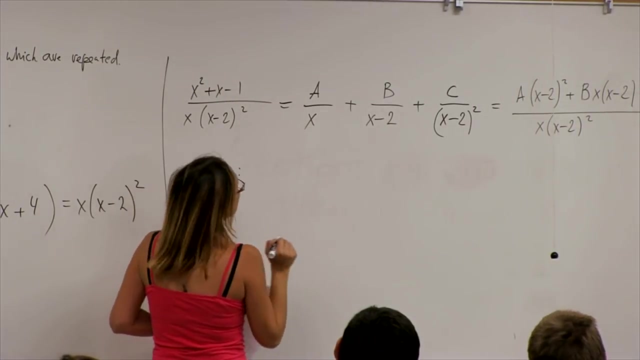 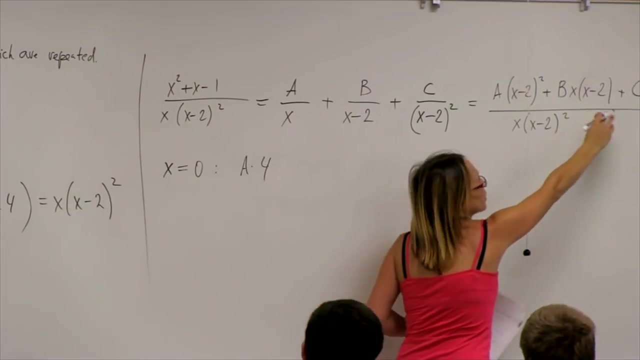 denominator like this, and we have to make sure that the numerator on the left is equal to the numerator on the right. I'm going to try easy values of x. okay, what are easy values? the first one is obvious: it's zero times four. and these two are killed. 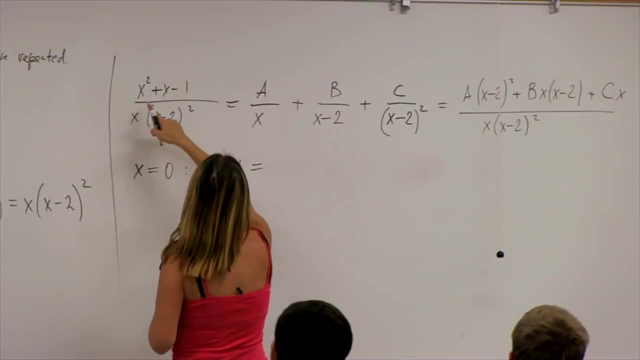 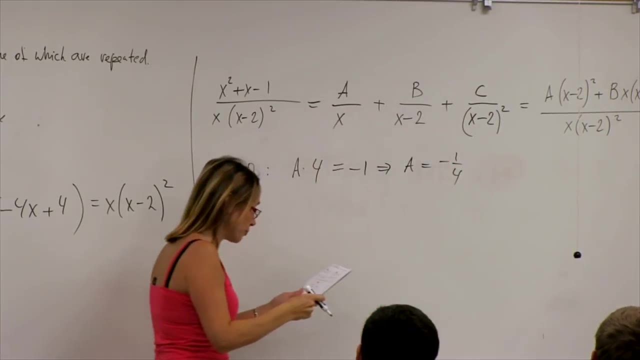 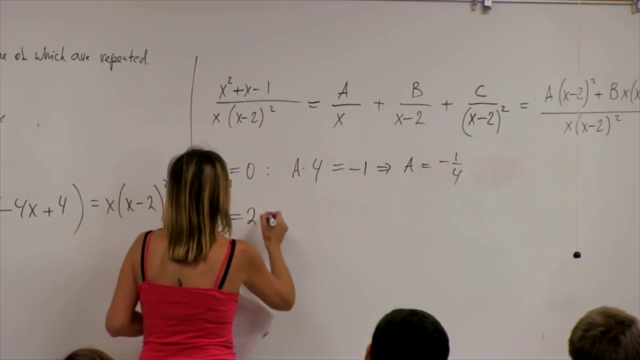 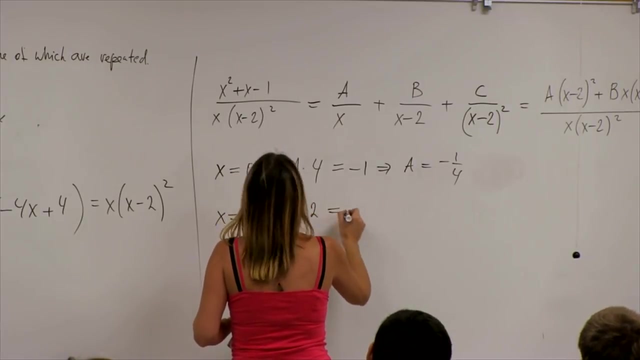 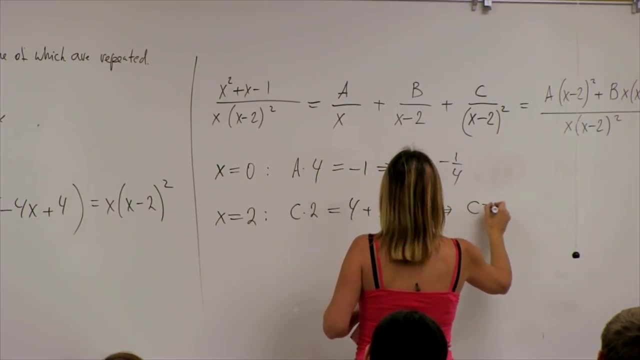 okay, equals. on the left I have zero plus zero minus one, so a immediately comes out as minus one quarter. okay, now what's another good choice? two: so this one is zero. this one is easy. also zero c times two, four plus two minus one, six, five, so c. 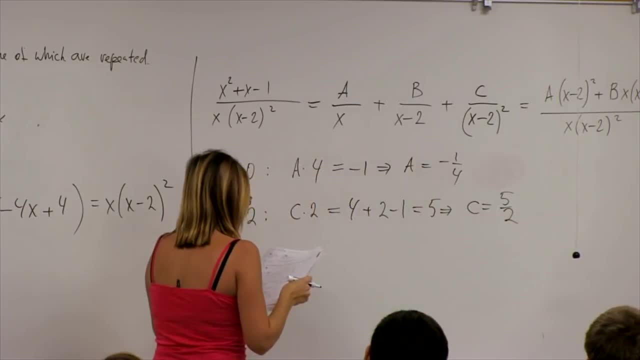 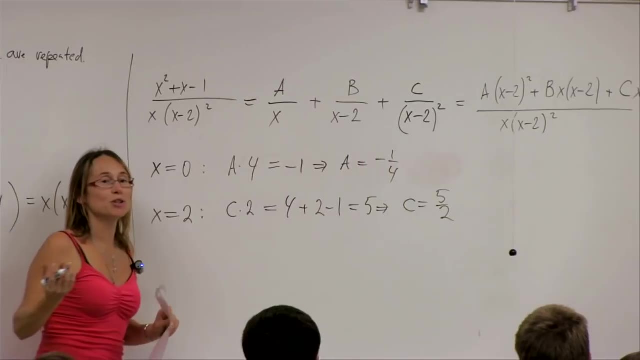 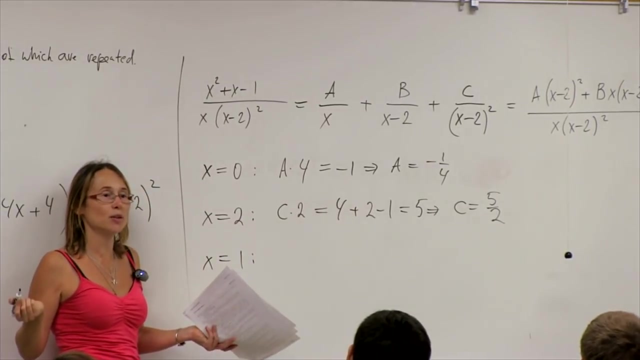 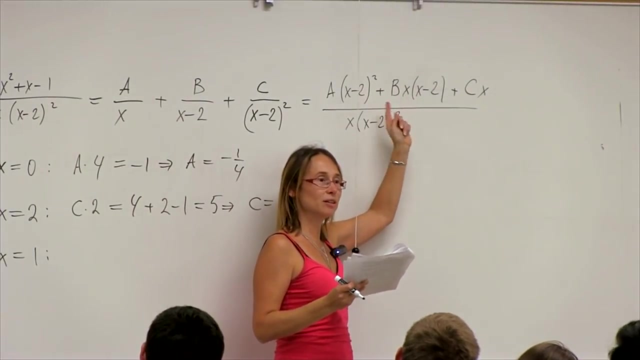 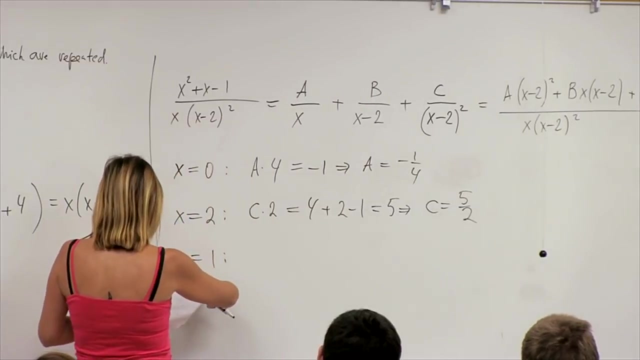 is five halves excellent, and I ran out right. there is no other root. so what do I choose? usually I suggest you stick in something that looks easy. okay, just have different roots that make them zero, but it will make them look nice and easy to operate. so if we 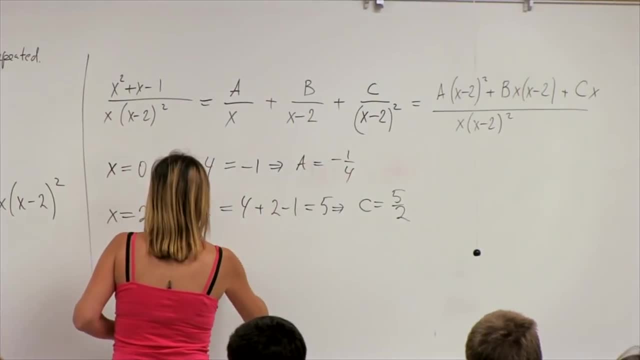 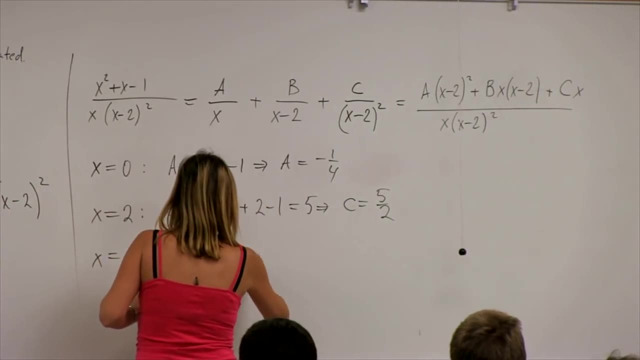 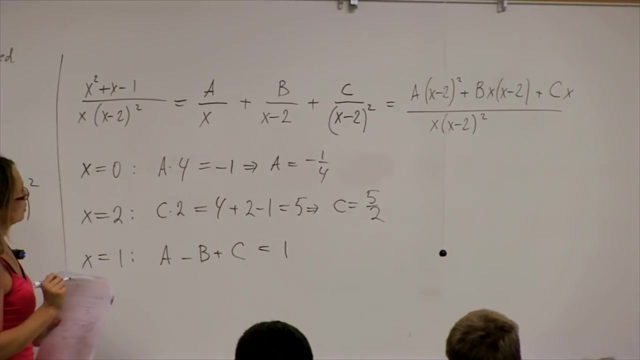 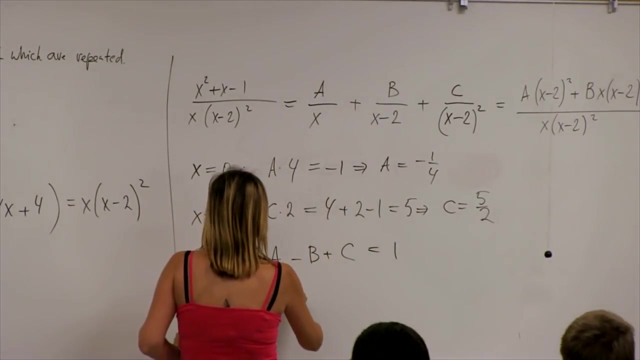 take x, equals one. what do I have? a plus b. um, actually, with a minus minus b plus c, not so bad, equals one, okay. so this equation can be solved because I already know a and c. so minus a quarter, uh, minus b plus five halves equals one. 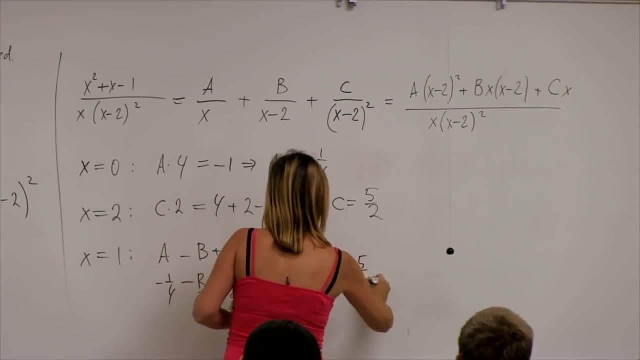 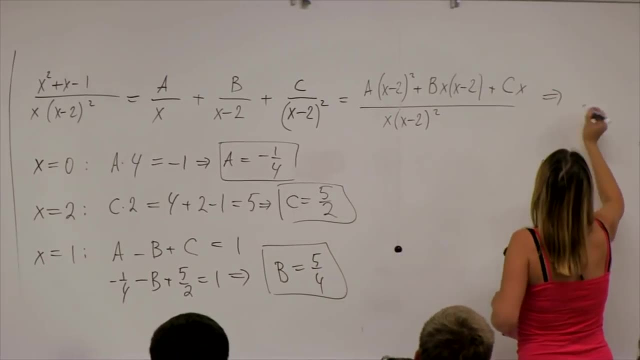 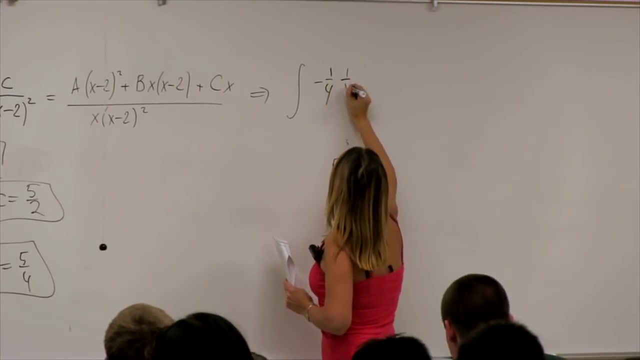 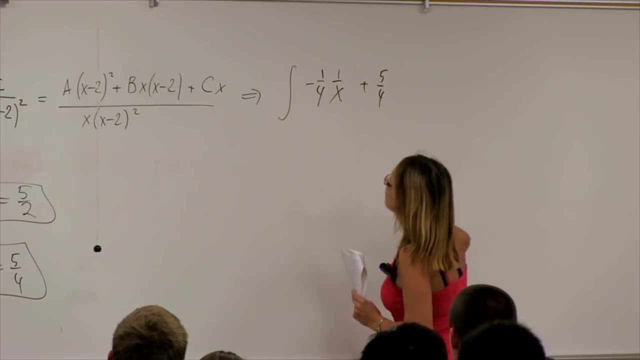 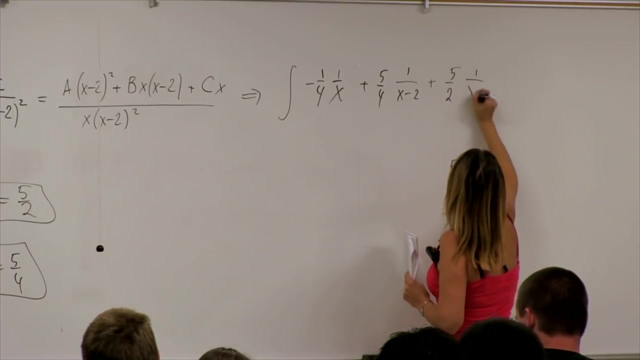 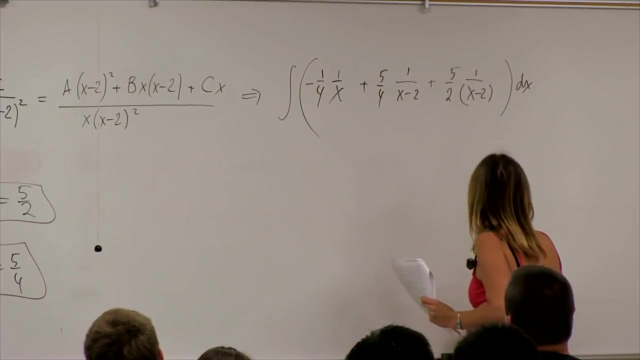 gives me b, uh, five quarters. so these are my coefficients and I can write down the resulting integral: minus x over x plus five over four, x minus two plus five halves, x minus two squared dx. is this an easy integral? yeah, it's not so bad, we're going to have 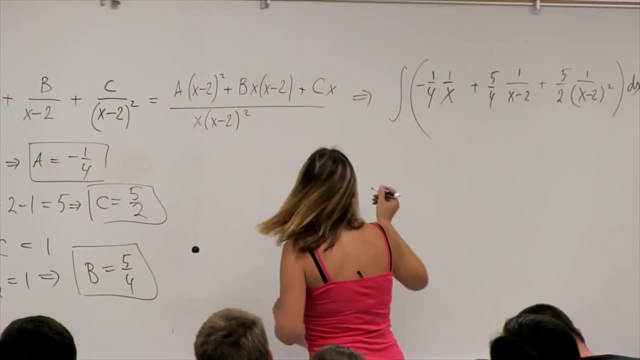 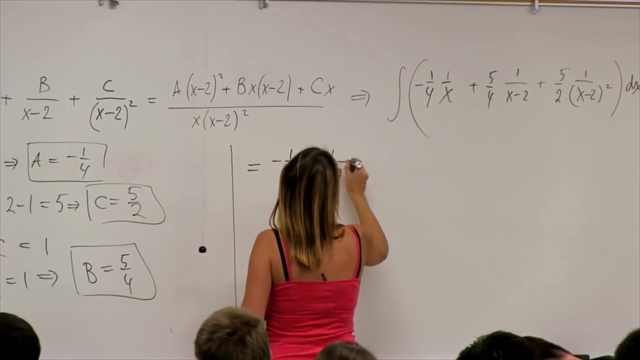 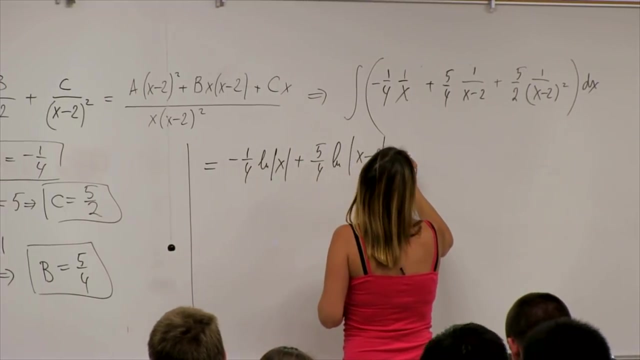 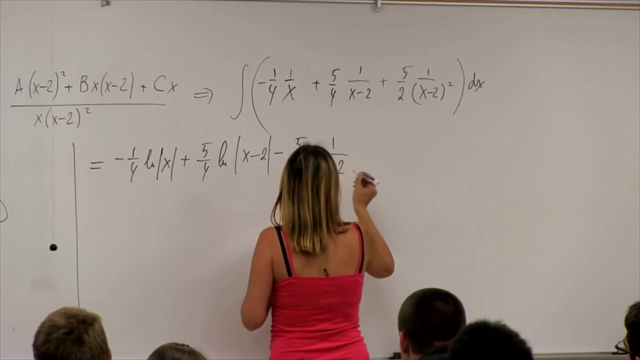 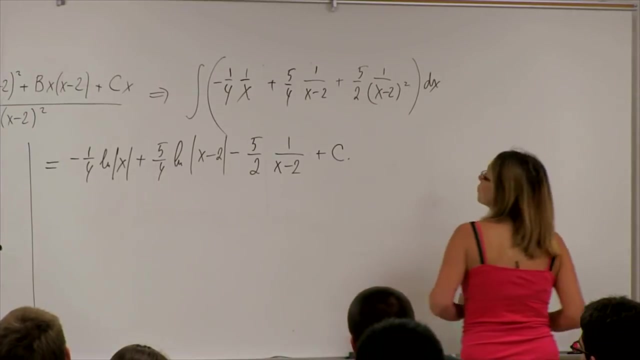 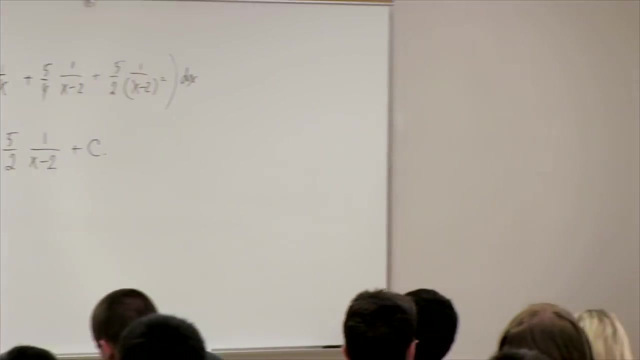 a couple of logs and something else, right, uh, so let's do it: minus a quarter log x plus five quarter log. x minus two minus five halves, x minus two um plus c. okay, so this is a simple integral. okay, so I have a fraction of x squared. 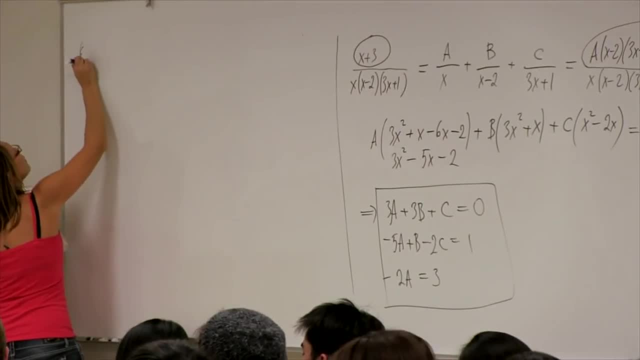 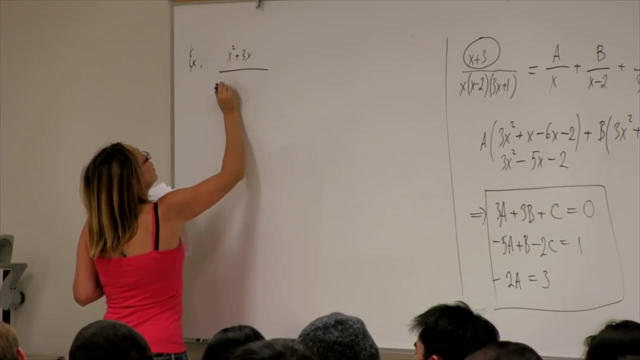 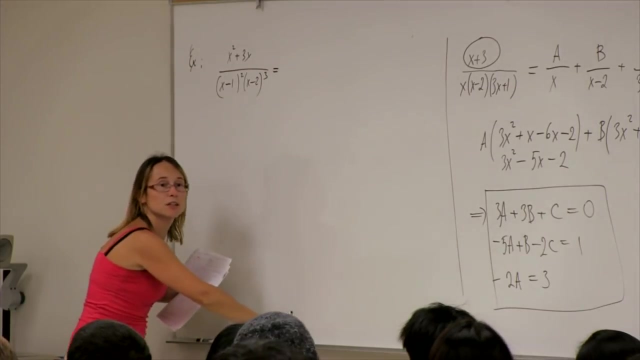 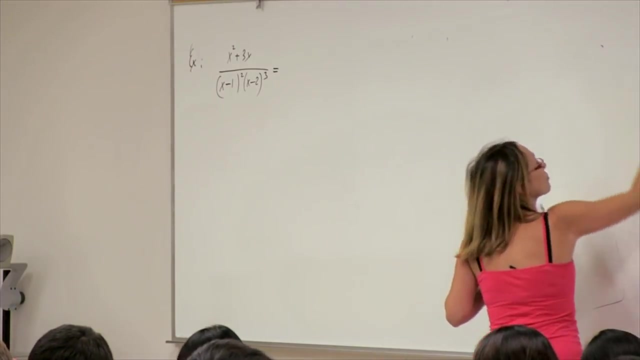 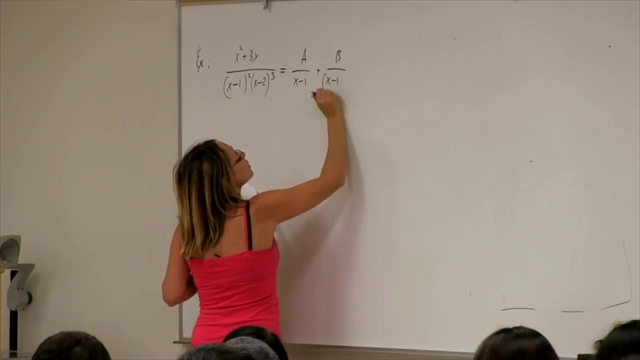 so I have a fraction of x squared. so I have a fraction of x squared. so I have uh, two different uh linear factors, each of them repeated. so I would have to write the following: a over x minus one plus b, x minus one squared, and that's it. 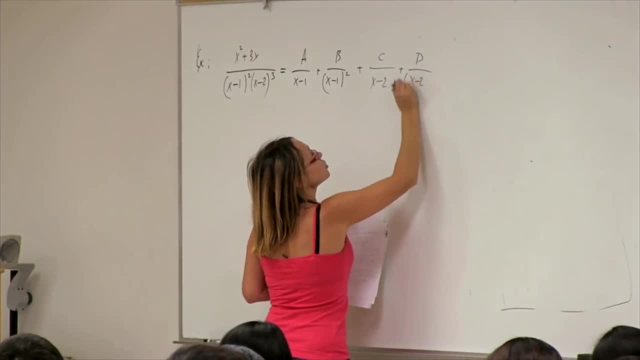 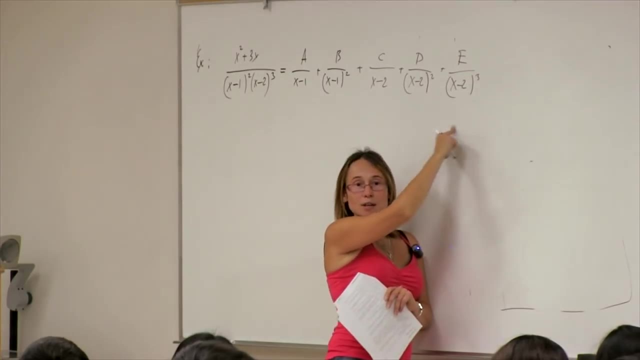 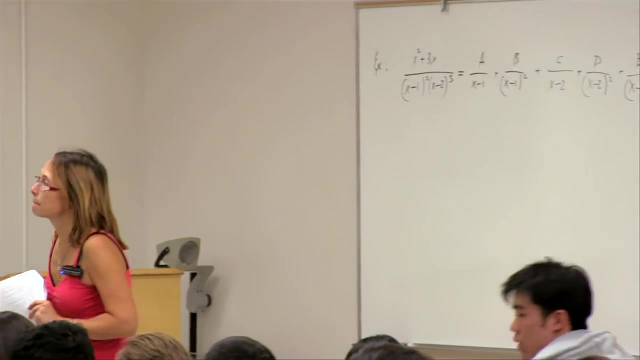 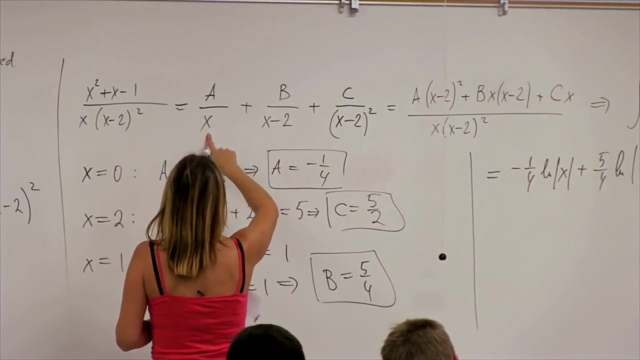 for x minus one. there are only two of them: plus c, x minus two. plus d, x minus two. three terms, uh, for x minus two questions: question this one: so the common denominator. uh, I have a factor of x in two of these. uh, so the common denominator? 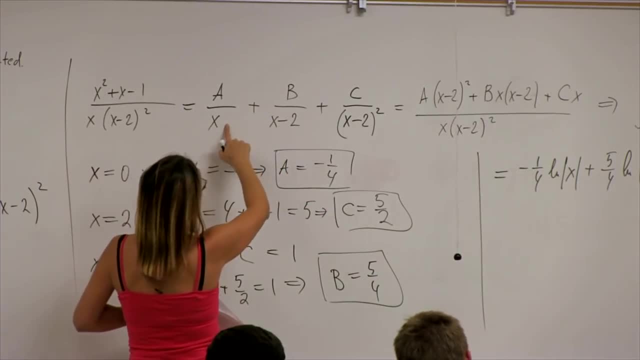 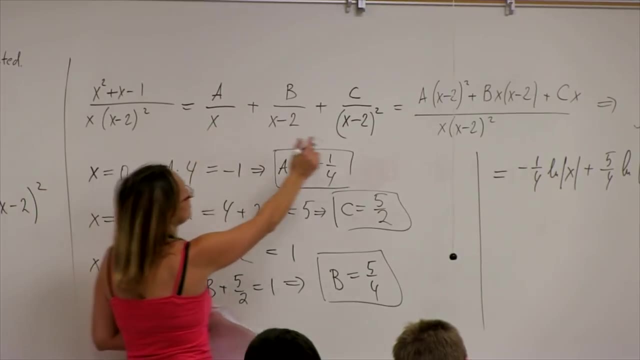 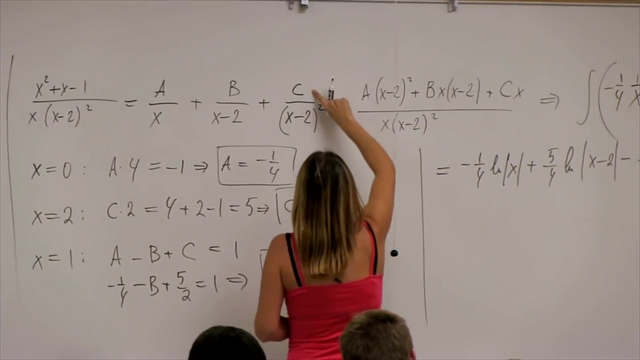 denominator is x times x minus two. so what? what is this one missing? it's missing x minus two, squared. right to right, there is this: this term is missing: x minus two squared. this term is missing one power of x minus two. and it's missing x and the last guy. 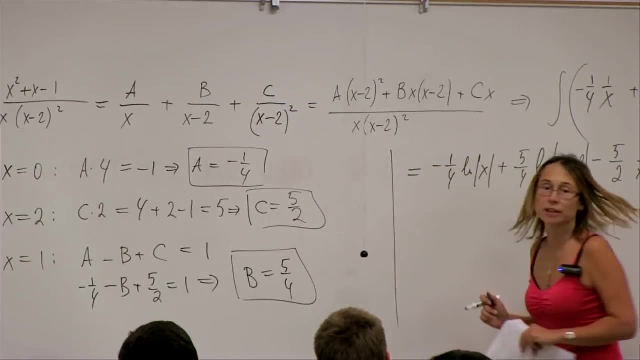 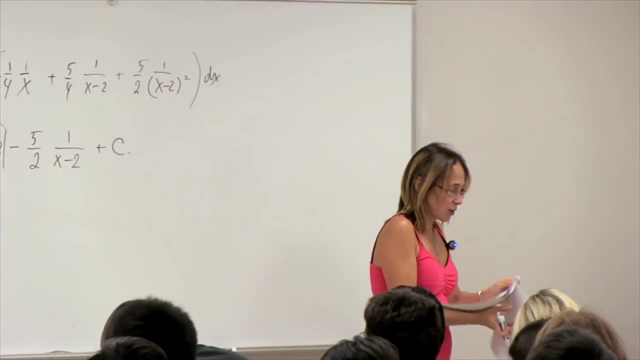 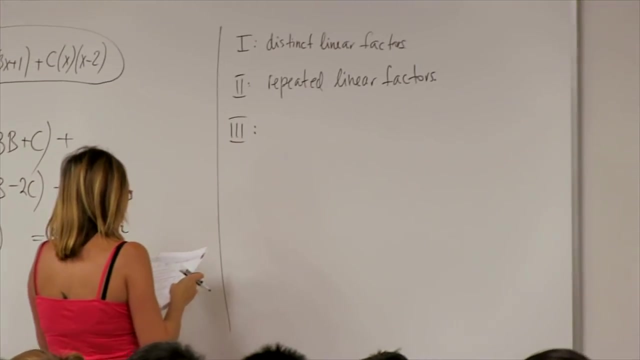 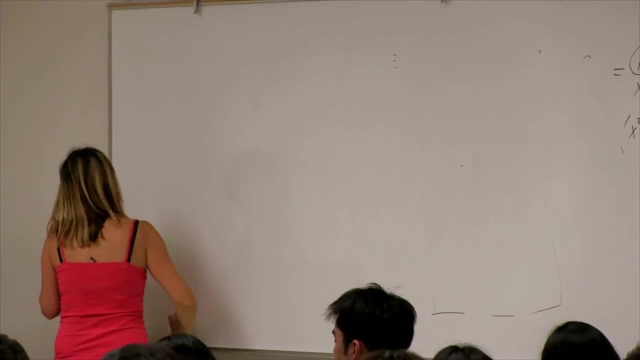 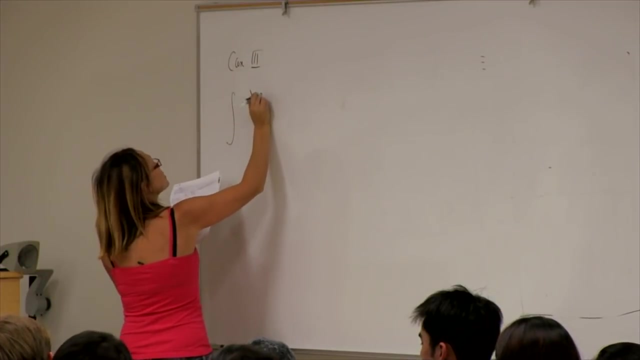 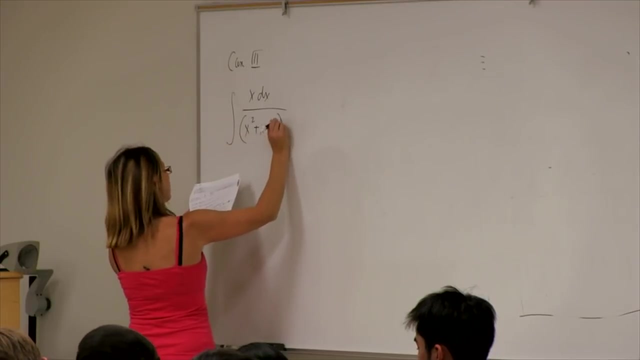 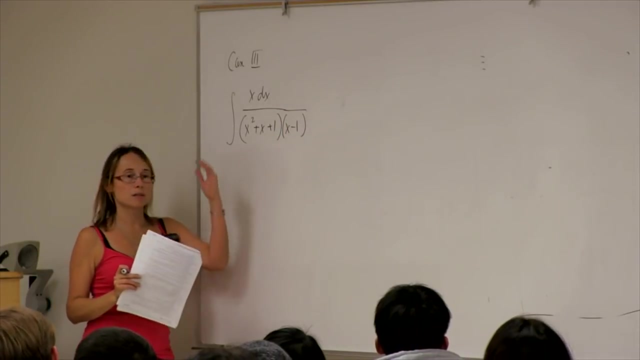 is only missing x. okay, so that's all. it gets more questions. okay, so it gets worse. uh, so case three, and let me start with an example. let's look at x, dx, x squared plus x plus one, x minus one. okay, what is this? it's a proper fraction. 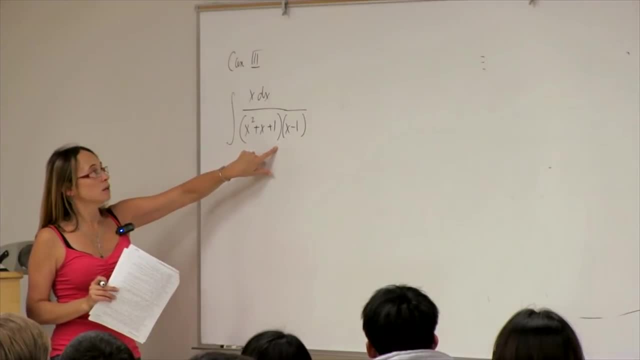 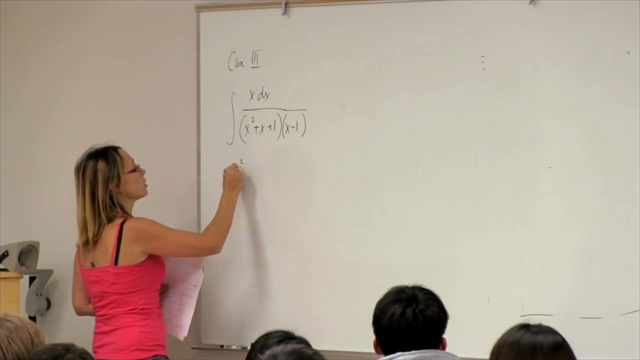 power one, power three, uh, and you can see that we have a linear factor here. so let's look for roots here to factor this one into two linear factors: x squared plus x plus one. so, as you can see, it has no roots, right, there is no value of x. 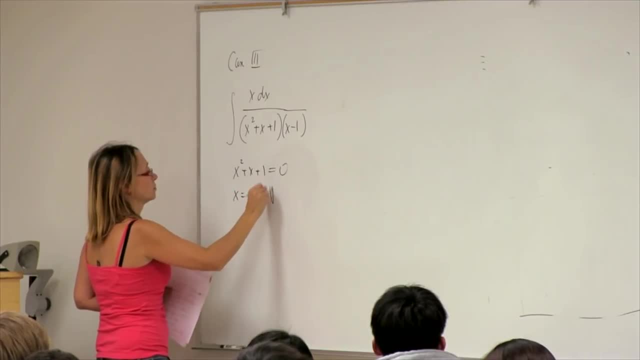 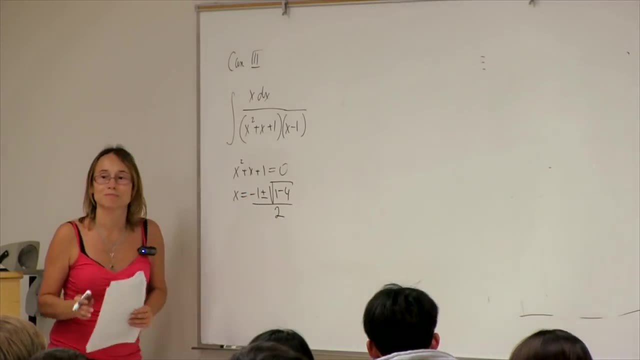 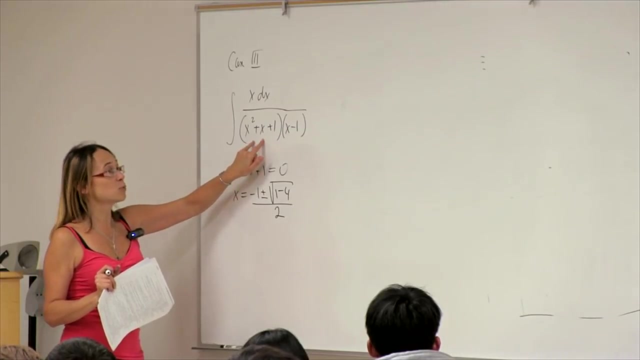 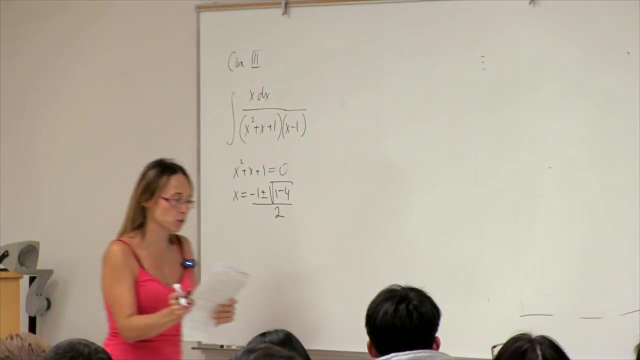 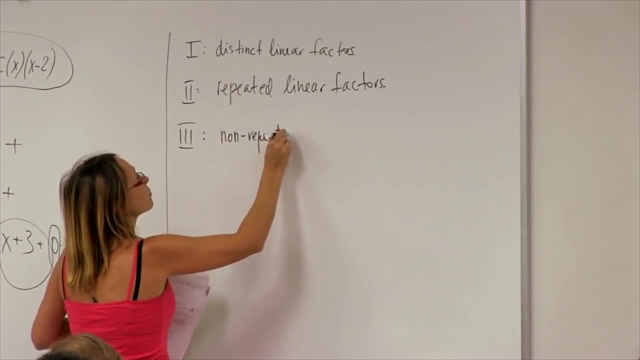 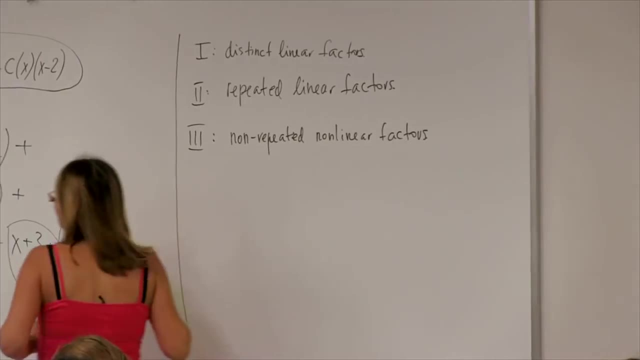 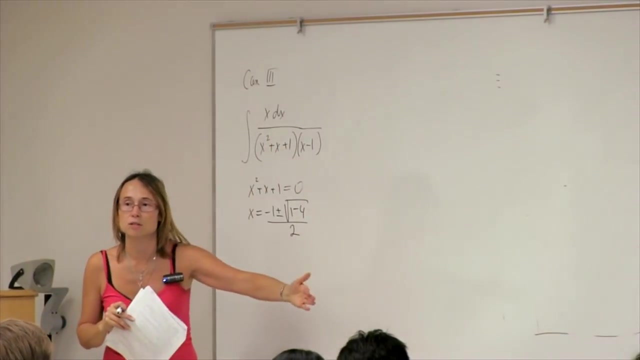 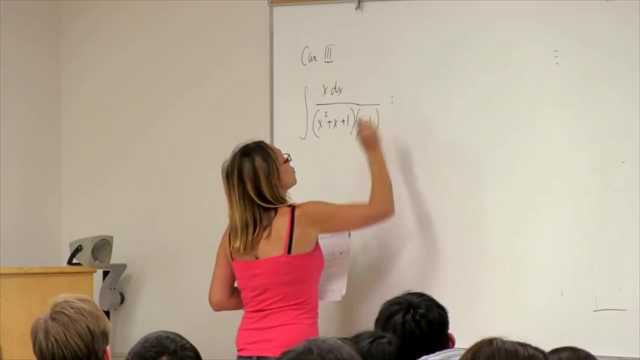 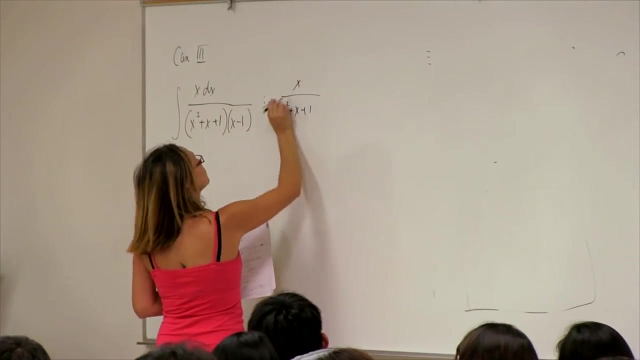 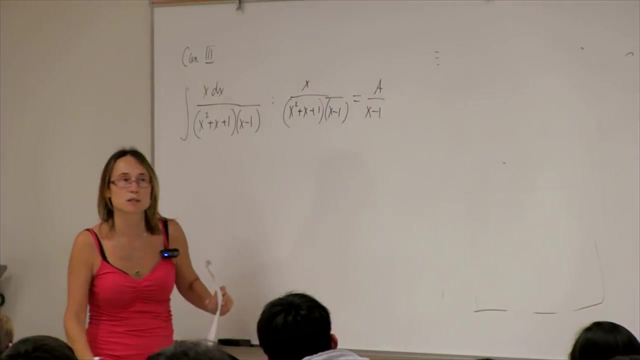 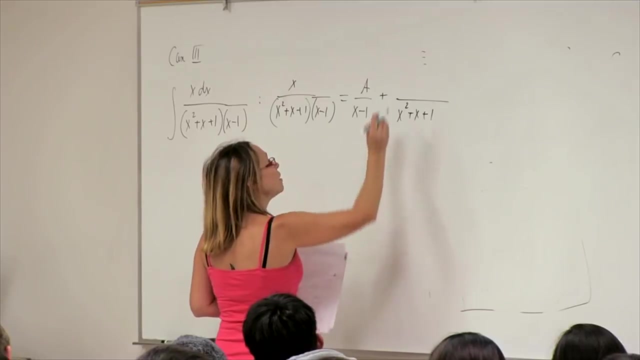 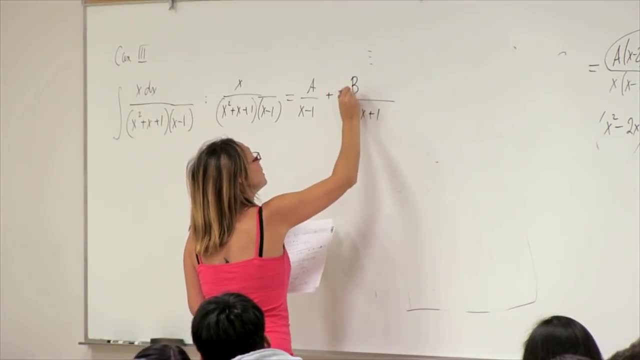 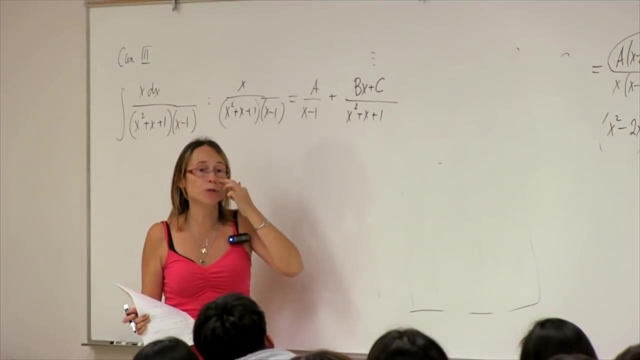 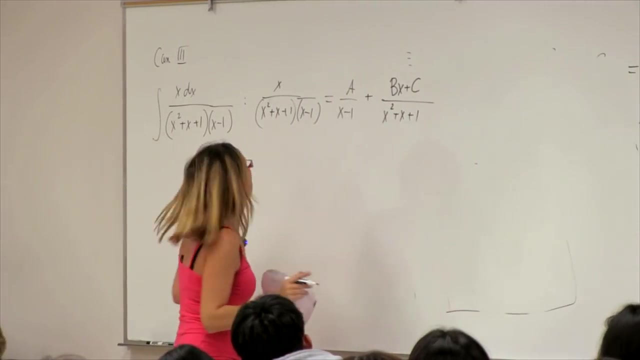 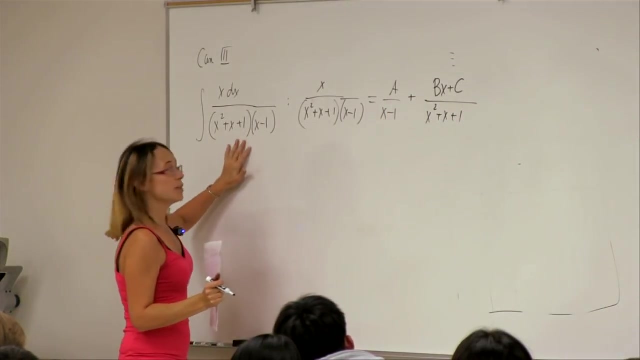 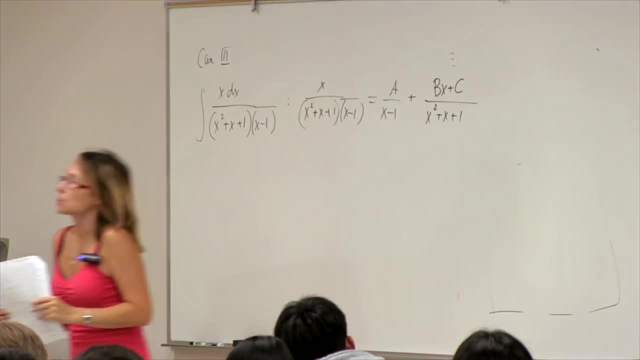 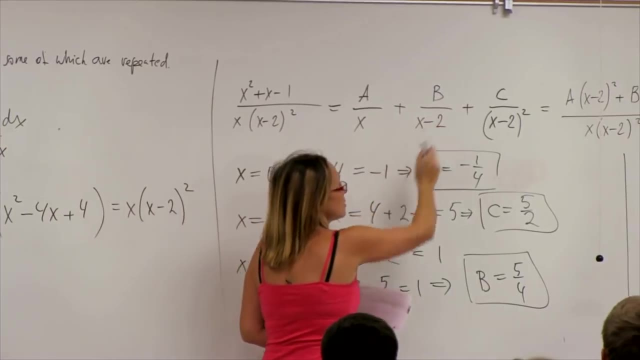 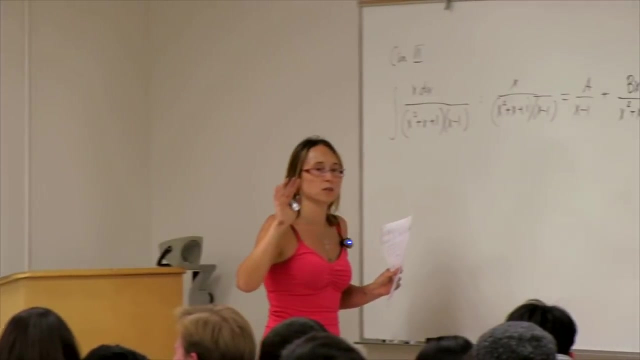 coefficients A, B and C Here. in the previous one, what did I have? Again, this was a third degree polynomial, so I have A, B and C. in the example I just erased there were two powers, two and three, so altogether it was five. so I had A, B, C, D, E. 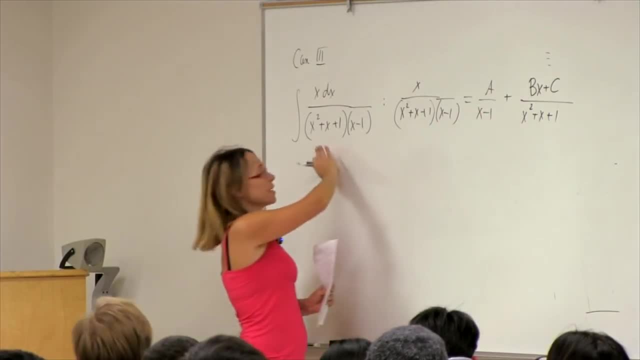 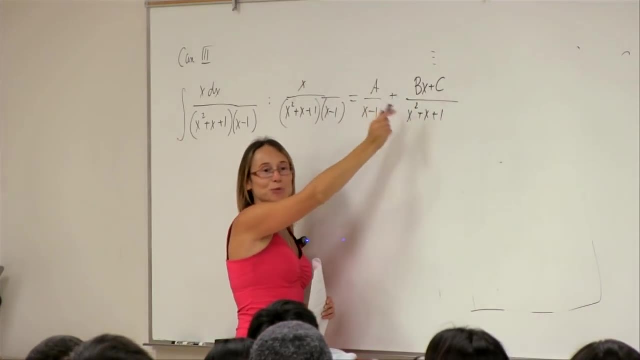 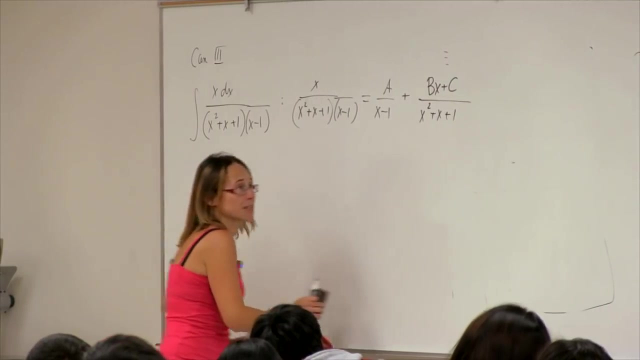 so the number of unknown coefficients has to coincide with the degree of the polynomial, and here, if I just had one constant here, I would only have two unknown numbers. I need to have three. so I make this a linear function. the rest follows the same algorithm, at least as far as 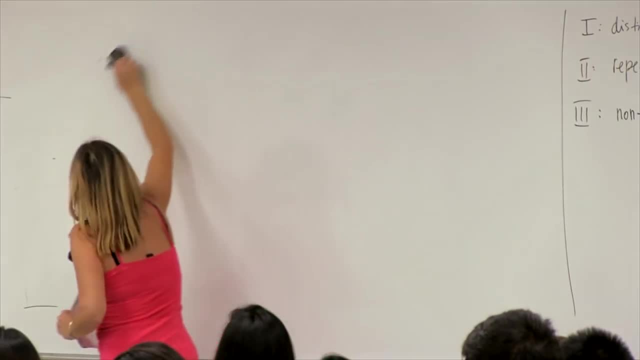 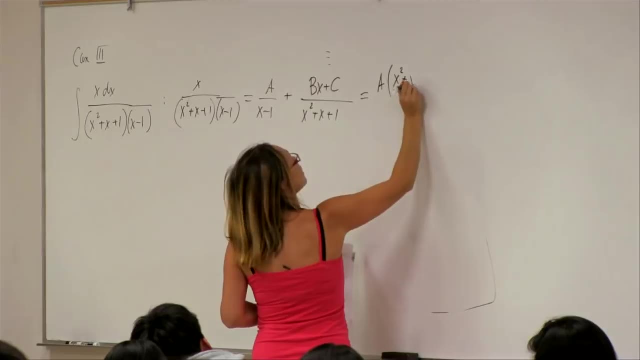 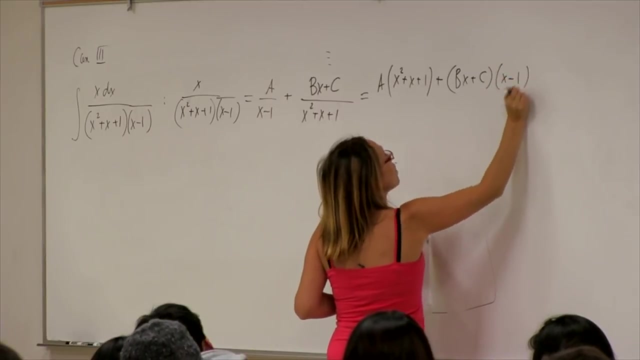 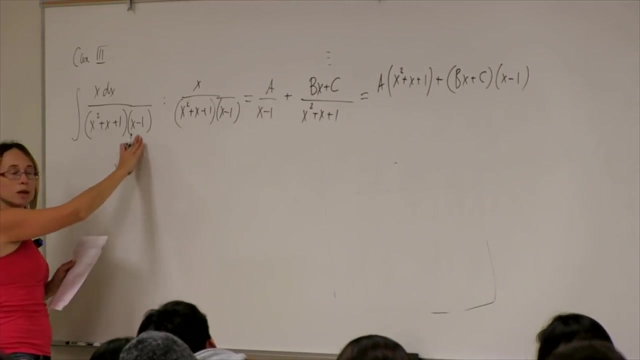 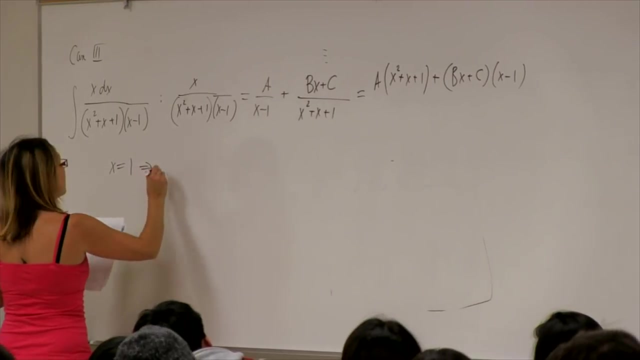 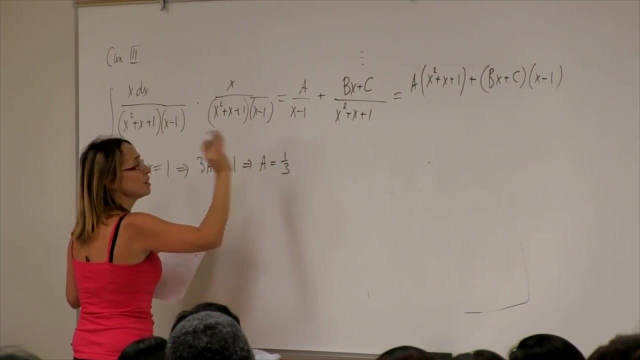 determining the coefficients goes. We have some meaning here. This is the next step, but for now we multiply it through okay, and we test some values of X. so one obvious choice is 1 and it kills this guy. so we have 3A and equals 1, so A is one third. 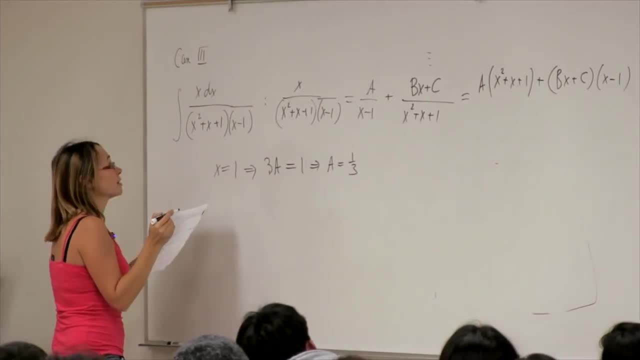 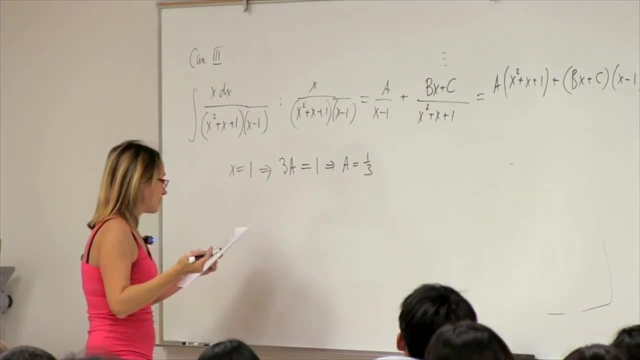 Linear factors are always very easy. okay, and that's it. No other roots, because this one, it, doesn't have roots. that's why it's not a linear factor. So what do I do? I take 0.. 0 is always a good choice. 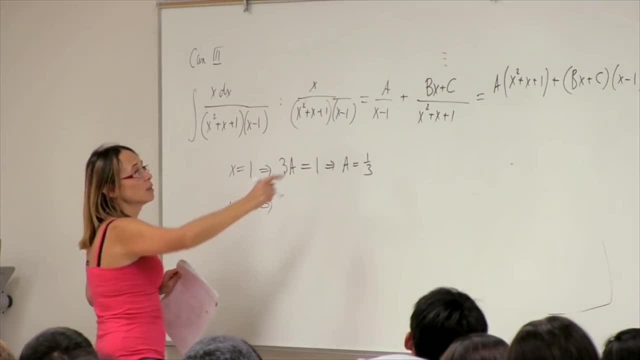 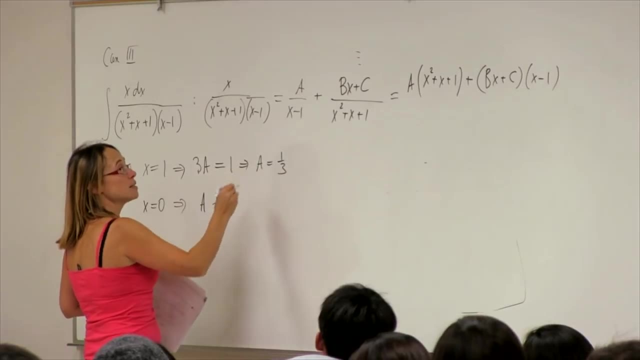 It makes everything simpler. so for A I have coefficient 1 and I have C and then C. So I'll do that. So for A I have coefficient 1 and then I have C, then 1.. times minus 1 equals 0. 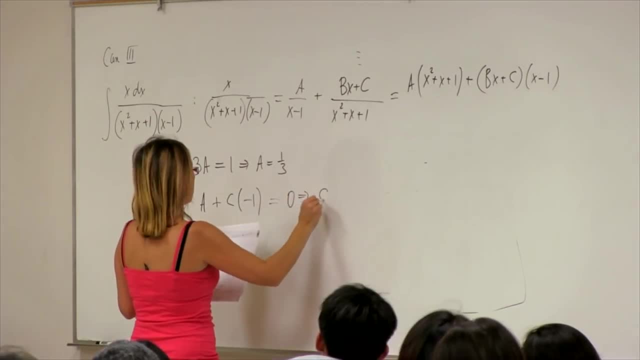 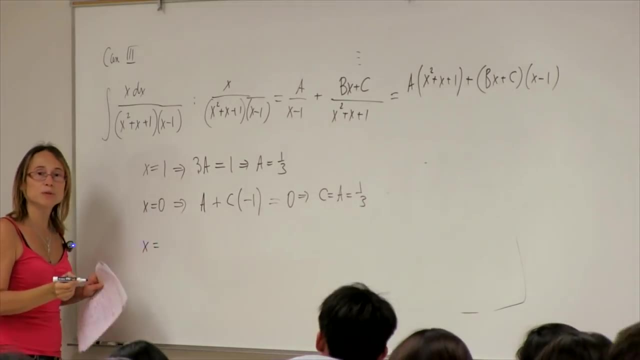 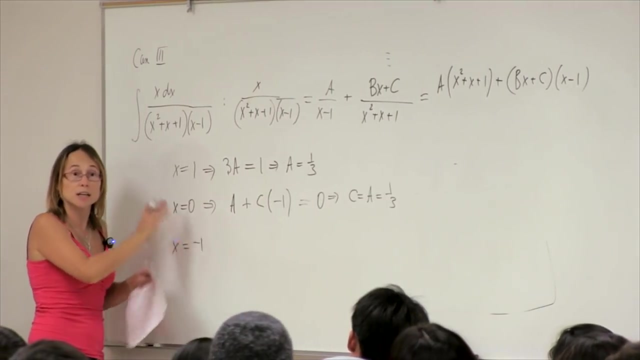 which means that C equals A is one-third, so I found C. it's easy. another choice, arbitrary but simple, is minus 1. you can take any other. you can take plus 173, if you like. it will give you the right answer, but the calculations will be. 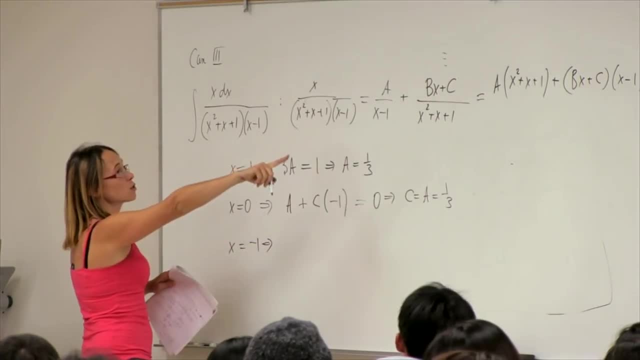 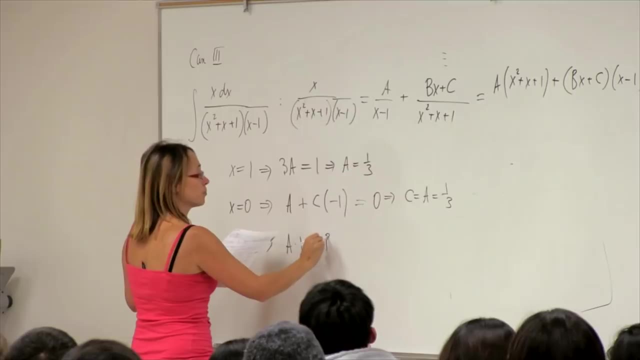 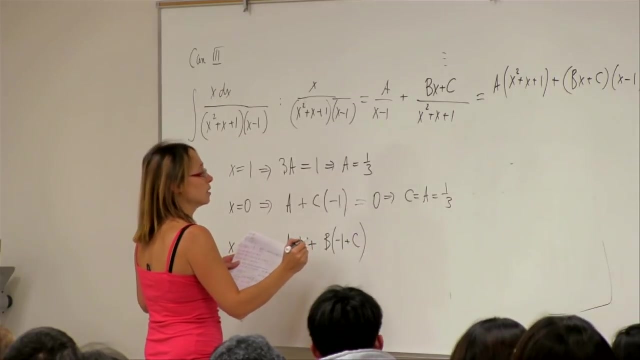 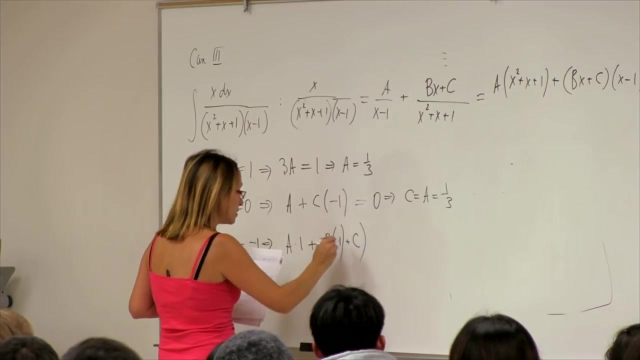 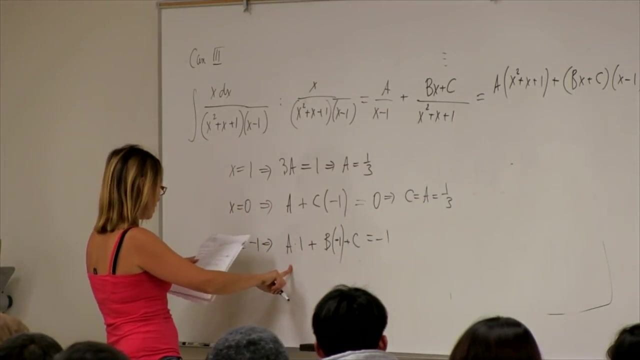 horrendous. so you try to do something simple. so with minus 1 I have A times 1 plus B, minus 1 plus C. okay, minus 1 plus C equals minus 1. so I already know A and C one-third minus B plus one-third. 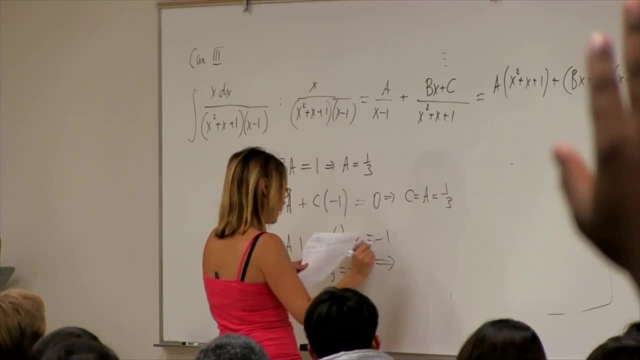 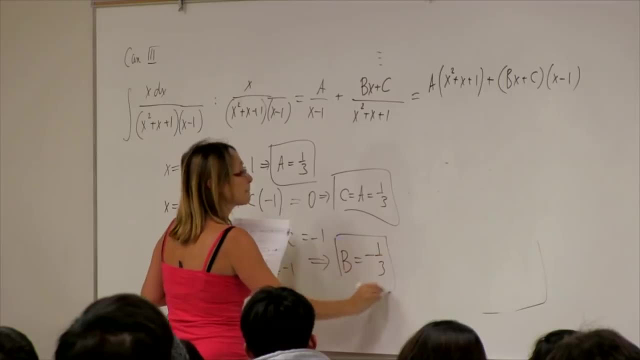 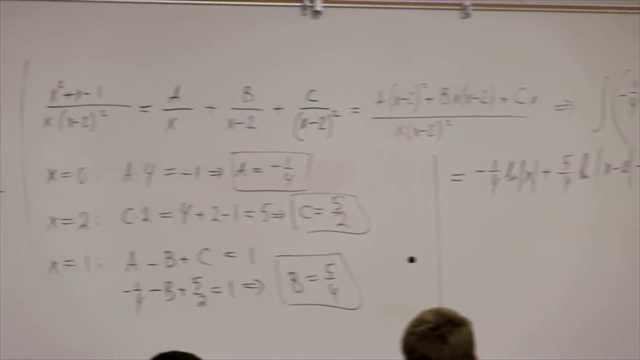 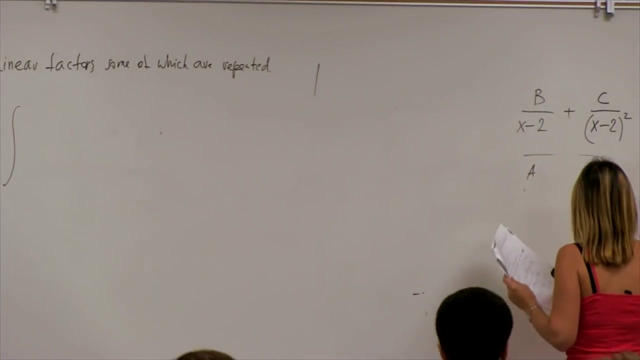 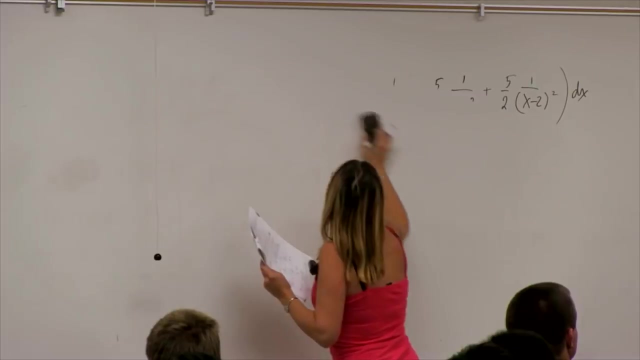 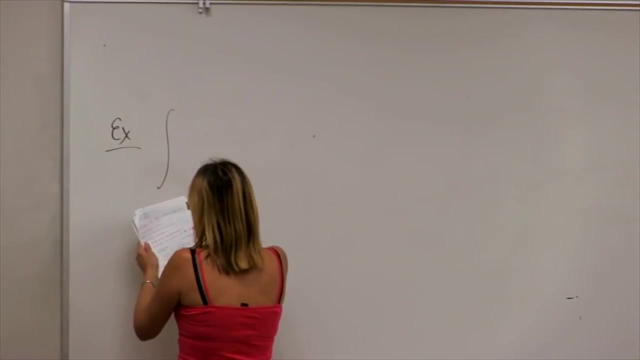 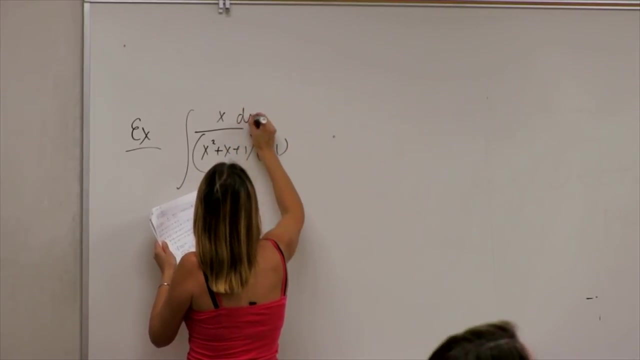 equals minus 1. I can solve this. hopefully it gives me B equals minus one-third. so I found all the coefficients and I can rewrite my integral in a simpler form. so let's do that. so X squared plus X plus 1, X minus 1 becomes equal one-third. 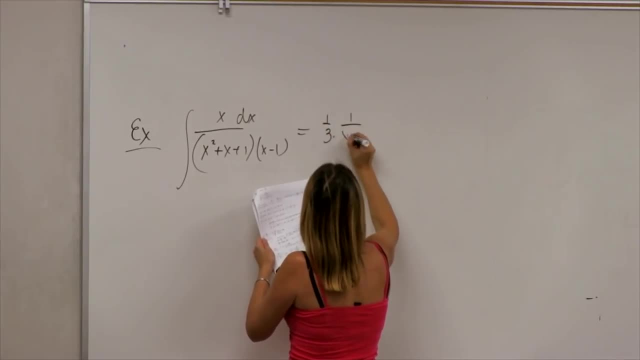 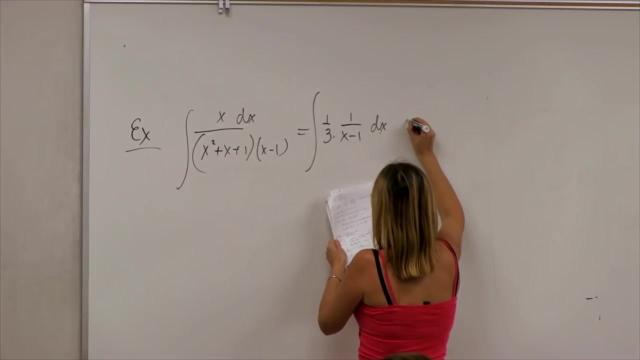 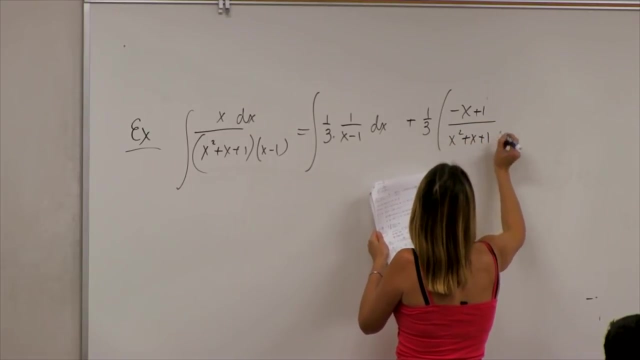 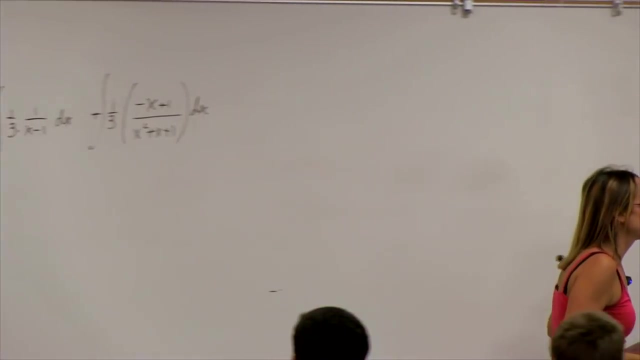 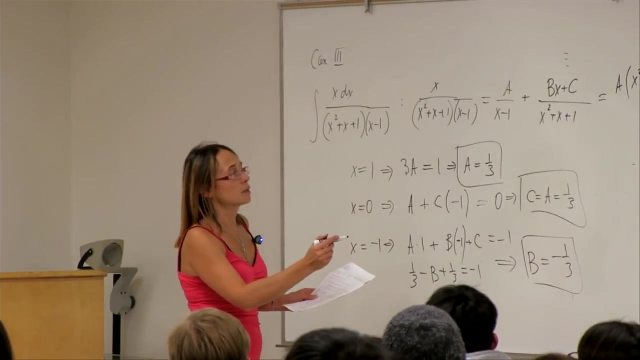 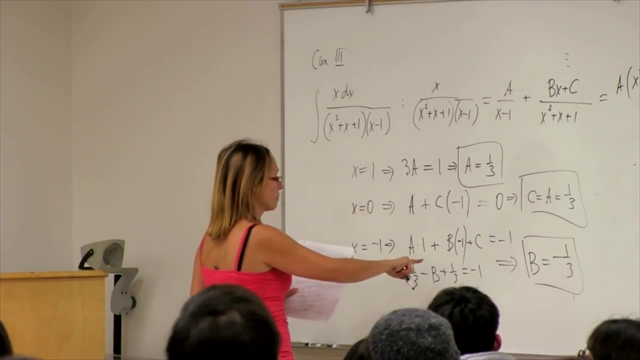 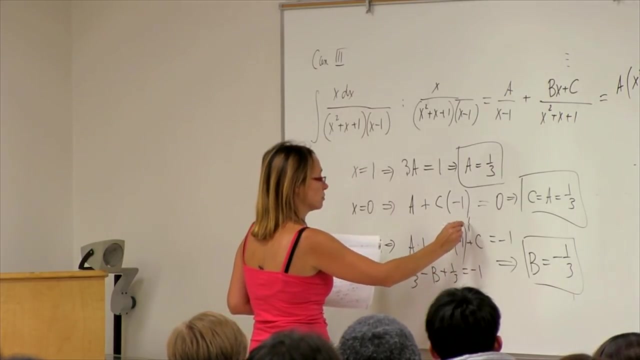 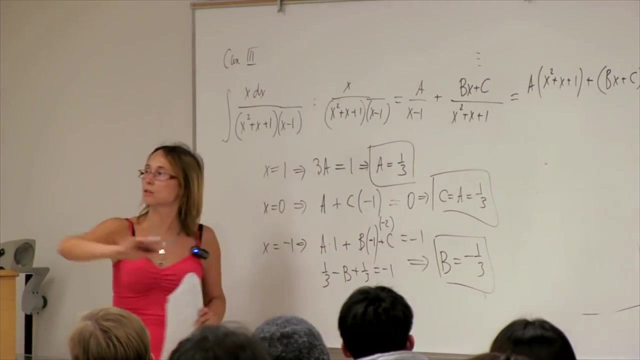 X minus 1, DX plus B, DX. okay, so these are my two terms question. I think you missed last part of C of the X minus 1. I missed. so yes, minus two. okay, so the answer is probably correct and it's probably a typo. let me know if this isn't correct. if the answer isn't. 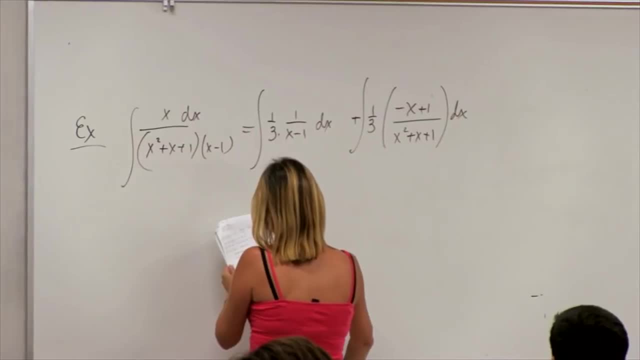 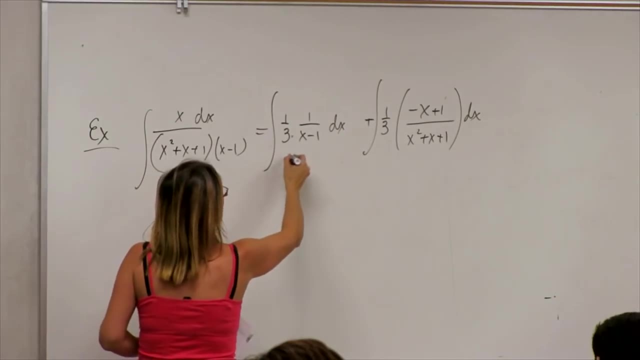 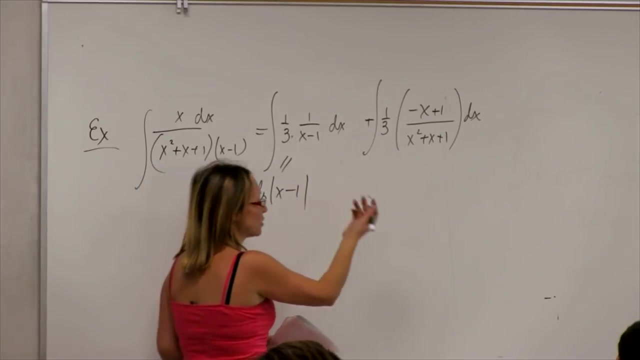 correct, okay. so what do we deal with here? this is known. we know exactly what this is. we're going to do them step by step. so this is 1, 3rd log X minus 1, and we don't have to worry about this until until we arrive at the final answer now. 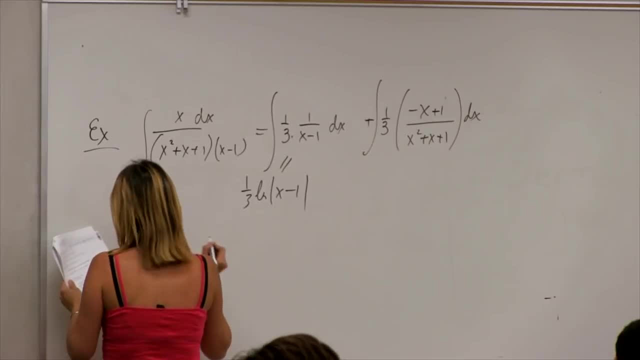 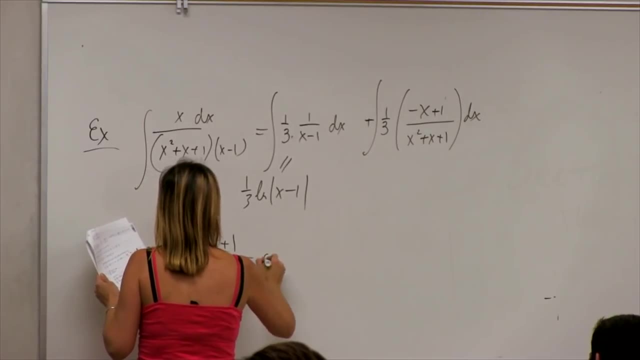 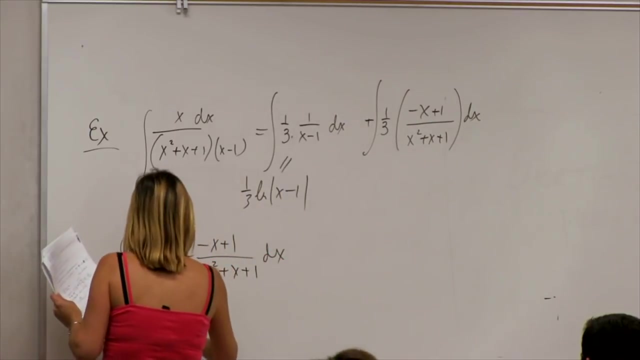 consider this integral: minus X plus 1 X, squared plus X plus 1 DX. okay, so this is the hard, the harder one. it's still doable. so one way of doing it is to use substitution. so I suggest we take you to be equal to this whole denominator X. 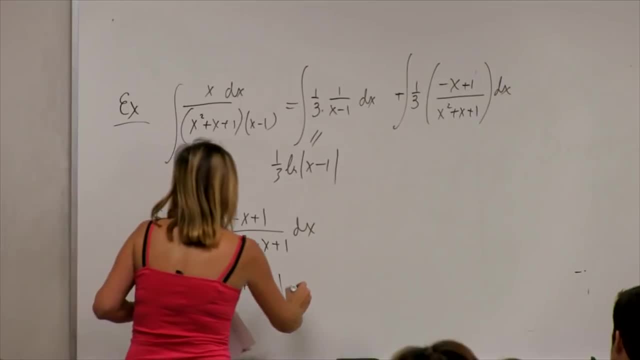 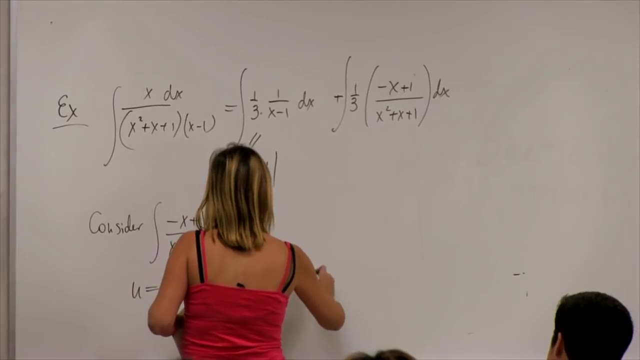 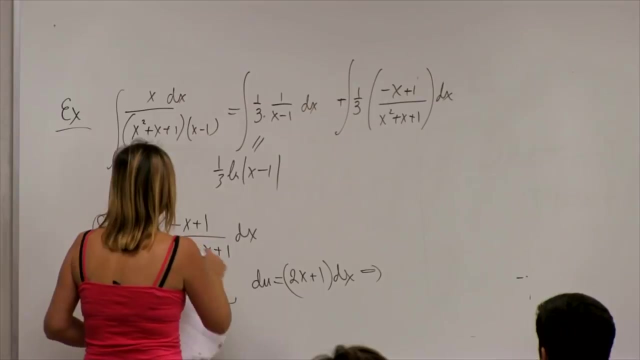 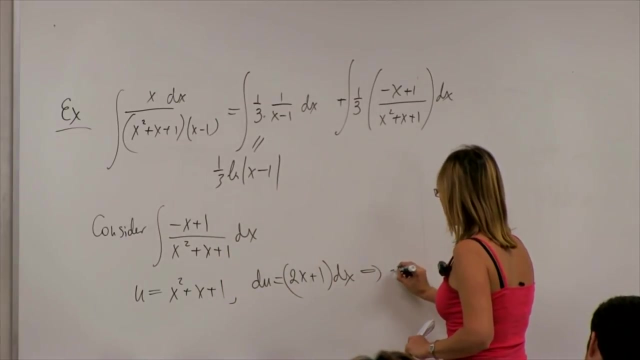 squared plus X plus 1, okay, and we immediately calculate DU. so 2x plus 1, DX, and what I want is minus X plus 1. what I get is 2x plus 1. so let's multiply it by minus 1 half, so minus 1. 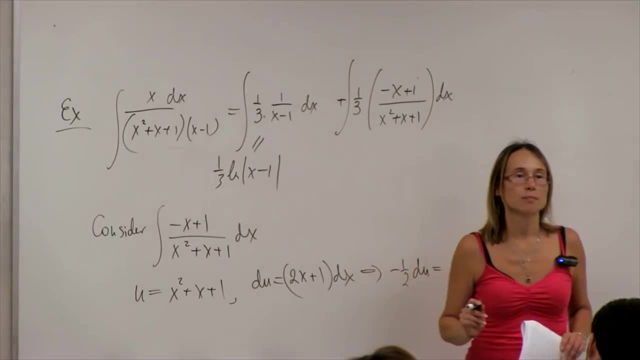 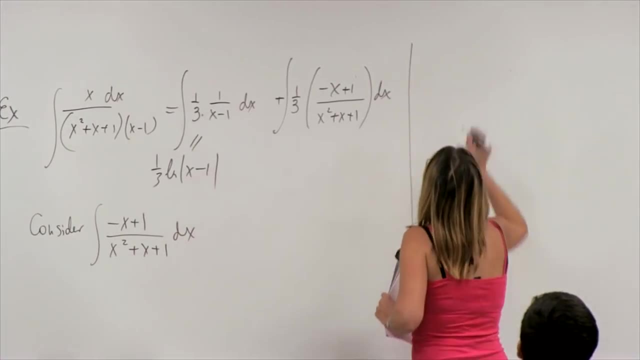 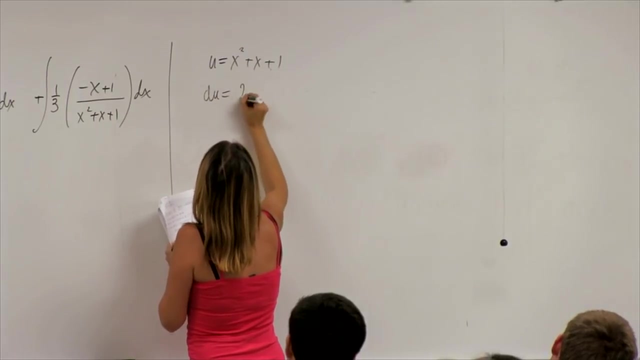 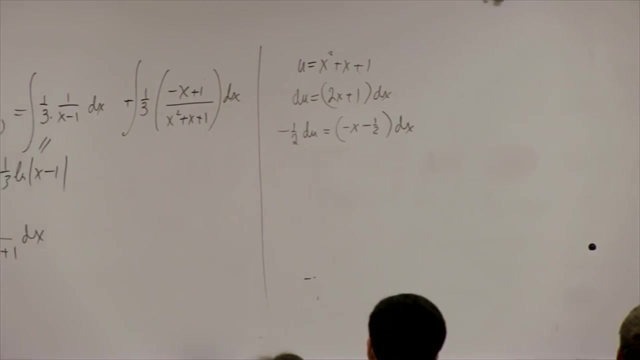 half DU question. oh, I'm sorry. yes, so you is X squared plus X plus 1, 2x plus 1 DX minus half DU is minus X minus 1 half DX. I'm trying to obtain minus X plus 1 for my differential and I'm 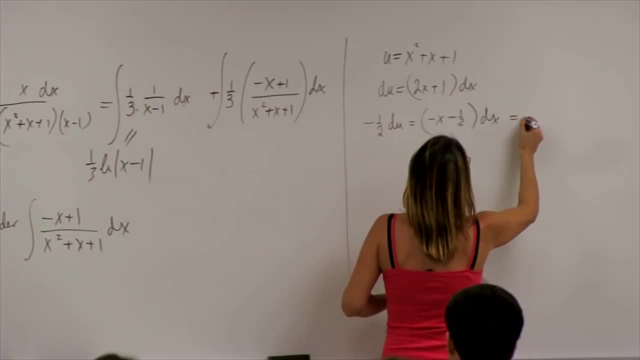 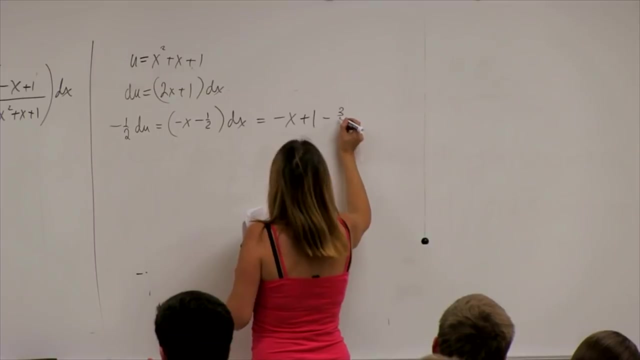 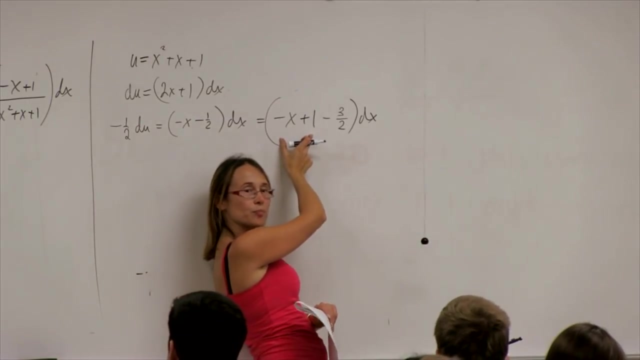 failing a little bit because I have minus X minus 1 half. but I can do this. I can say minus X plus 1, minus the 3 halves DX. so I have the part that I want and they have an extra constant factor, right? so what does this? 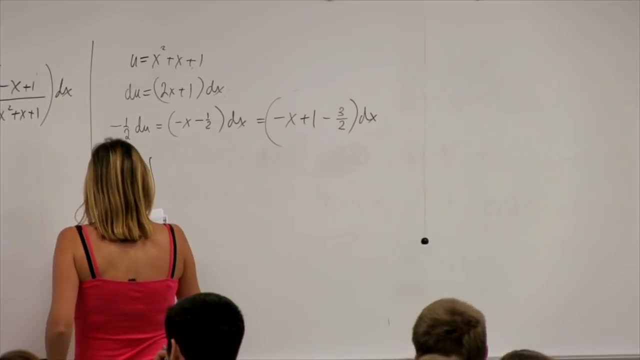 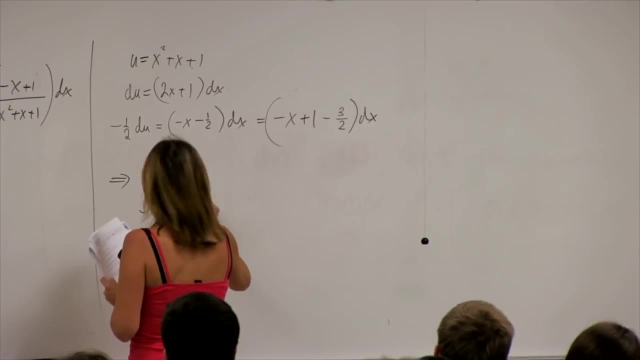 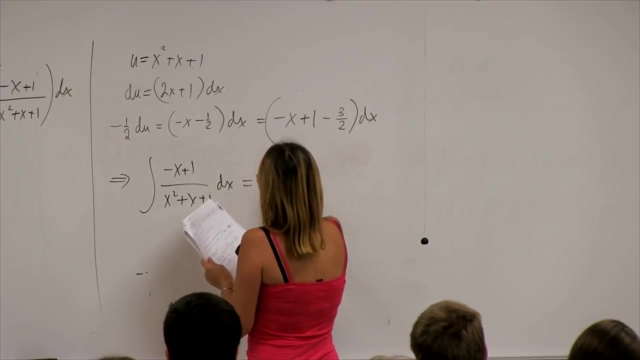 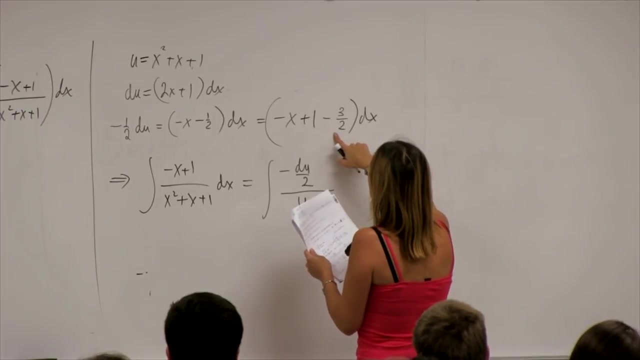 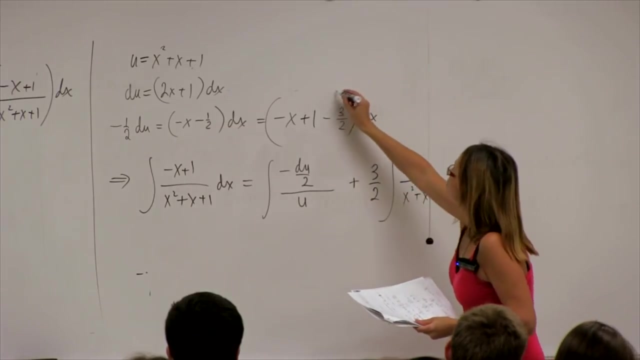 give me: I have minus X plus 1, X squared plus X plus 1, DX equals minus a half 2 divided by you. okay, and I have plus three halves DX, X squared plus X plus 1. so this part goes here and this part comes here. 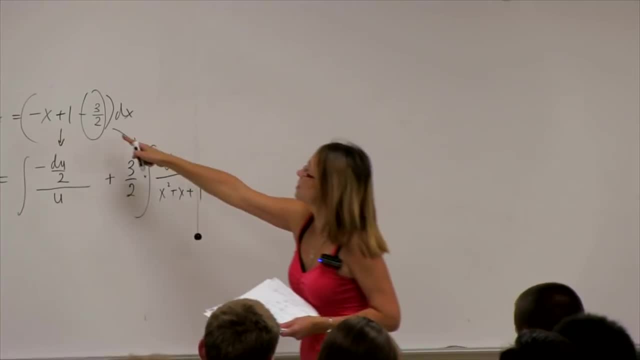 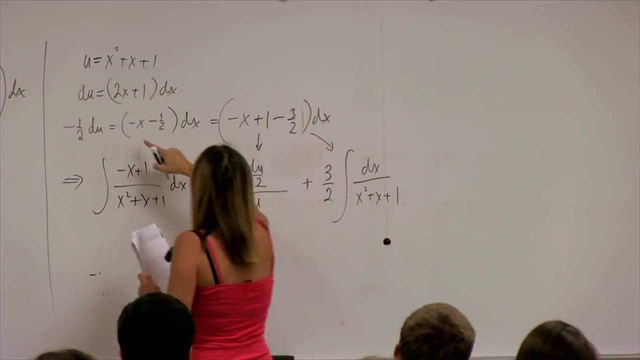 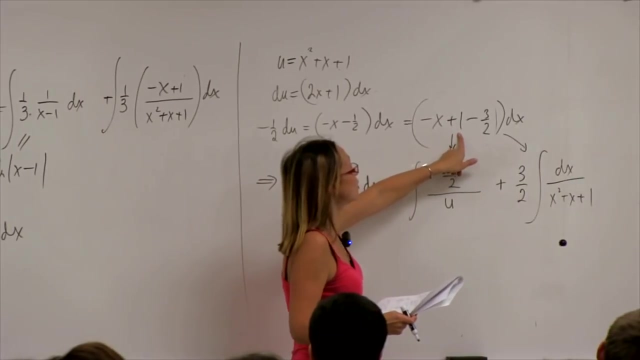 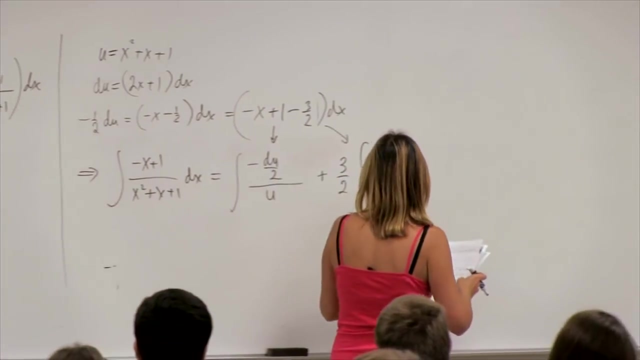 question this: so I have minus X minus 1 half and I want minus X plus 1, so I'm forcing it to be minus X plus 1, but as a price that I pay I have to subtract minus 3 halves, so it's kind of forcing it to be what it. 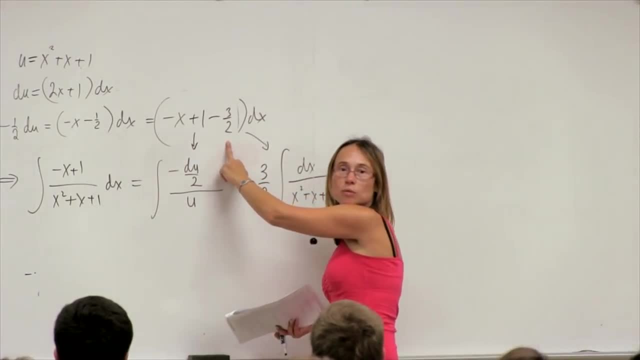 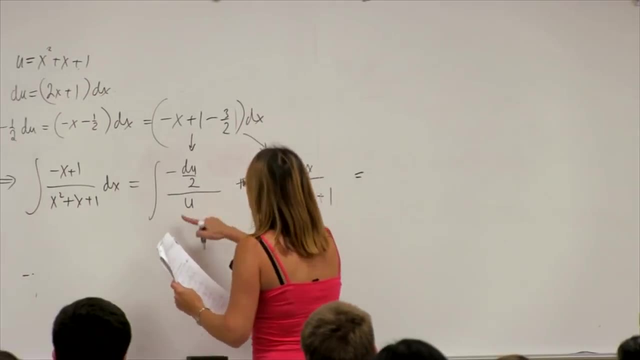 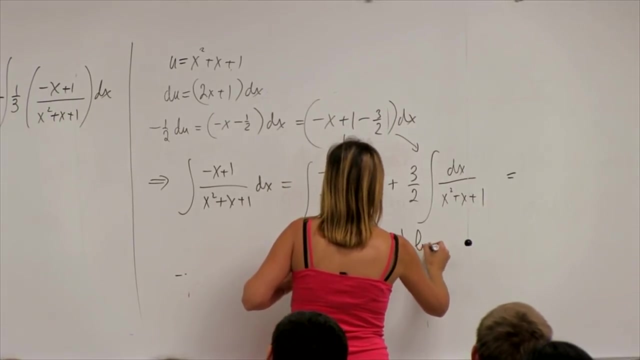 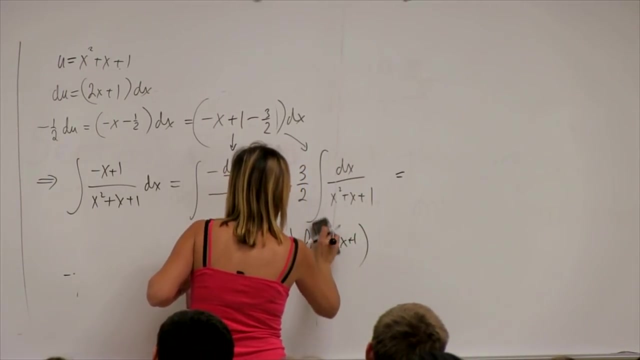 should be, and then paying the consequences by having this extra term. so, and let me do these two separately. this one is really easy: minus 1 half log of u is minus 1 half log of this whole thing: X squared plus X plus 1. actually I can forget the absolute value because this guy is. 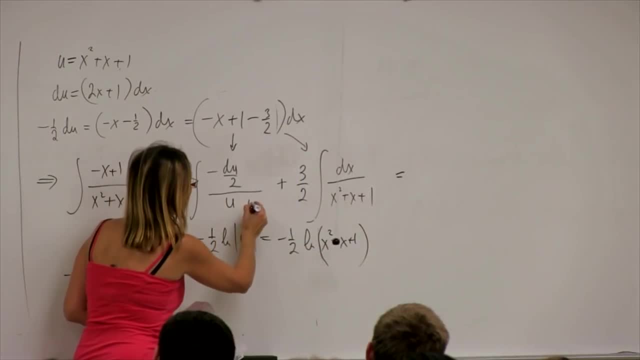 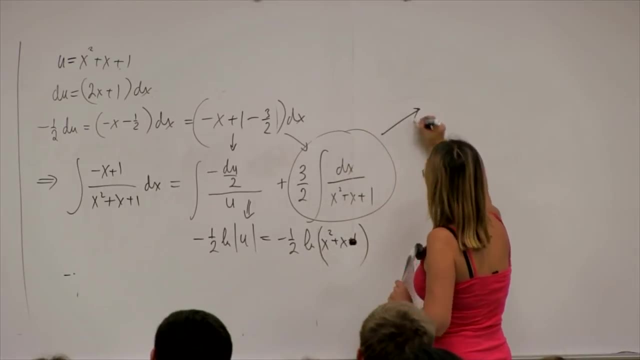 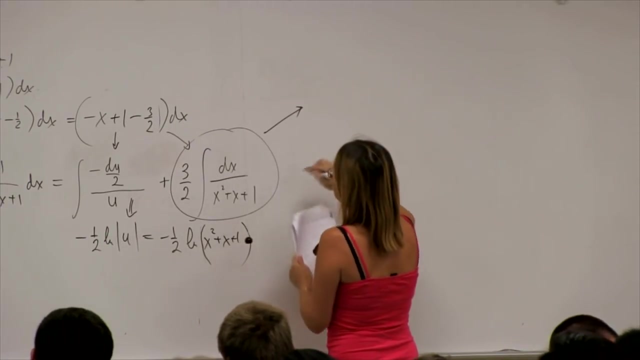 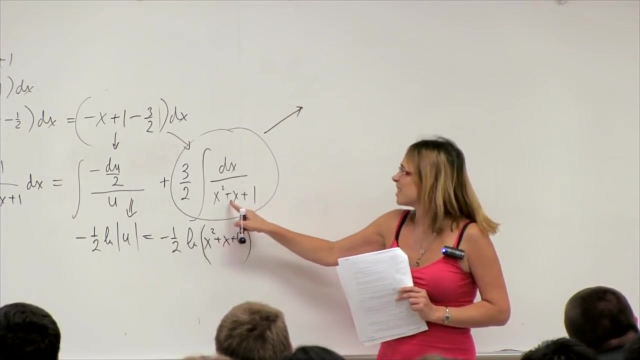 always positive. ok, so this is very easy to take. how about this term? so with this one, I can recognize it as something that that looks like the antiderivative of the arctangent, for the arctangent remains. Remember I have to have x squared plus 1.. 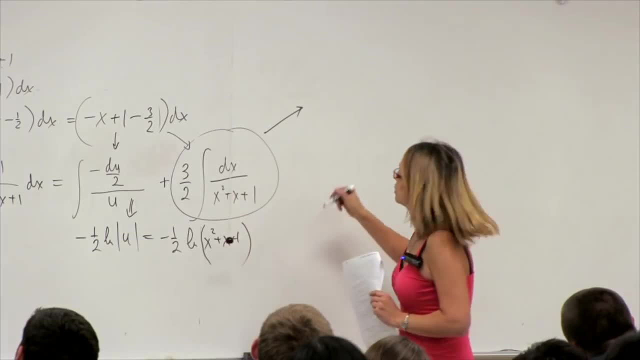 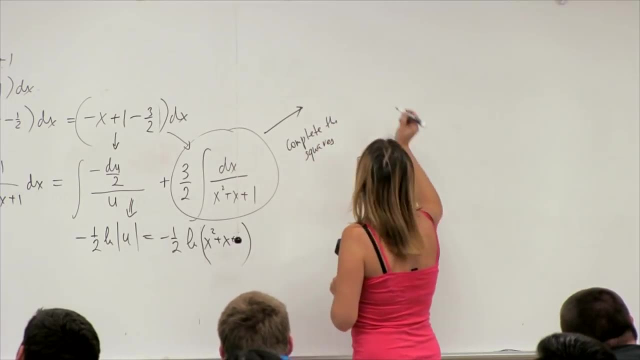 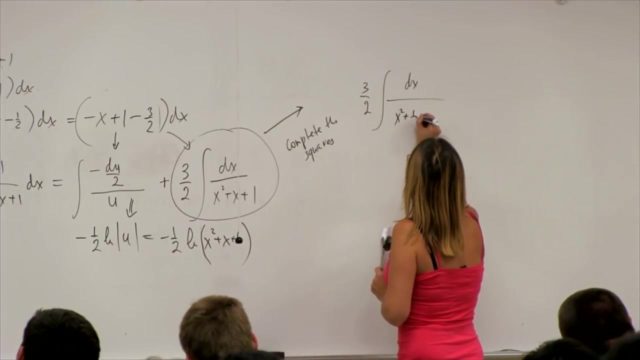 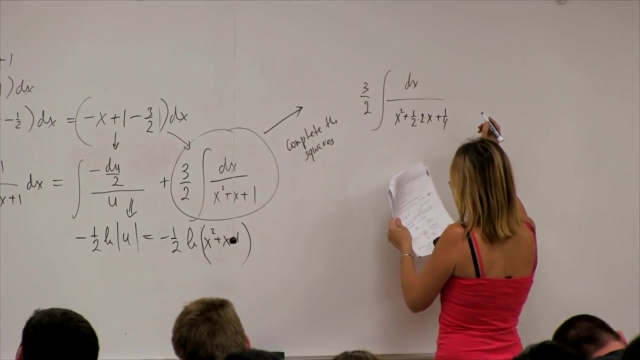 Here I have something else plus 1.. So I have to complete the squares. So complete the squares. So I have 3 halves dx and here I have x squared plus 1, half times 2 times x plus 1 quarter plus. what is missing is 3 quarters. 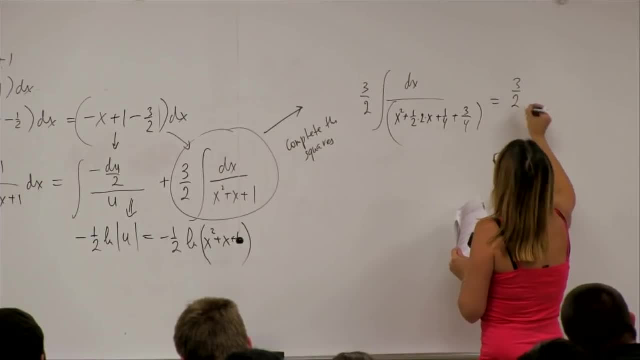 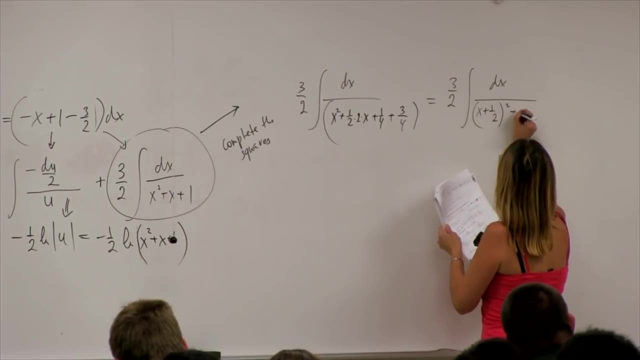 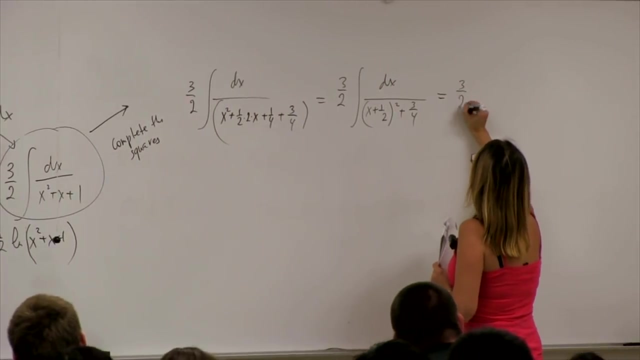 I complete the squares in the denominator 3 halves dx, x plus 1 half squared plus 3 quarters completing the squares. Now I want this to be 1.. So I go 3 halves dx and I take out 3 quarters here. 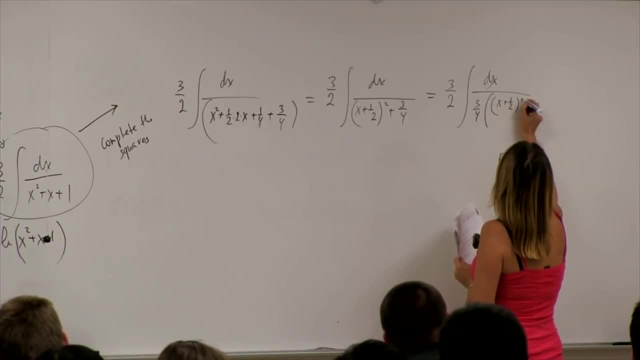 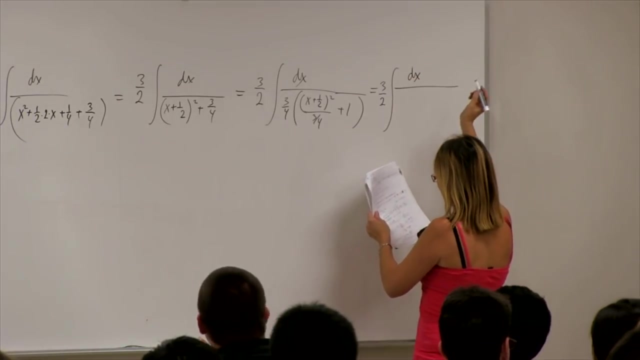 And I get x plus 1, half squared, divided by 3 quarters plus 1.. So now this guy is going to be my new variable. Square root of this is going to be my new variable. One more step: 3 halves dx, 3 quarters. 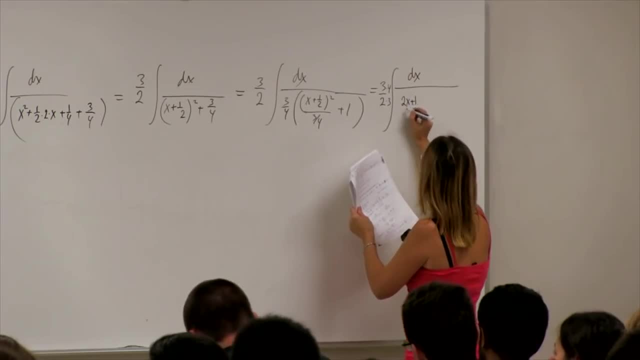 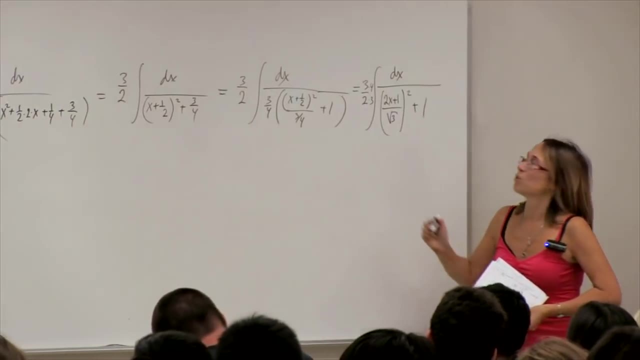 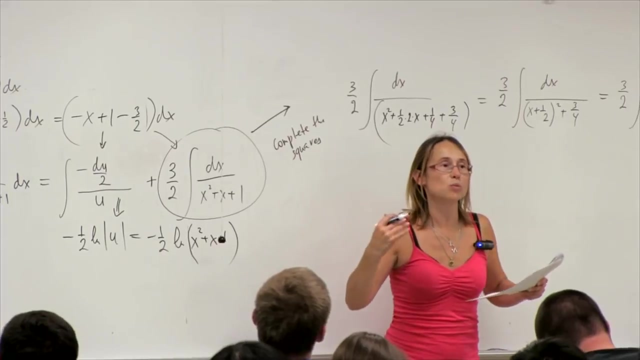 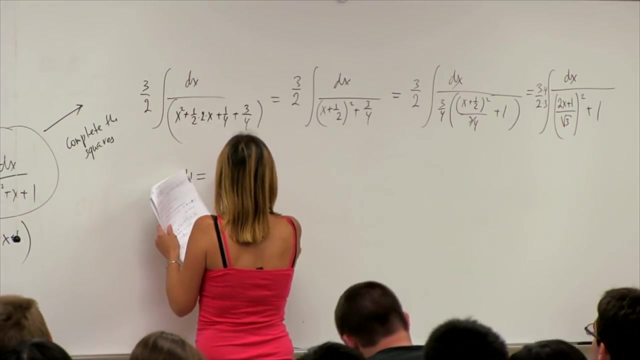 And here I have 2x plus 1 over square root of 3. 1. 1. Squared plus 1.. So this is the same as the original one, where I factored out a full squared plus 1.. And now you can see that the substitution u to x plus 1 over square root of 3 gives me: 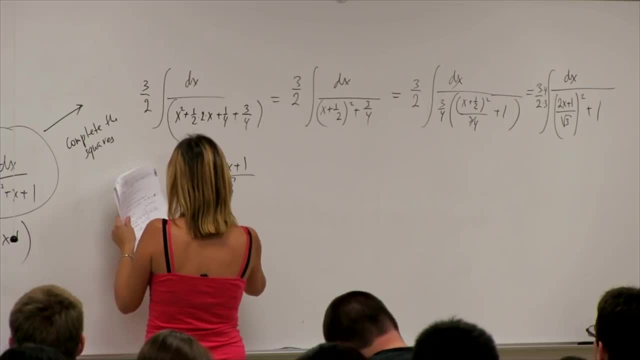 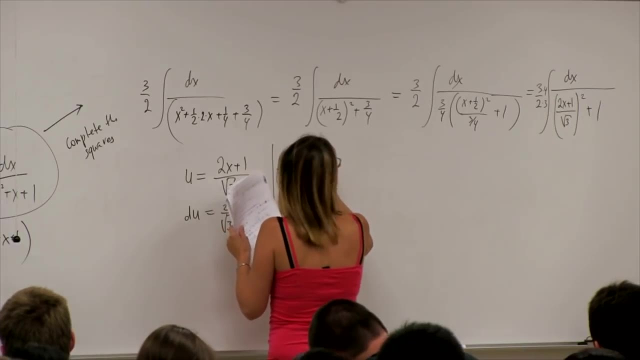 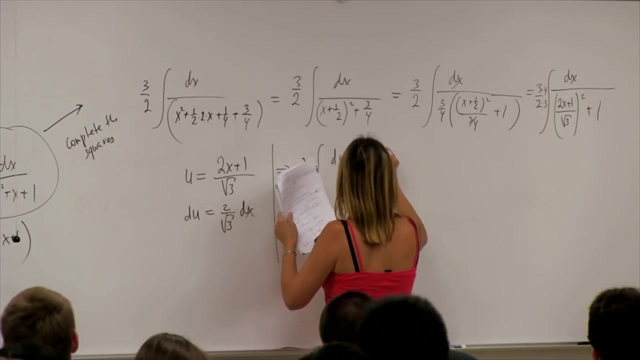 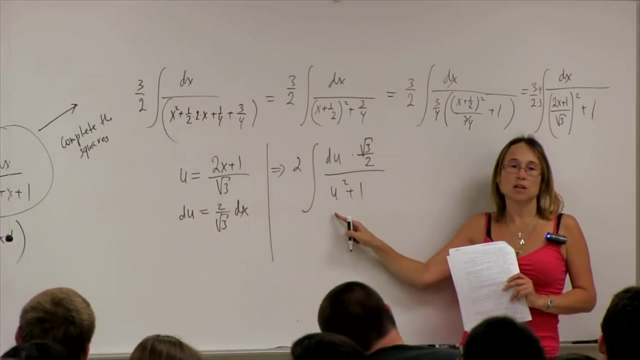 the desired shape. So du is 2 over square root of 3.. dx, so I get 2 du times squared of 3 over 2 u squared plus 1. you can see that now it really is an antiderivative of the arctangent and 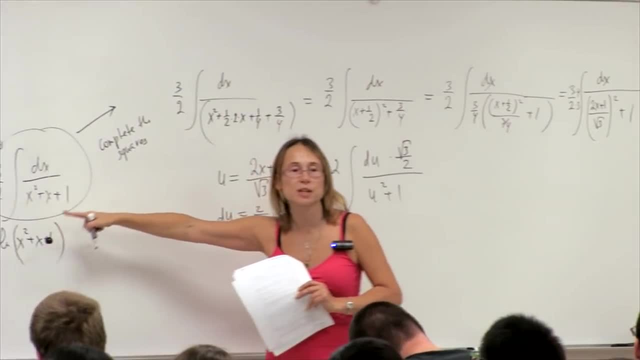 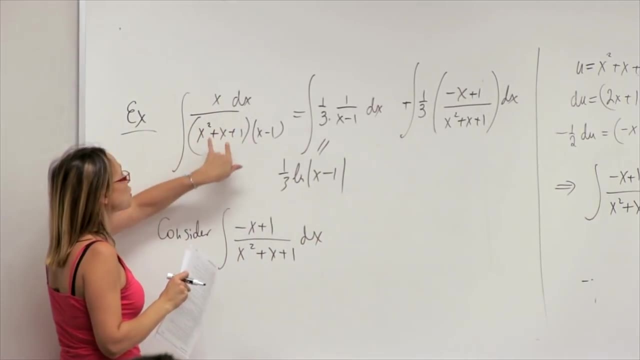 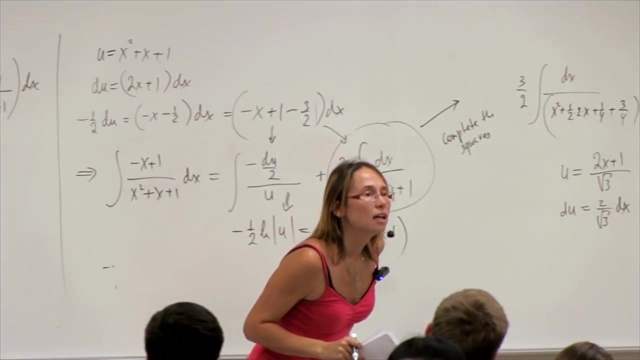 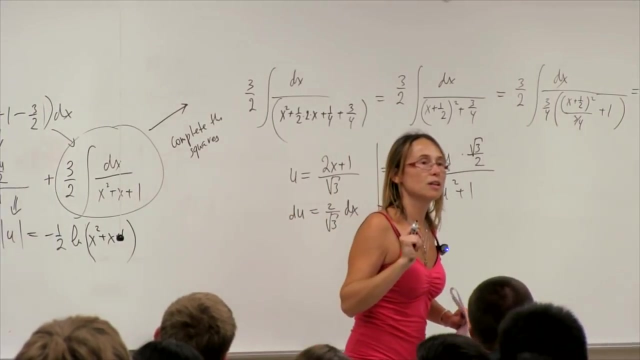 this is what I have to recognize from here, and such examples come up all the time for case 3. so I have to integrate something like a constant divided by this irreducible quadratic factor. I come here: 2x plus 1, half this one. 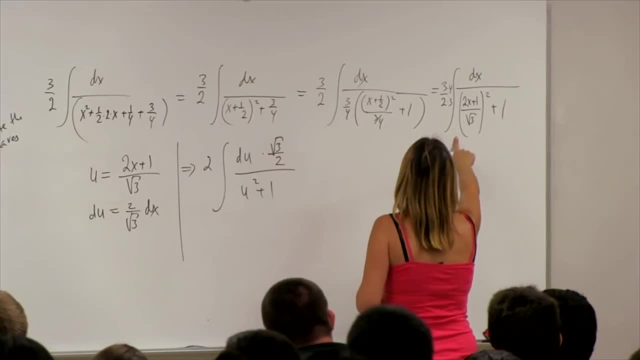 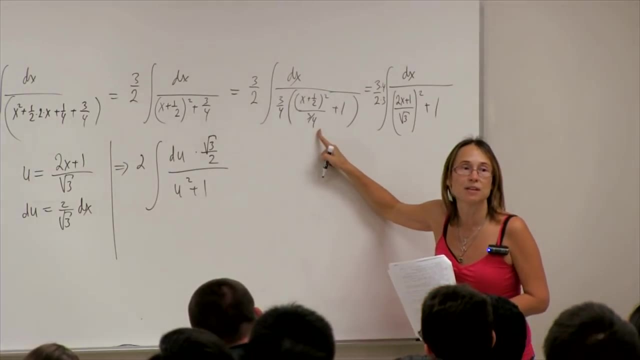 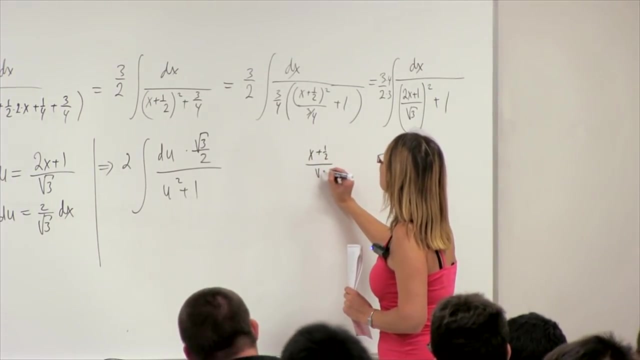 how do you do this? this one, okay I. I had to present this as the square of something, so I had to take the square root of this. what's the square root of this? it's x plus 1, half divided by square root of 3 times 2. 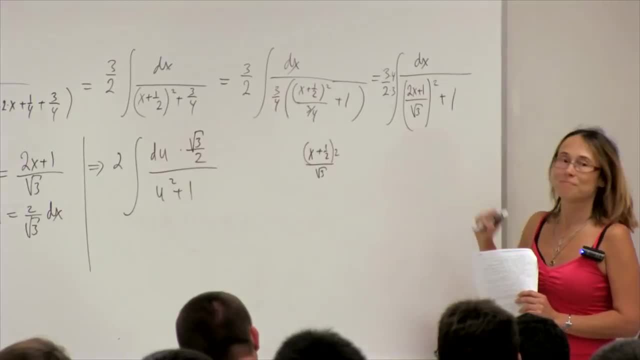 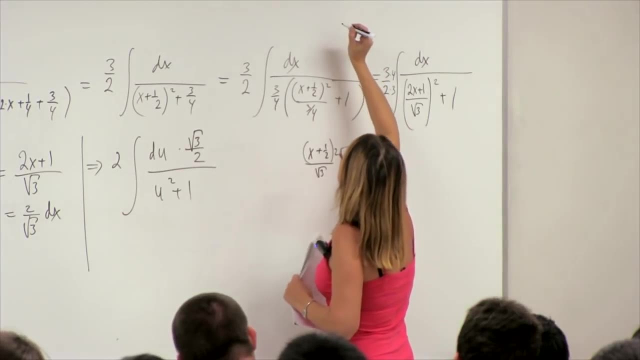 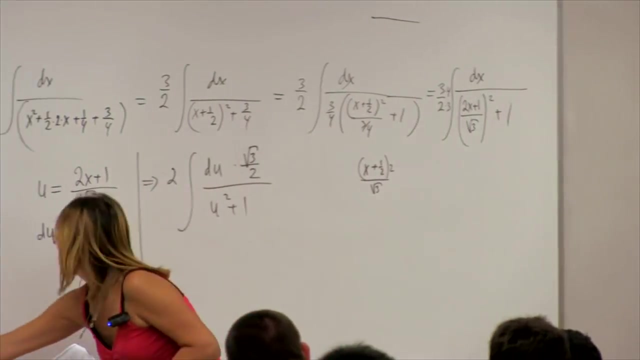 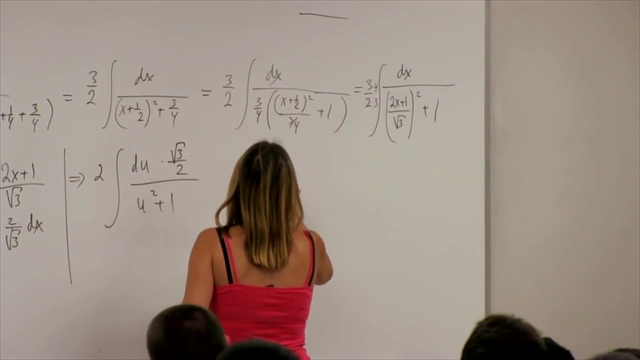 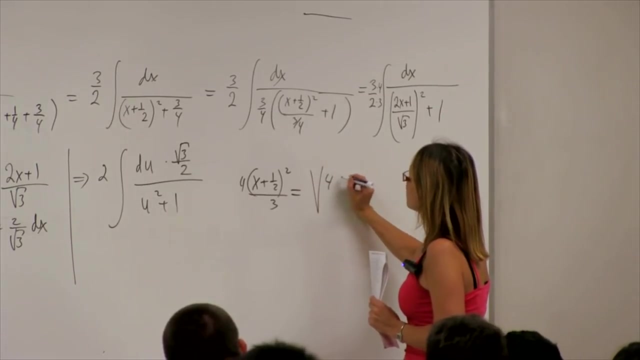 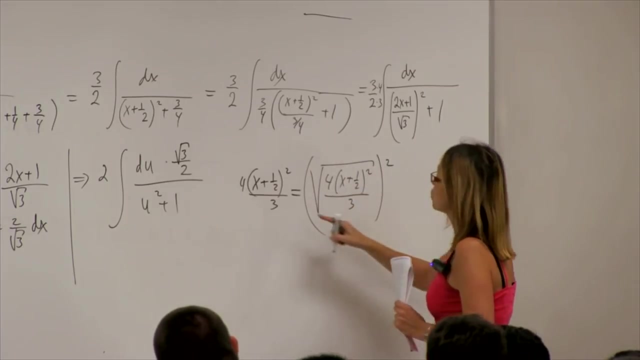 okay, and this is what comes here. why is it still squared? so I, I have um, let me write it out: x plus 1, half squared over 3, 4, equals square root of this squared. so first I take the square root and it's squared, that right. 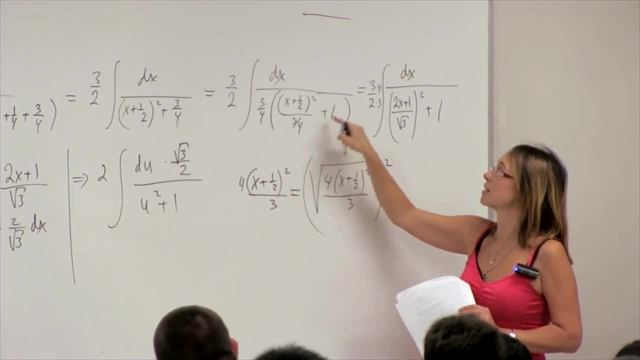 so to figure out, to figure out a way of writing it as a square root of this. I'm going to write it as a square root of this, so a way of writing it as a square of something. I have to take a square root of it. 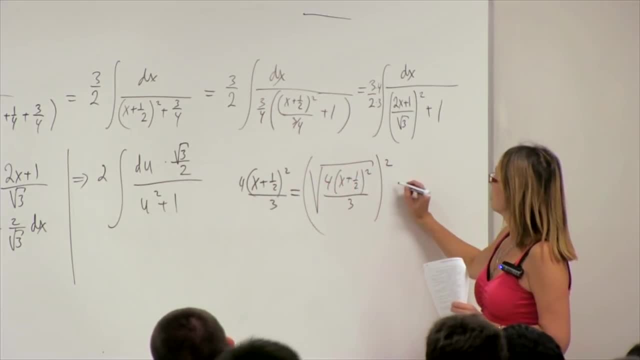 and make a square out of it. so this, this is the operation here. so I'm going to leave the square here and take the square root x plus 1 half, and I have 2 and I have square root 3. this is what I have here. 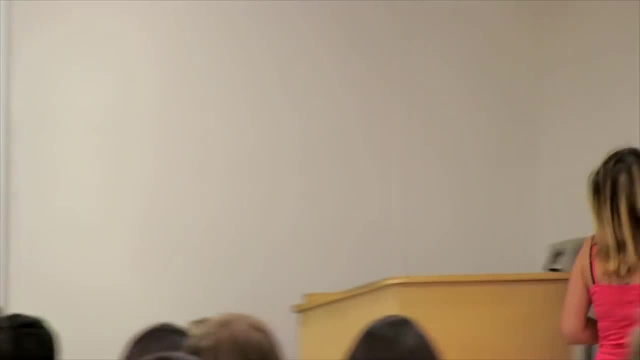 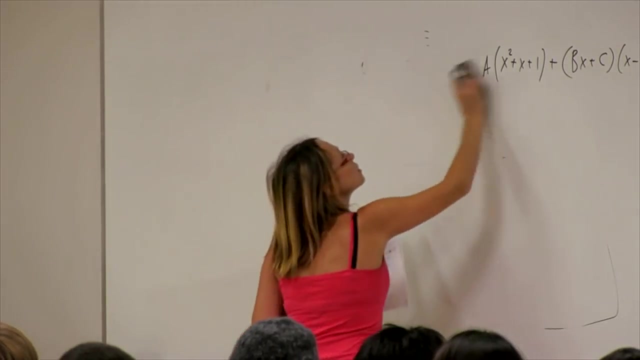 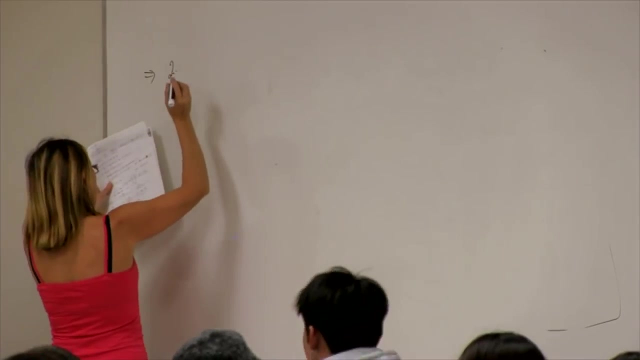 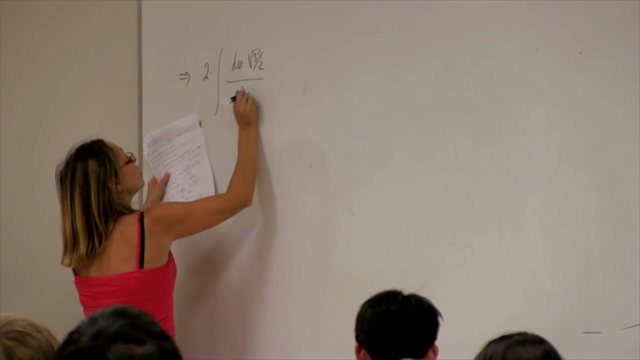 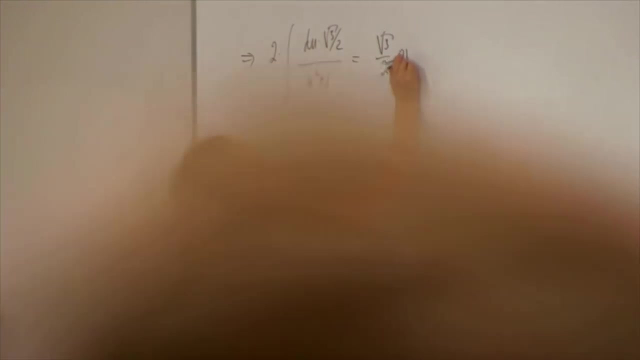 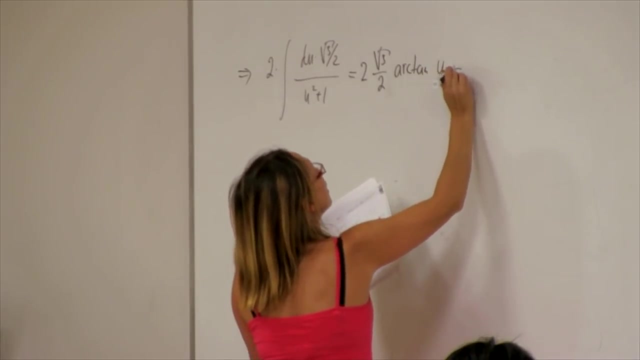 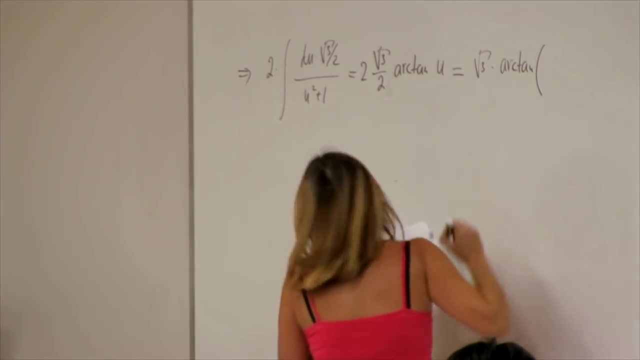 so I'm very close to finishing this. so I have 2 times du squared of 3. what's the antiderivative? this is, of course, squared of 3 over 2 arc tangent of u, and that is squared of 3 times arc tangent of my definition of u. 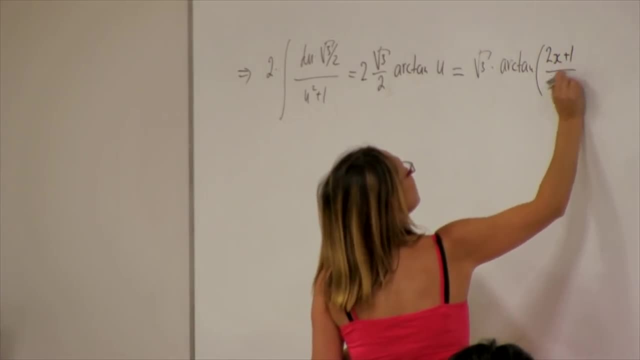 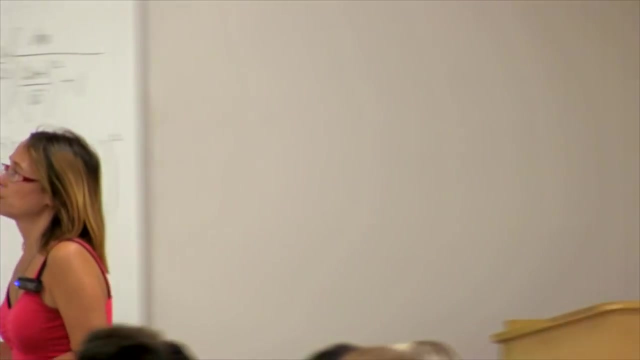 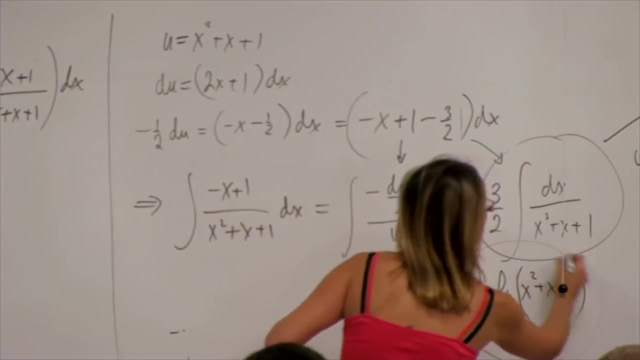 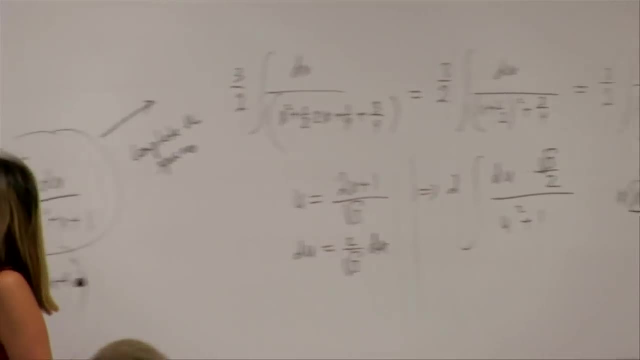 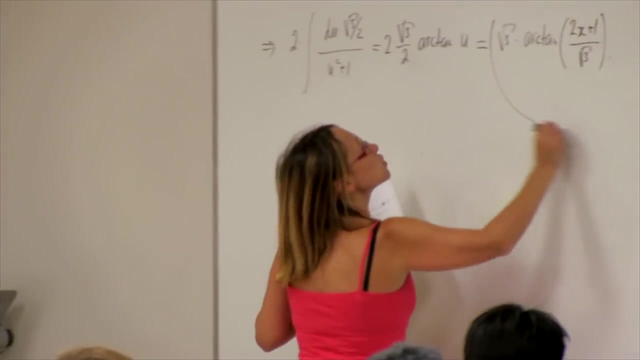 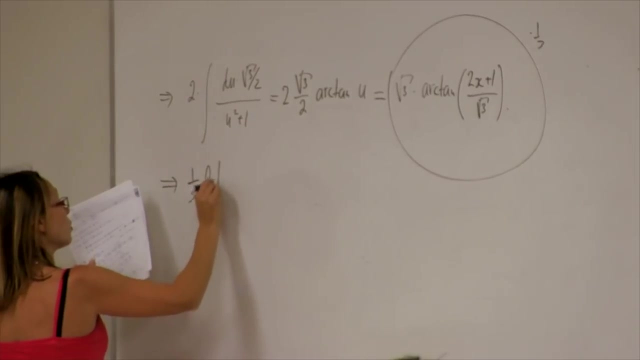 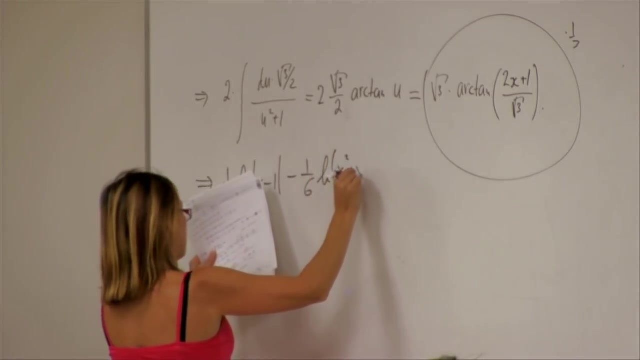 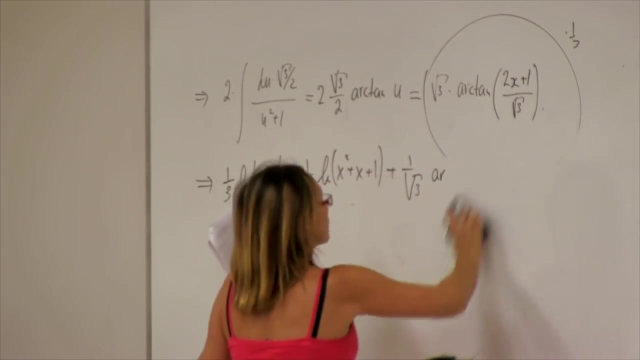 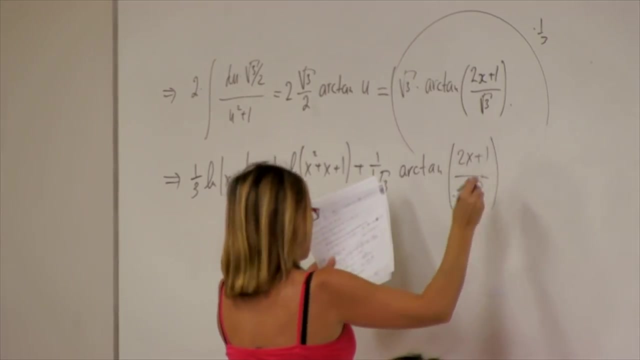 and I have this and I need the factor of 1 third in front. so all together, so this is the third times- 1- 3. so all together I have 1 third log of x minus 1 minus 1 sixth log and the next right hand. 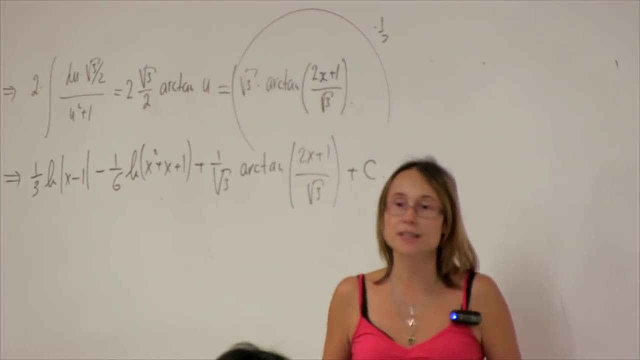 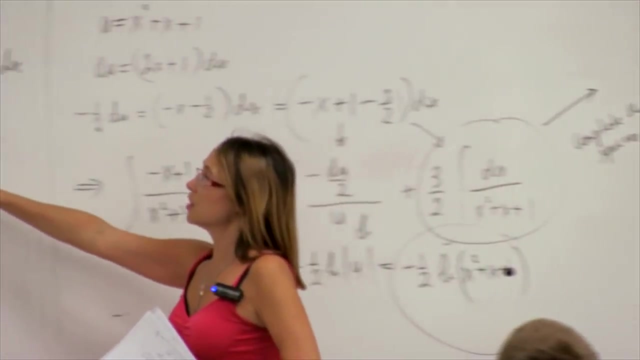 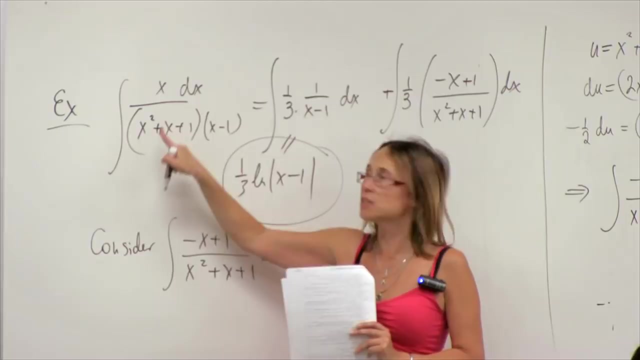 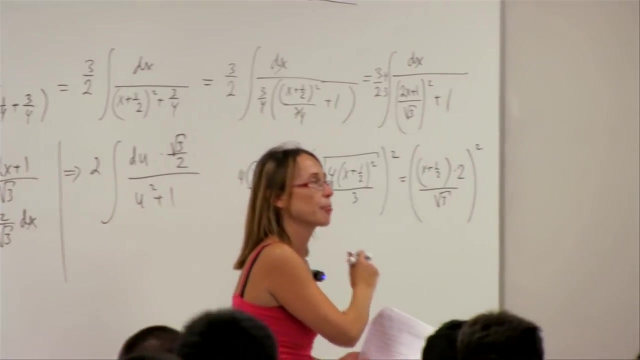 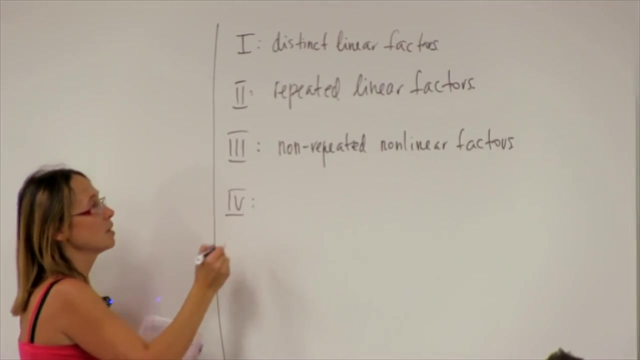 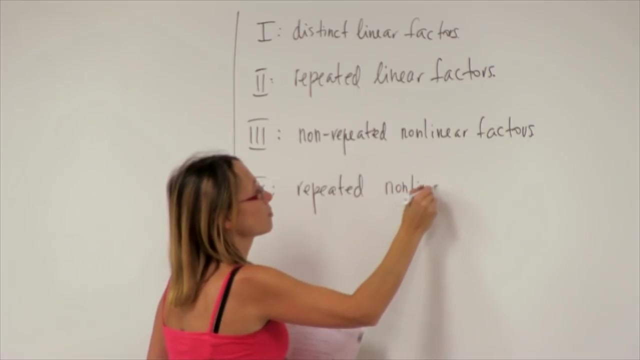 vector in x, and I will. I will define the equation by myself. nice, nice, no, no, nothing, OK, yeah, ok, that's a where in out to be an arctangent, as long as you complete the squares. now to finish, what is the fourth logical case? repeated nonlinear factors? and I will ask the TA.